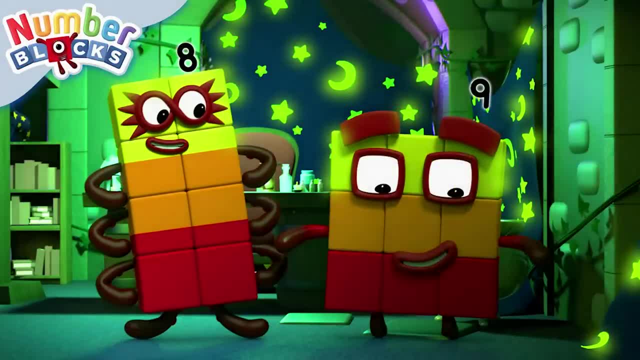 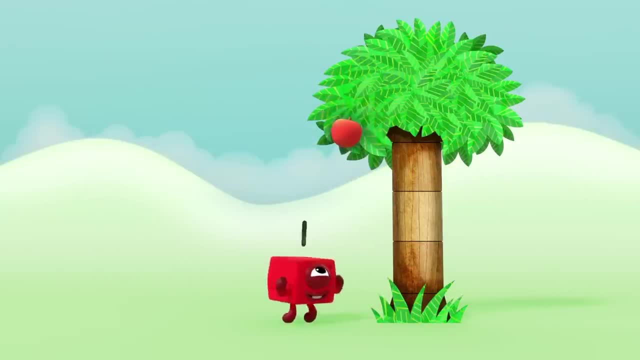 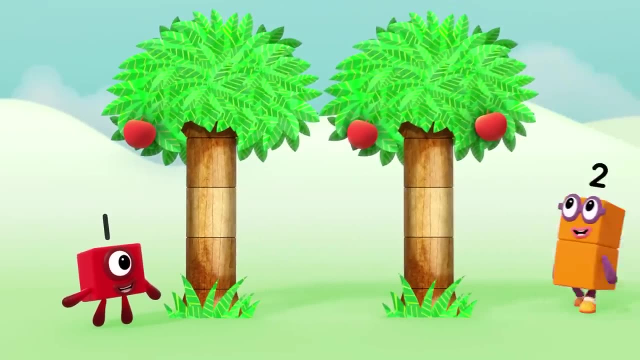 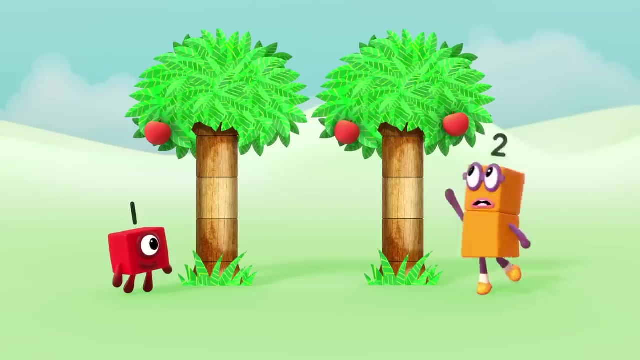 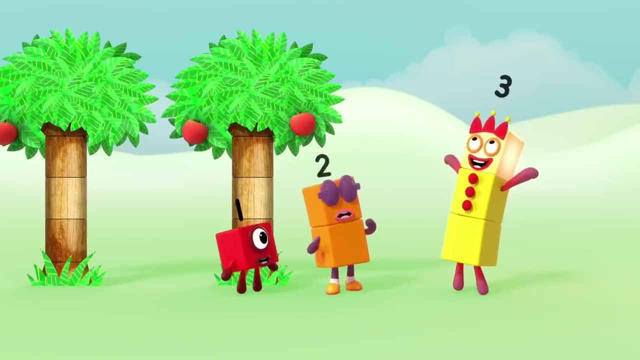 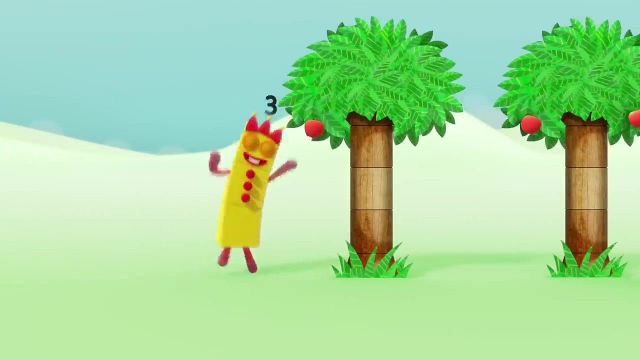 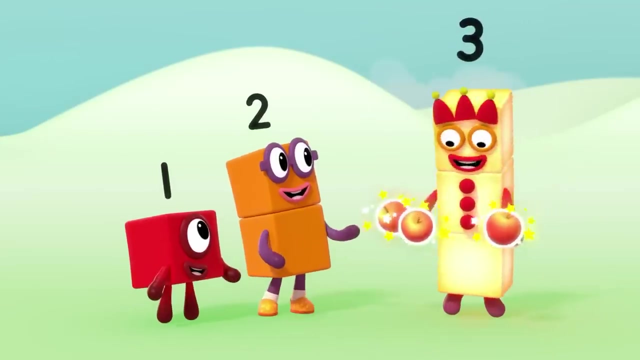 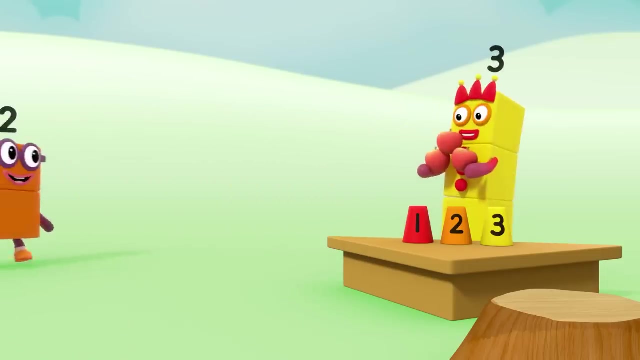 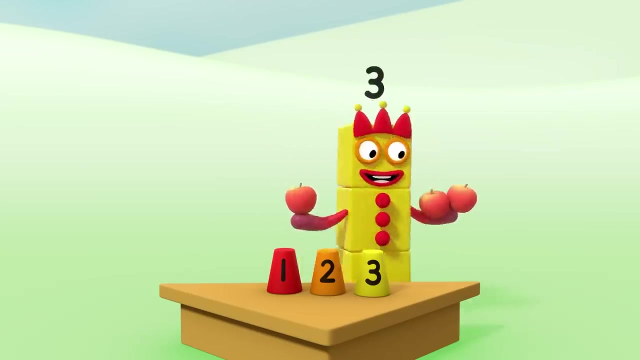 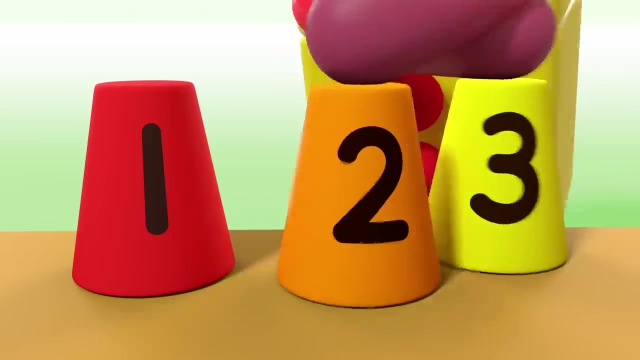 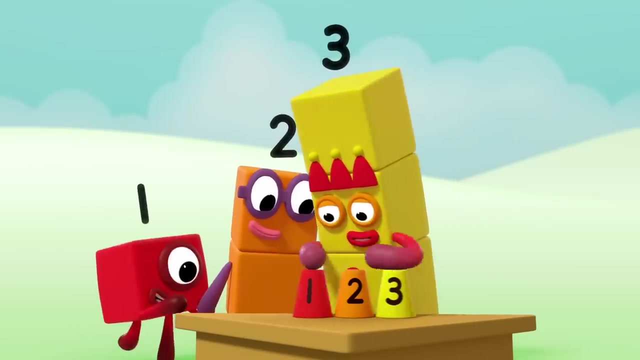 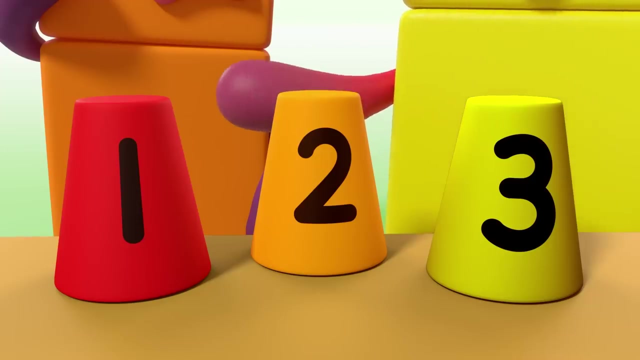 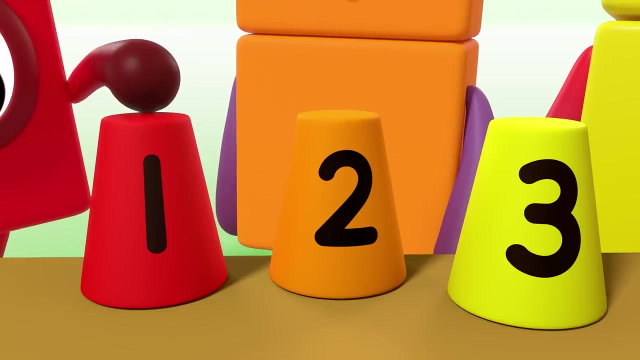 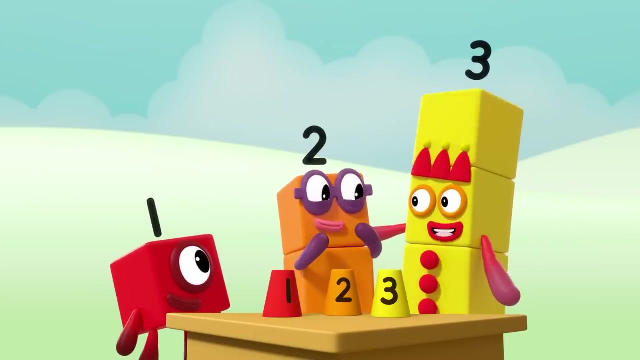 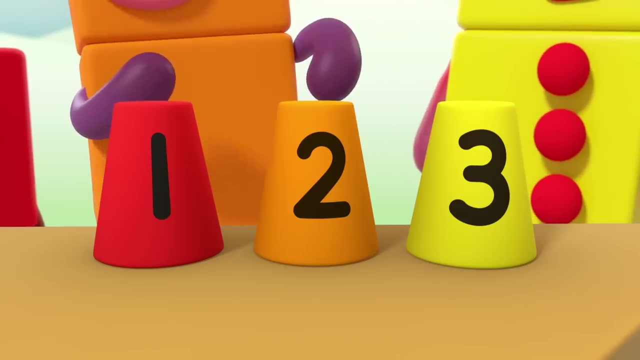 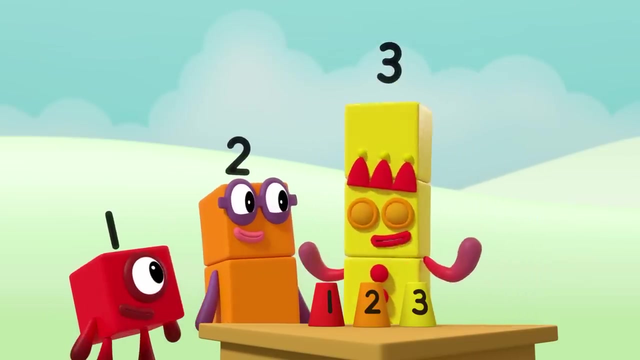 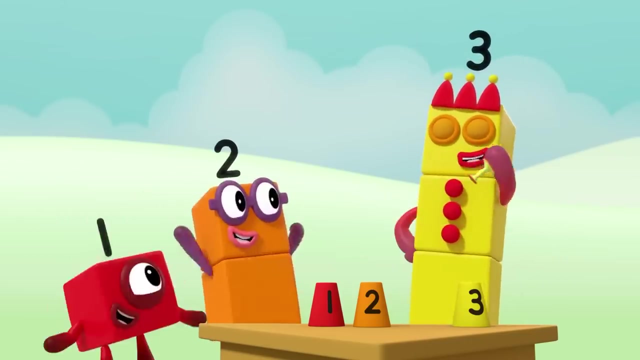 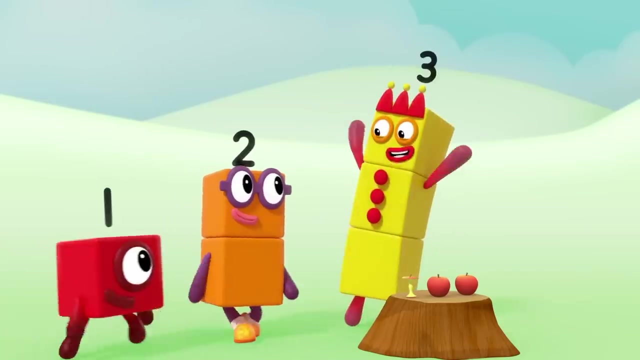 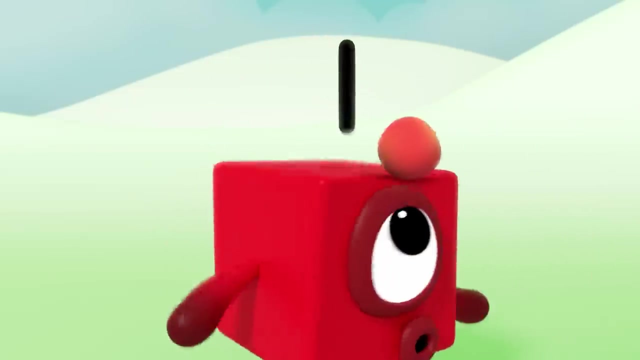 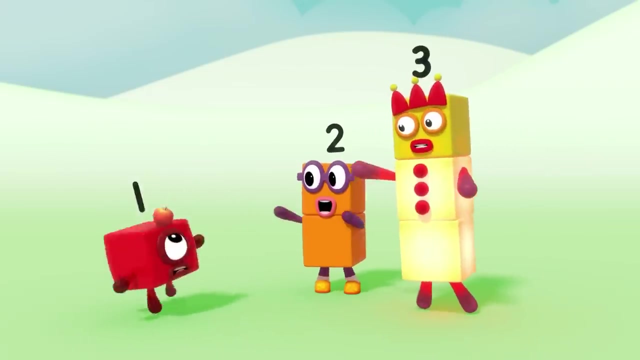 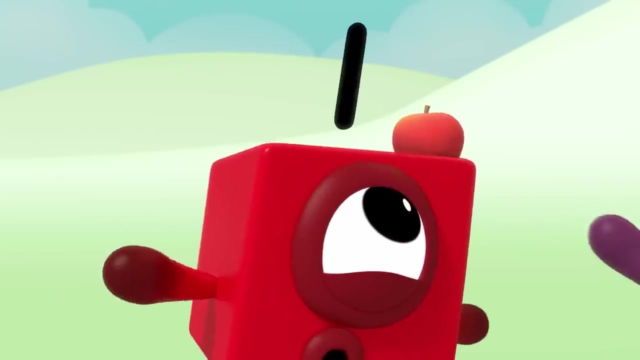 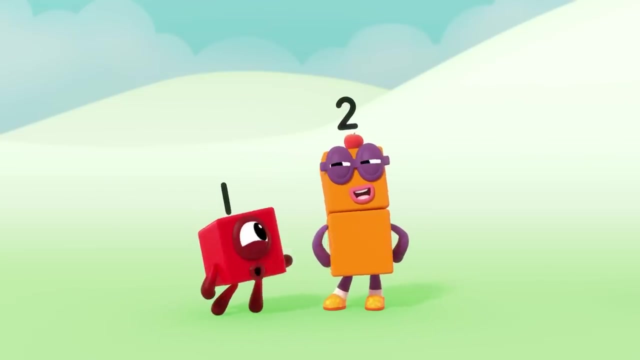 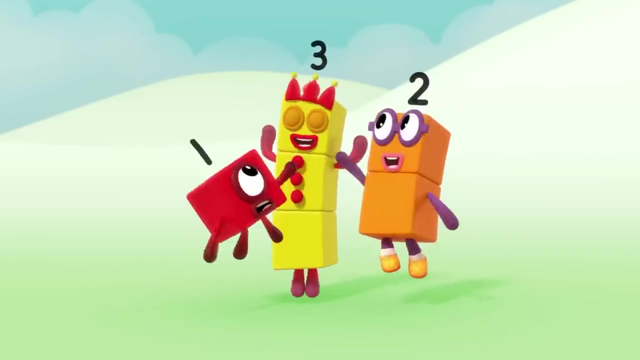 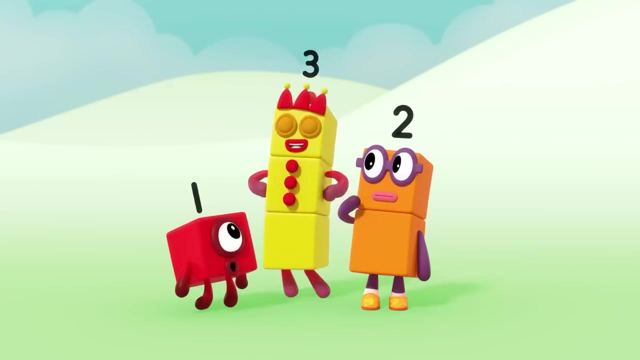 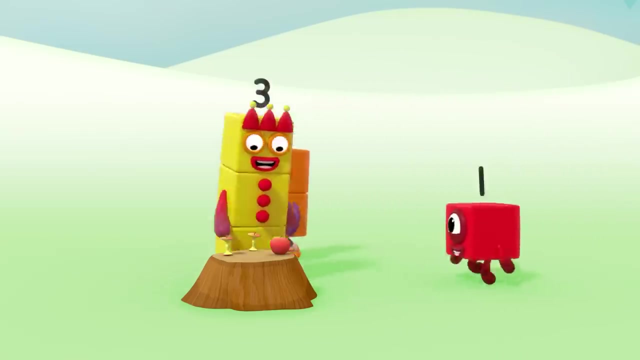 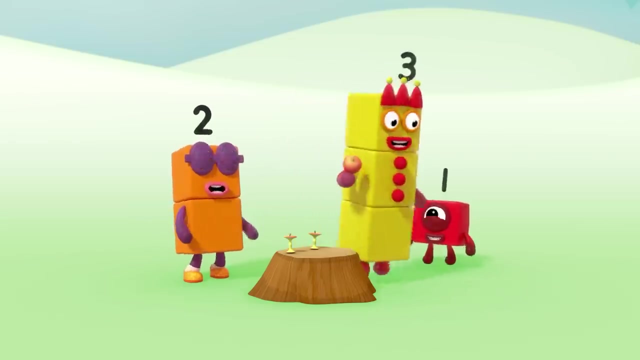 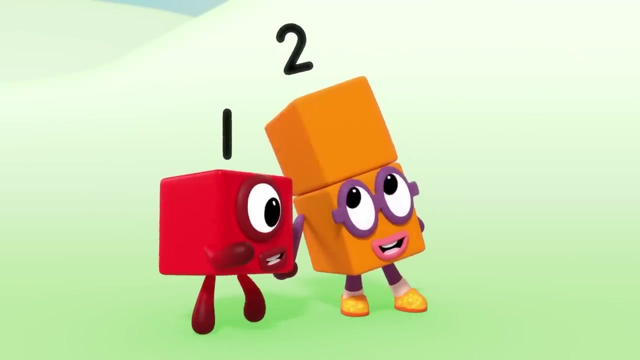 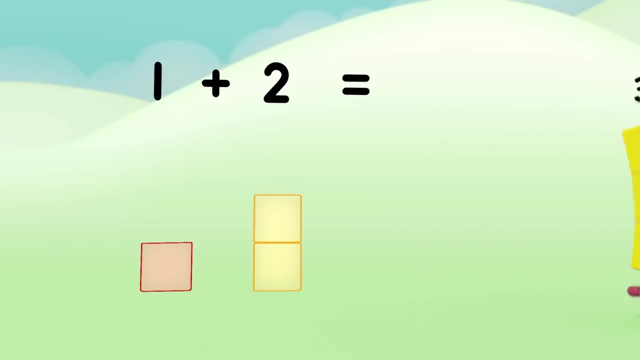 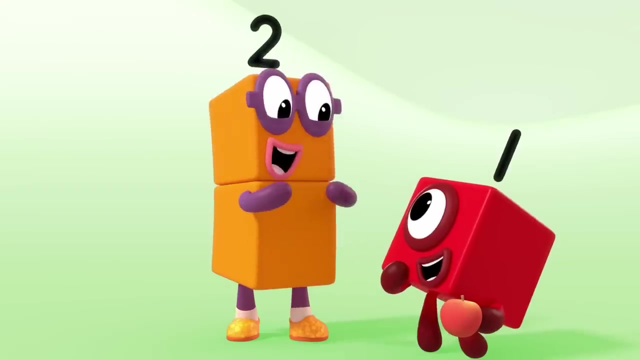 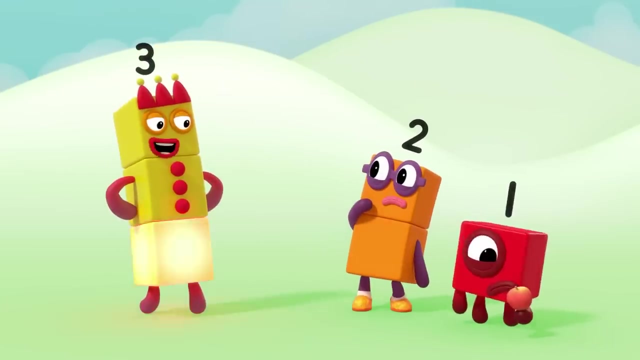 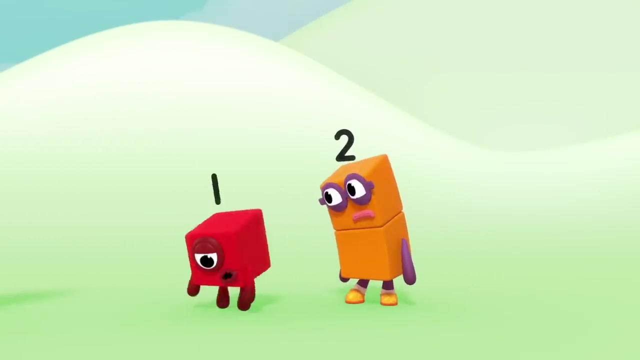 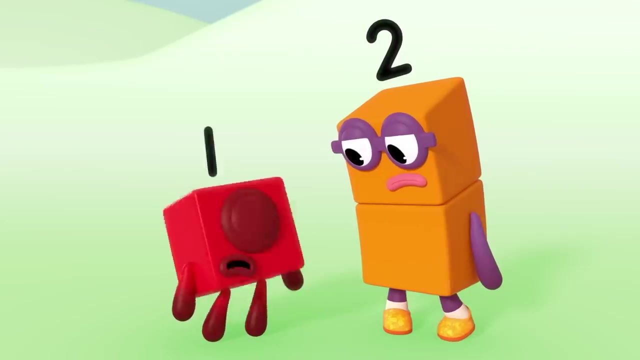 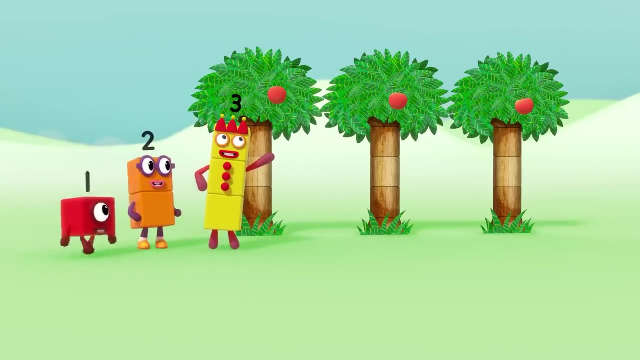 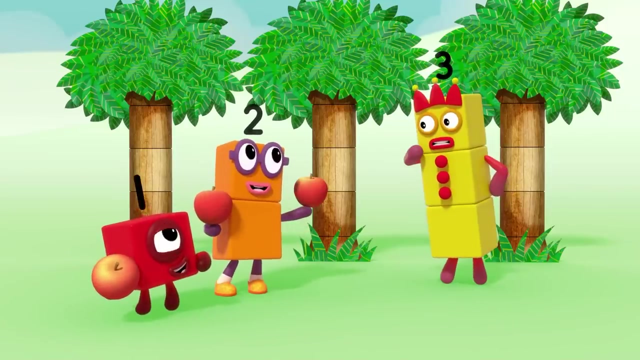 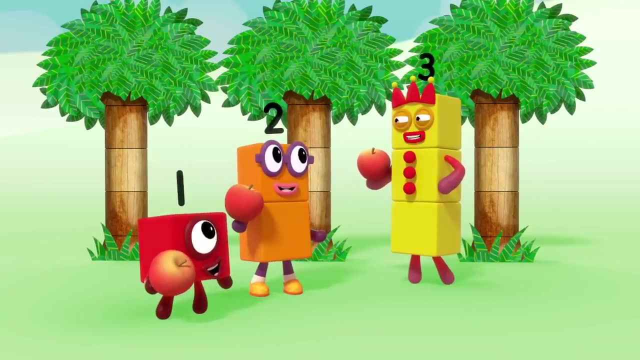 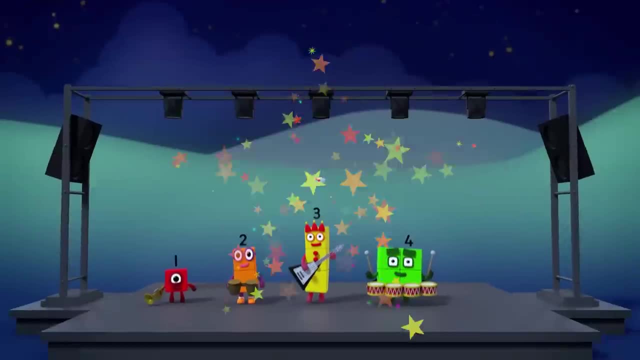 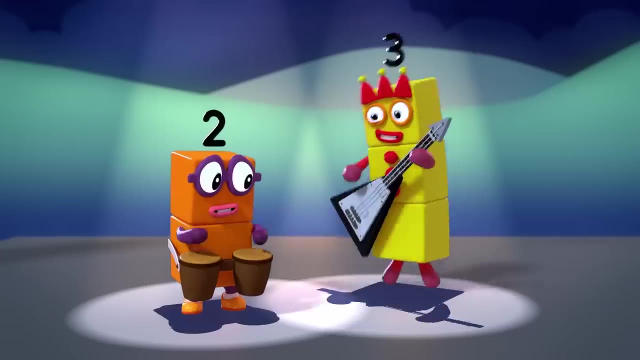 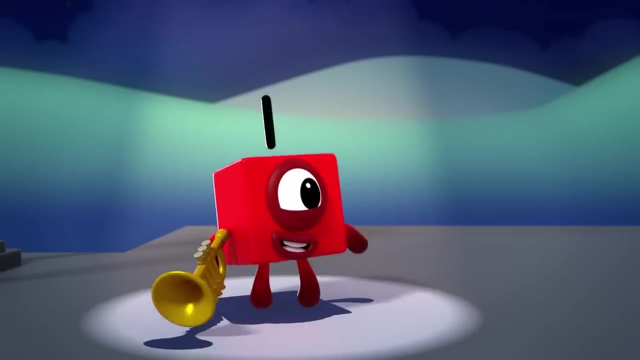 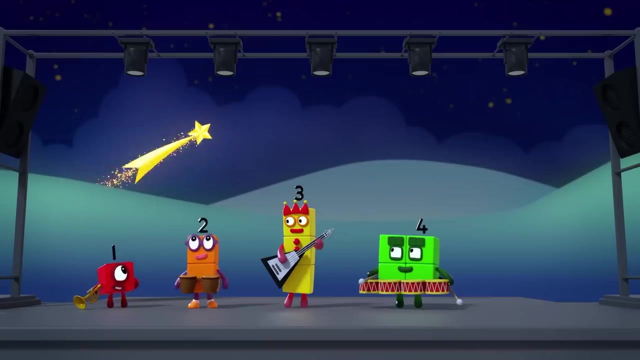 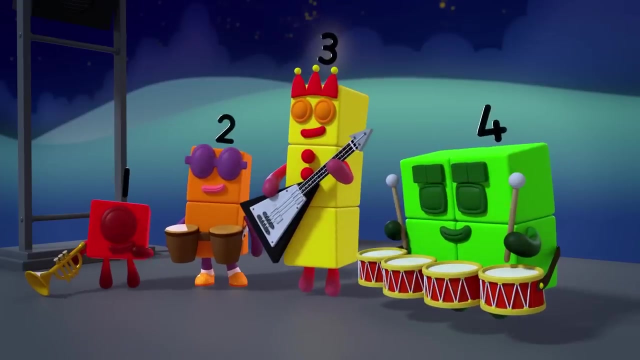 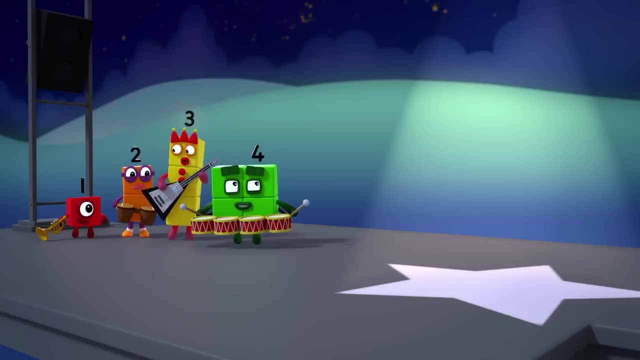 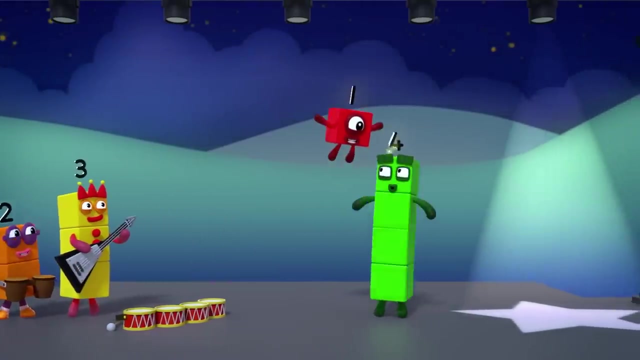 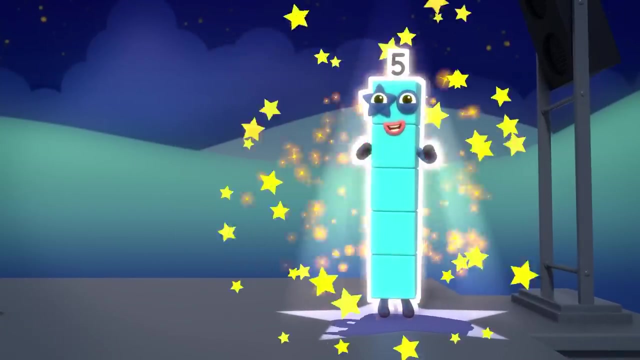 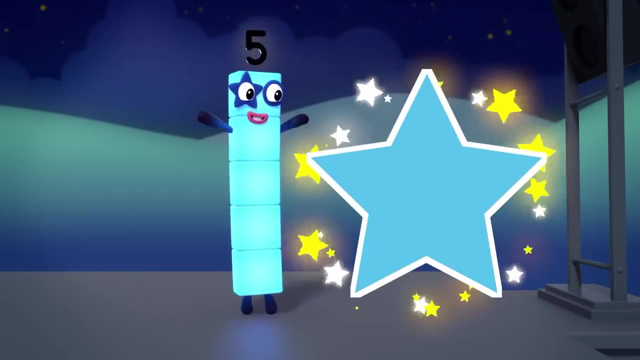 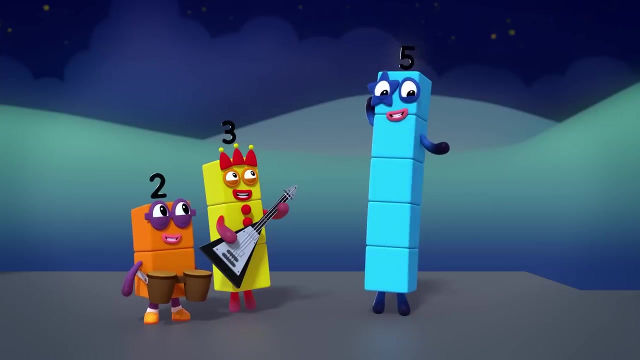 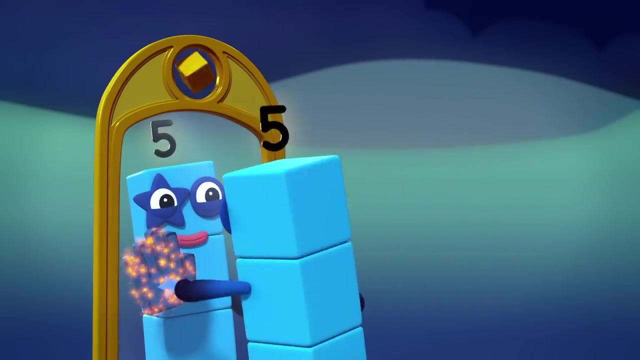 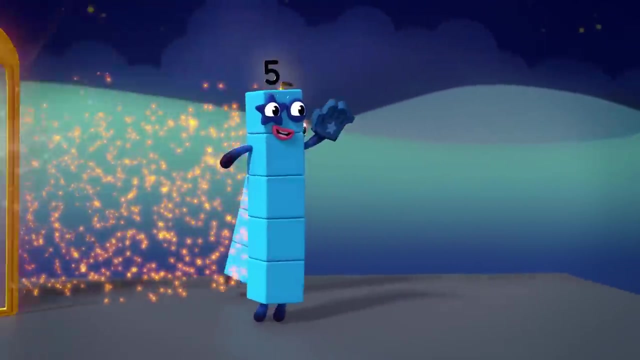 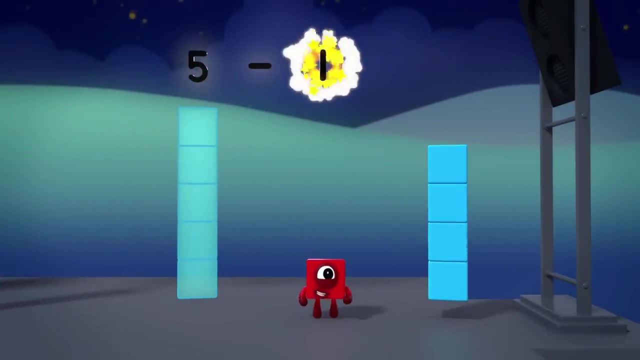 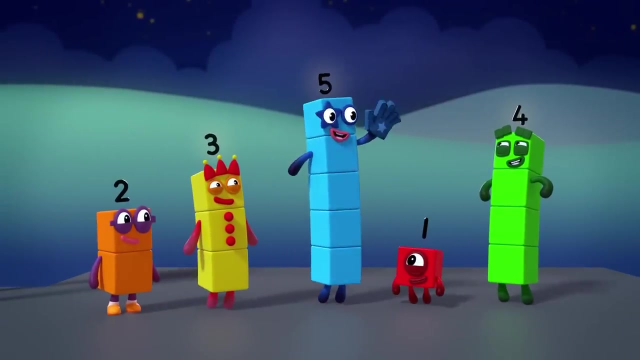 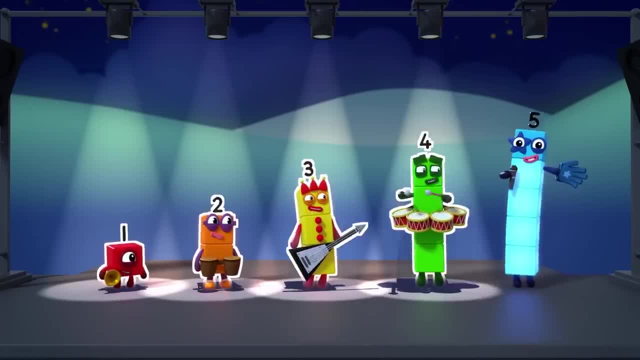 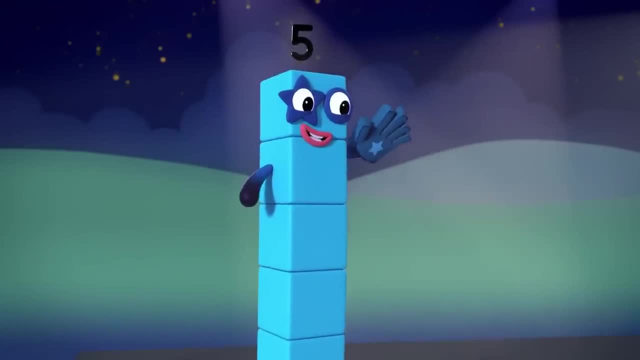 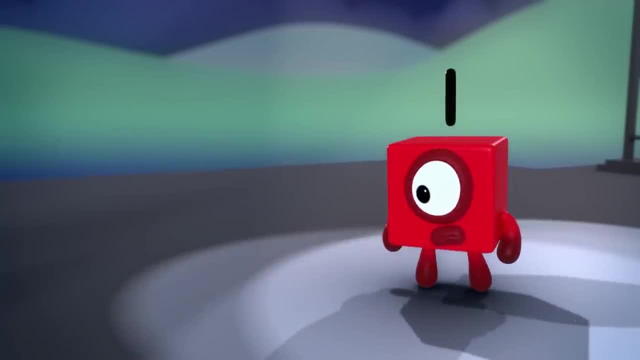 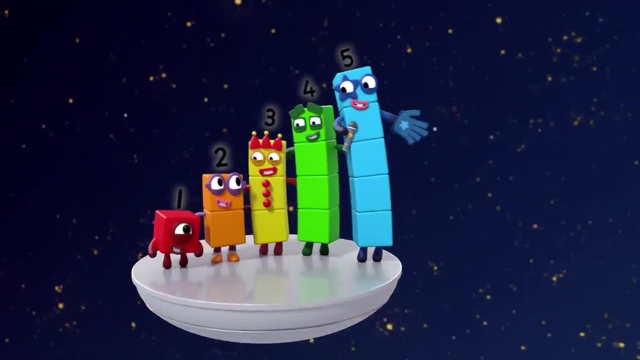 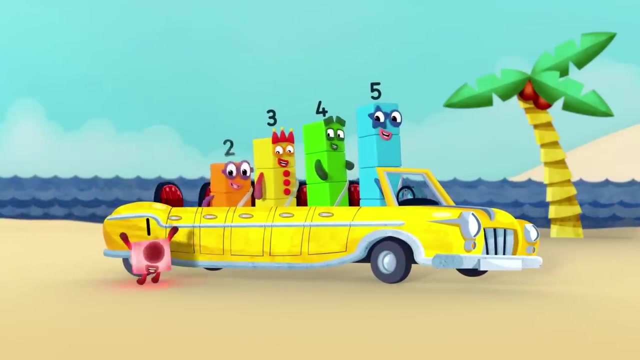 To the side up above, Down, low, too slow, High five, Ooh, I feel so alive. You know that you'll arrive When you're with number five. Five points on a shooting star: One, two, three, four, five, Five seats on my motor car. 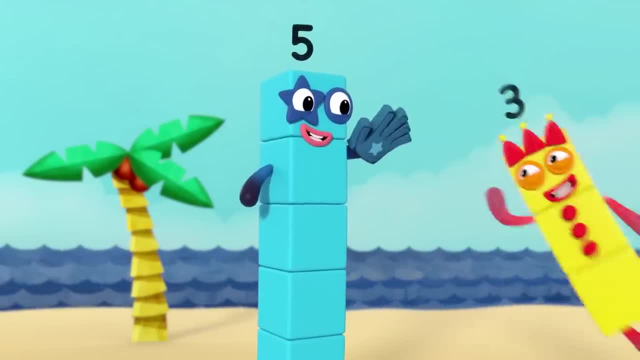 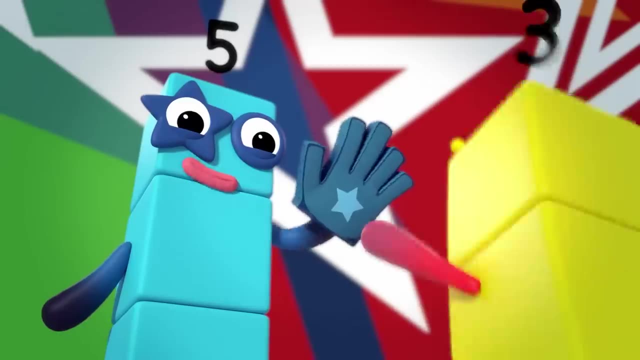 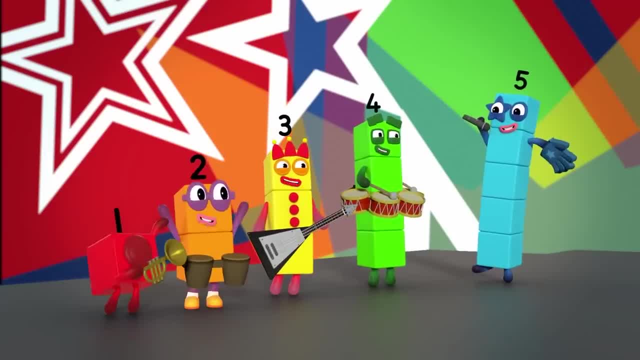 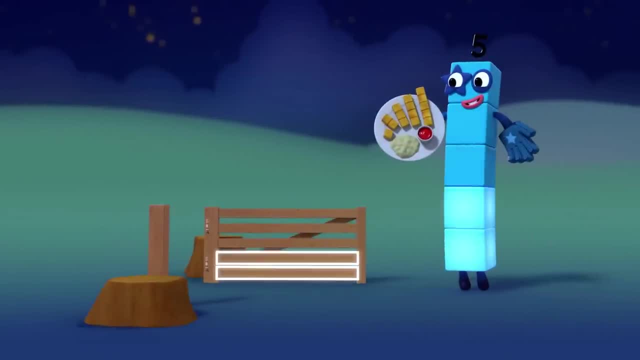 You know that you've arrived When you're with number five. Five fish fingers on a plate: One, two, three, four, five. Five bars on a five-bar gate: One, two, three, four, five. I'm fine. Ooh, I feel so alive. 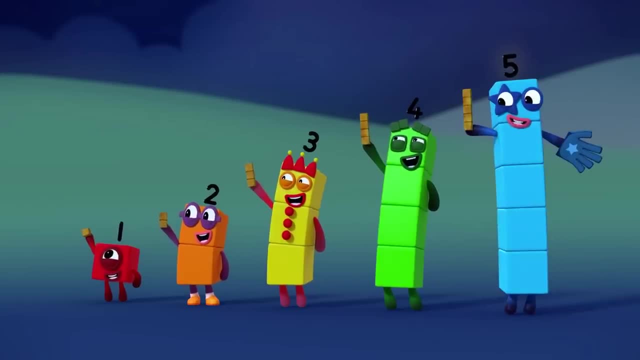 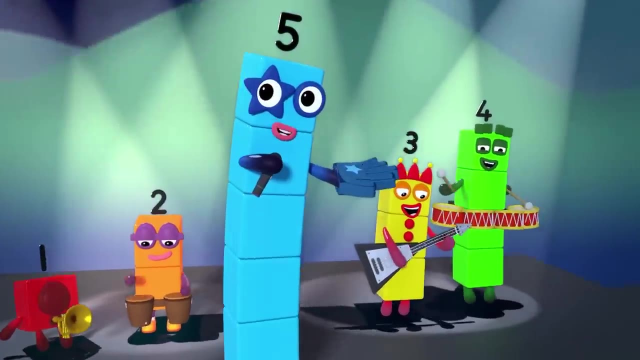 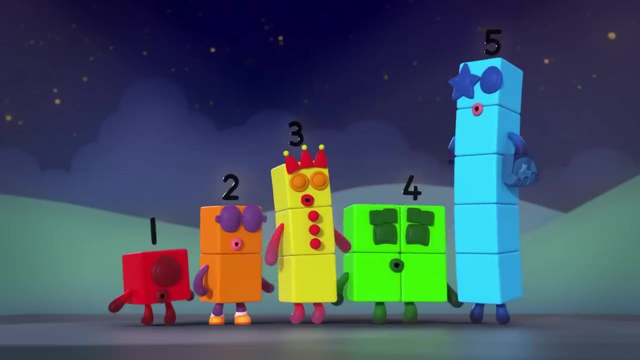 You know that you've arrived When you're with number five. I'm number five And I hope you understand. Whenever you need help, I'll be there for you With battle in the hand. Now the band is all together. The rest can join the queue. We'll be five stars forever. 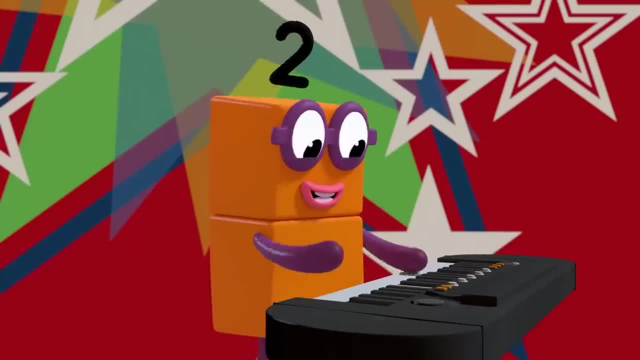 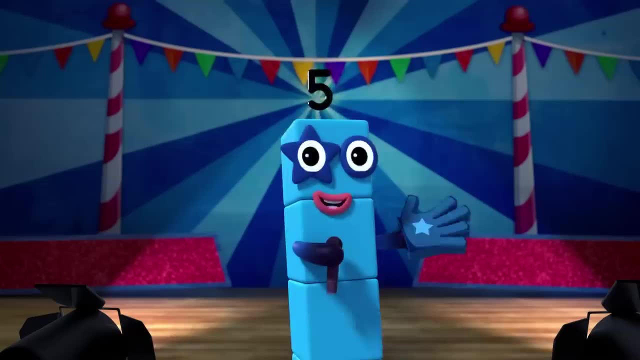 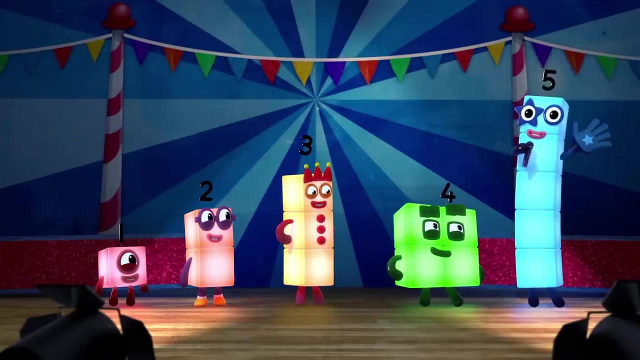 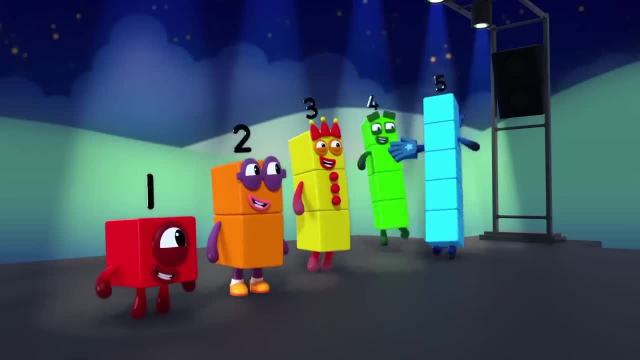 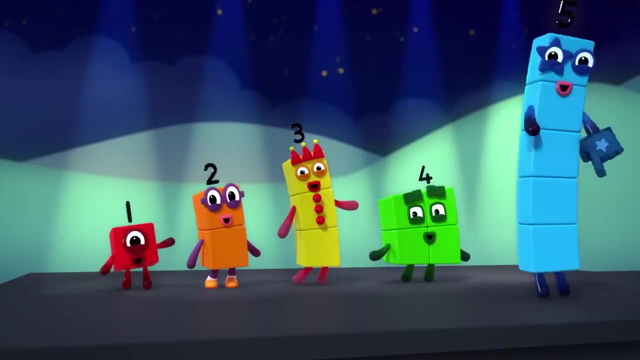 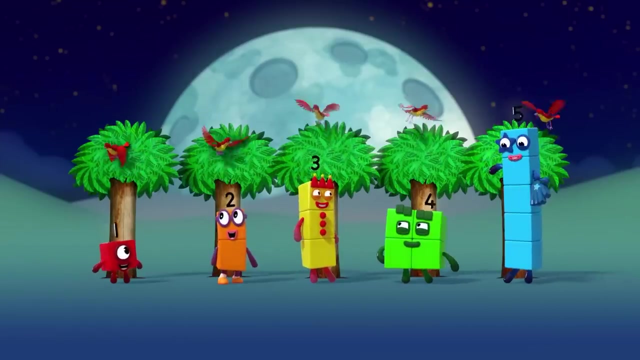 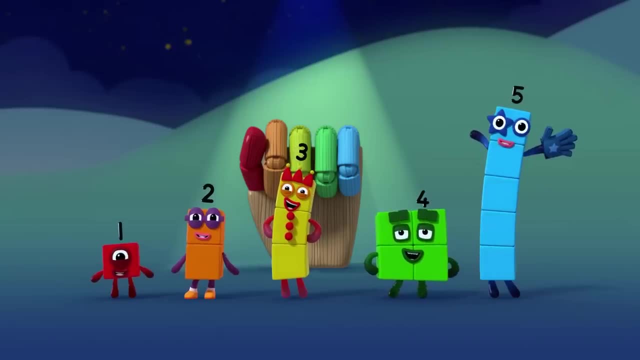 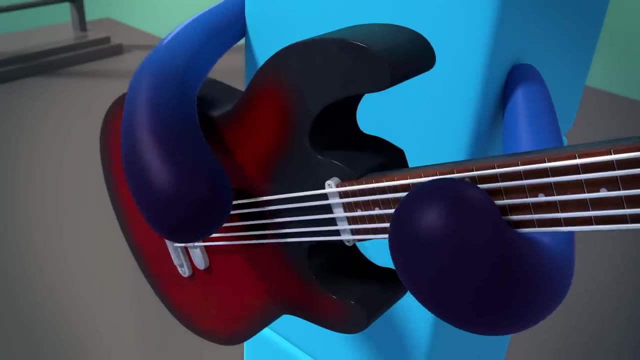 One, two, three, four, five. Everybody do the big hand dive. One, two, three, four, five. One, two, three, four, five. One, two, three, four, five, Five strings on a five string bass: One, two, three, four, five. 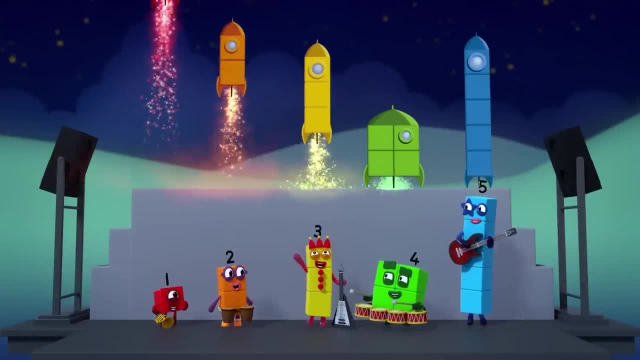 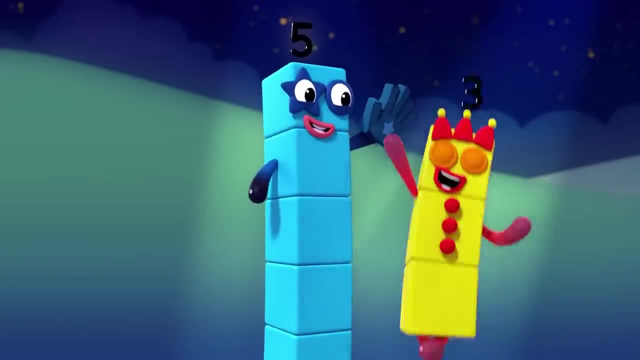 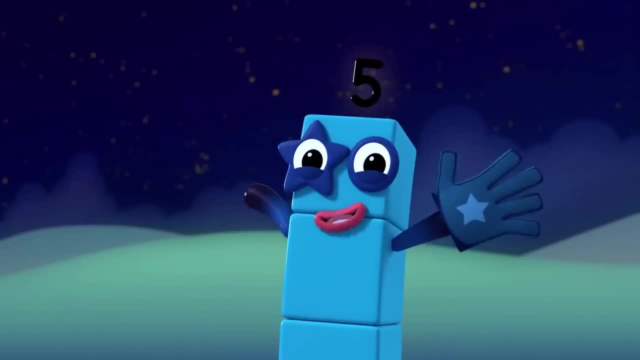 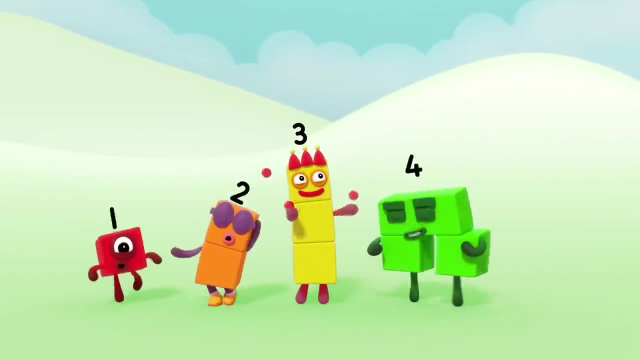 High five, High five. Oh, I feel so alive. You know that you've arrived. You got the big one. You looking split. Who is that? When you're with number five? One, two, one, two, three, I can do my exercises, Hi, team. 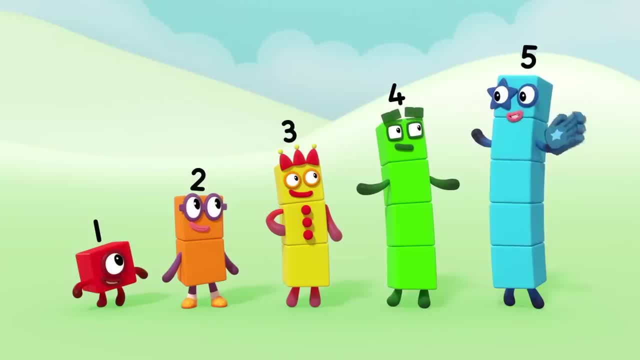 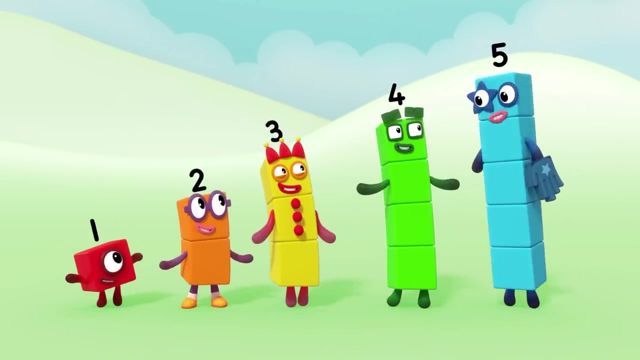 Hi-fi. So are we all here? Um Well, how can we tell? I know just the thing: Ready, steady, sing One, two, three, four, five. That sounds right. What shall we do today? Walk in the sunshine, Run through the forest. 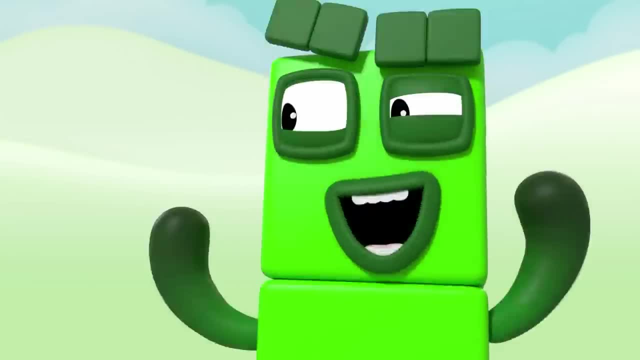 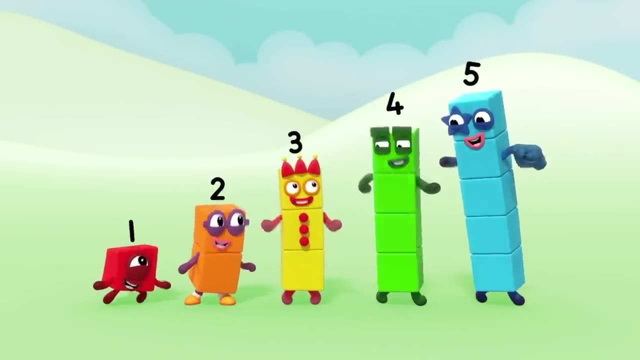 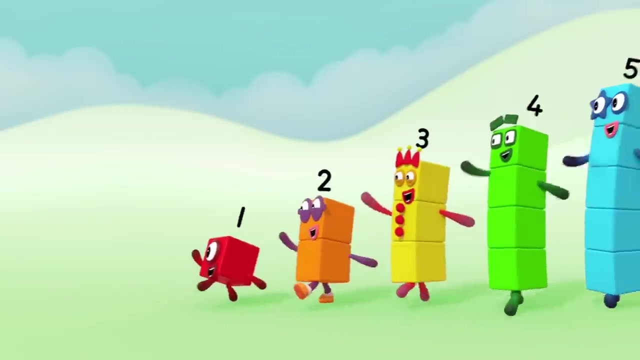 Climb to the top of a tree, Pretend to be pirates, Discover a whole new world. Let's have an adventure. Hooray, Everybody ready. Off we go Off. we go On a big adventure. We don't know what the day will bring. Off we go. 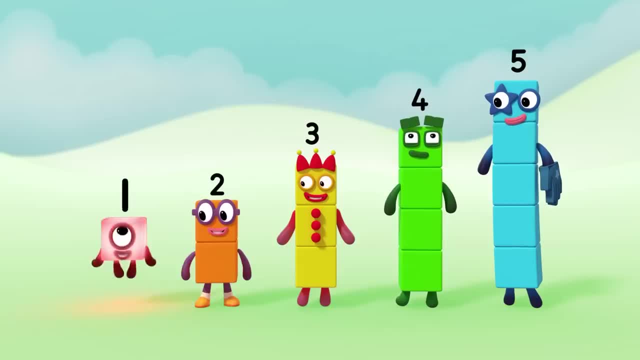 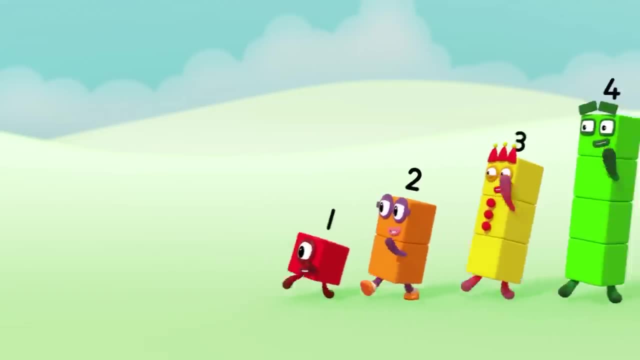 On a big adventure. Ready, steady sing. One, two, three, four, five- That sounds right. And off we go again. Off we go On a big adventure. We don't know what the day will bring. Off we go, Walking in the sunshine. Ready, steady, sing. 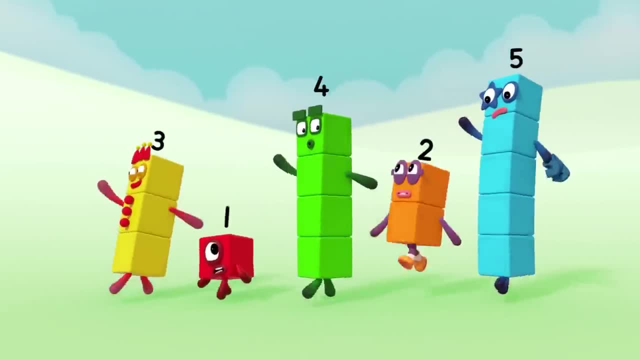 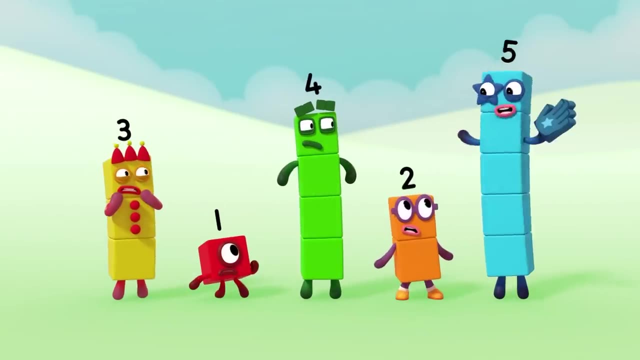 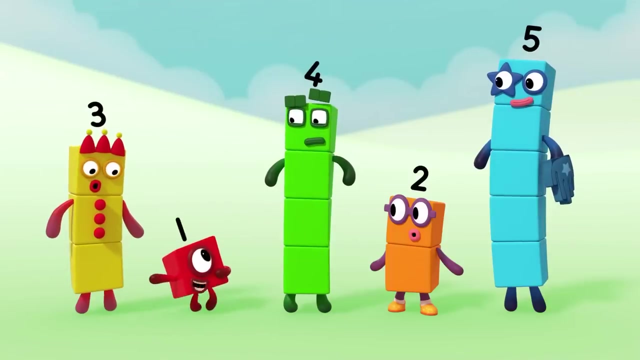 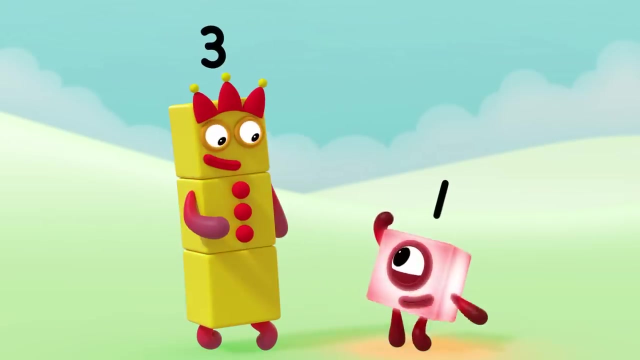 Wait Too short, Can't see Three, one, four, five. That doesn't sound right. We're in the wrong order. I know what to do. Diddly, diddly do. Smallest that way, Biggest this way Go. I'm bigger than you. I'm smaller than you. 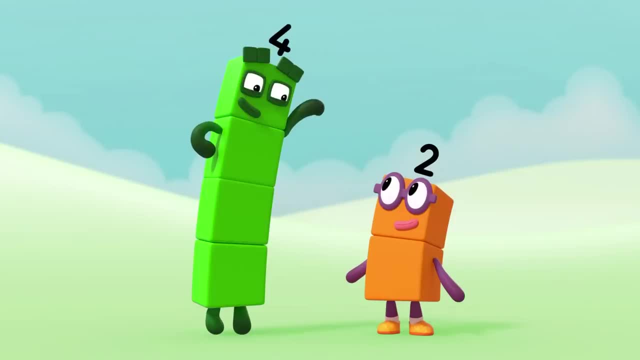 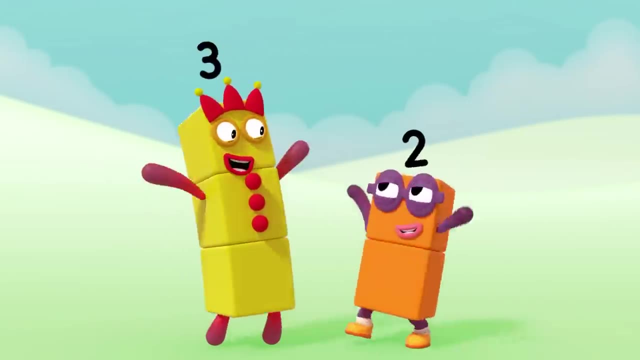 Diddly diddly do. I'm bigger than you. I'm smaller than you Diddly diddly do. I'm bigger than you. I'm smaller than you Diddly diddly do. Are we all in order? Did we all do the right thing? 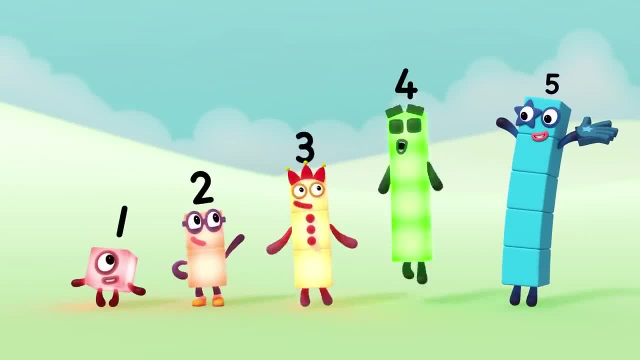 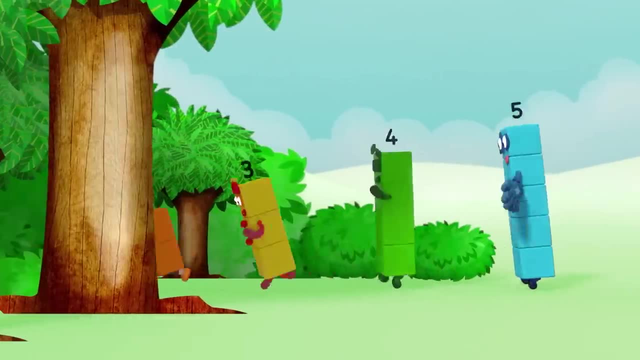 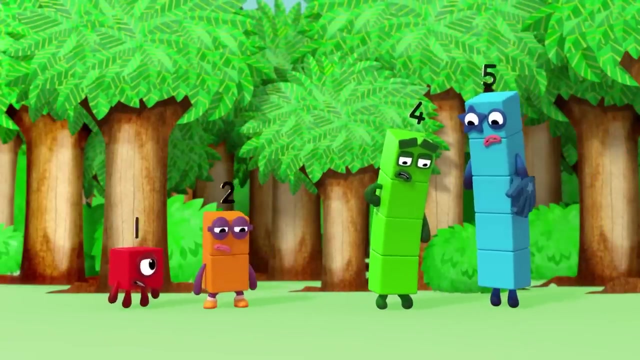 Ready, steady, sing One, two, three, four, five. That sounds right. And off we go again. Off we go On a big adventure, We don't know what the day will bring. Off we go Running through the forest. Ready, steady, sing One, two, four, five. 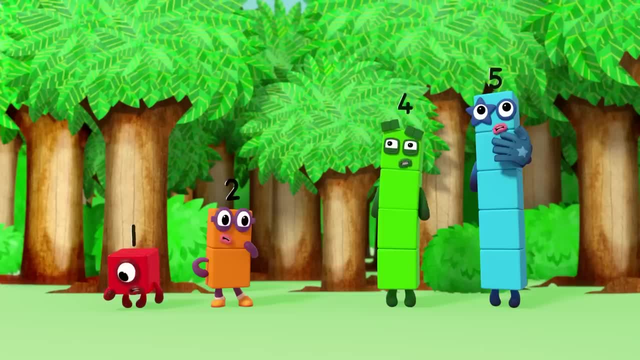 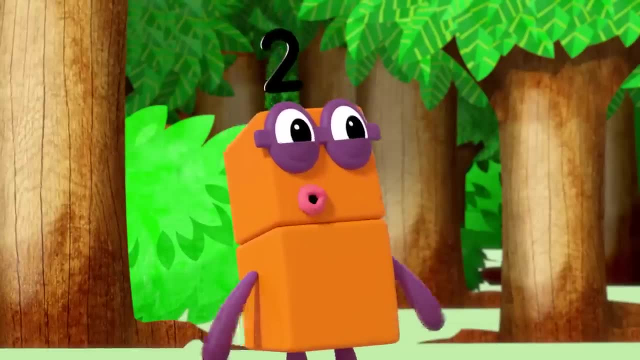 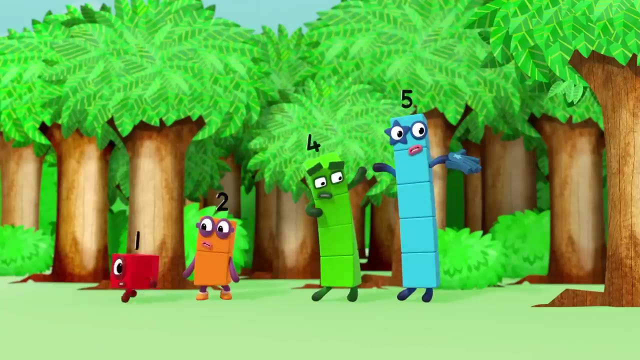 That doesn't sound right. Someone's missing. Who can it be? Let's see. I'm one. Start with me. I'm two, I come after one. I'm four, I come after three, Three, Three's missing. Where is three, Three, Look at me. I'm number three. 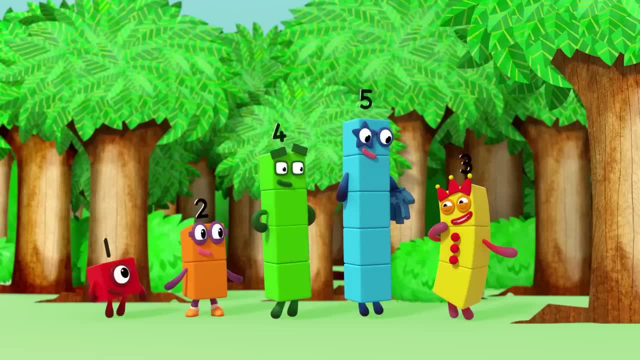 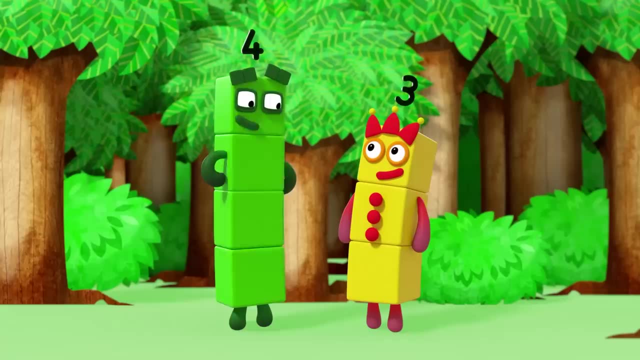 Three, I know what to do. Diddly diddly do? I'm bigger than you? I'm smaller than you. Diddly diddly do I'm bigger than you? I'm smaller than you. Diddly diddly do? I'm smaller than you. 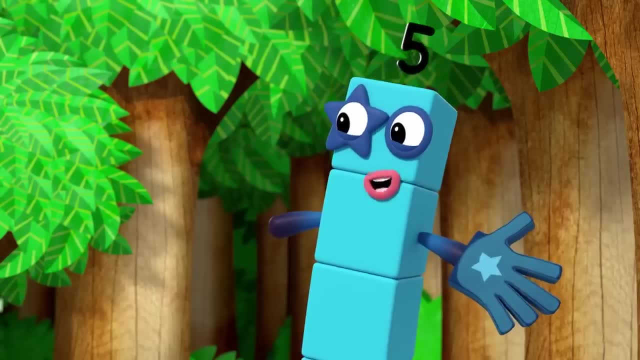 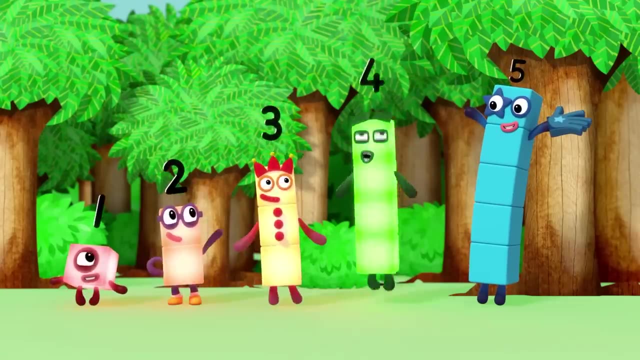 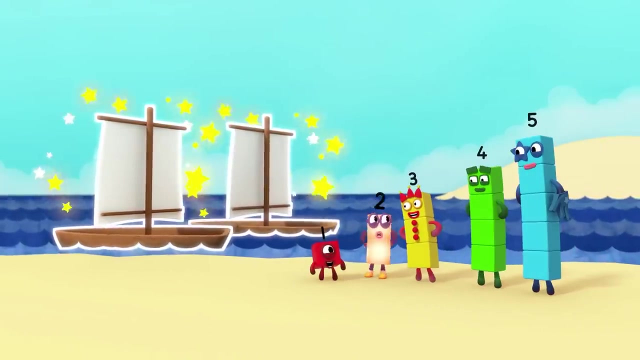 Stop. Are we all here now? Did we all do the right thing? Ready, steady, sing One, two, three, four, five. That sounds right. And off we go again. Look One, two, two sailing boats. We can be pirates. 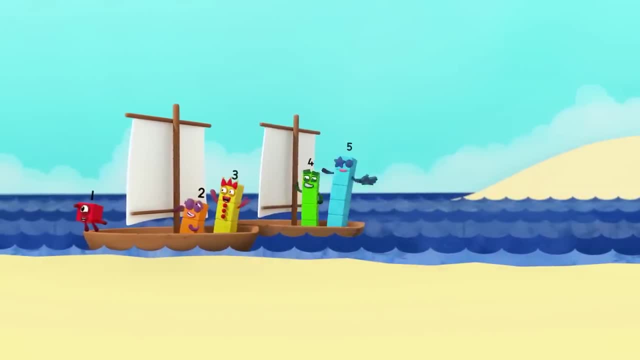 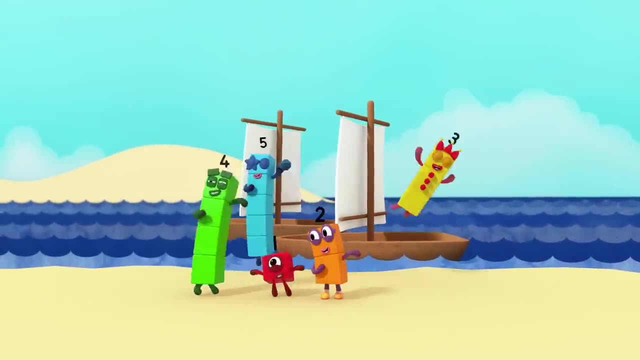 Ha, ha, ha, ha, Off we go On a big adventure. We don't know what the day will bring. Off we go Sitting on the ocean, Ready, steady, sing Four, five, one, two, three. That doesn't sound right. We're in the wrong hole. 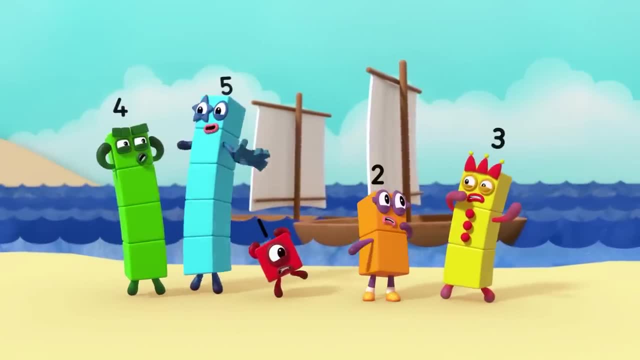 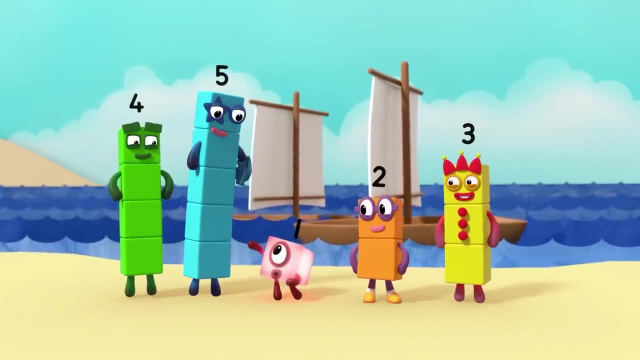 See Four, five, one, two, three. That sounds right. We're in the wrong hole. We're in the wrong hole. We know what to do. diddly-diddly-doo, I'm bigger than you. I'm smaller than you. 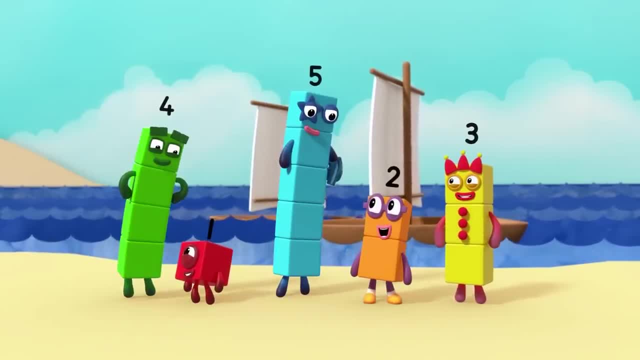 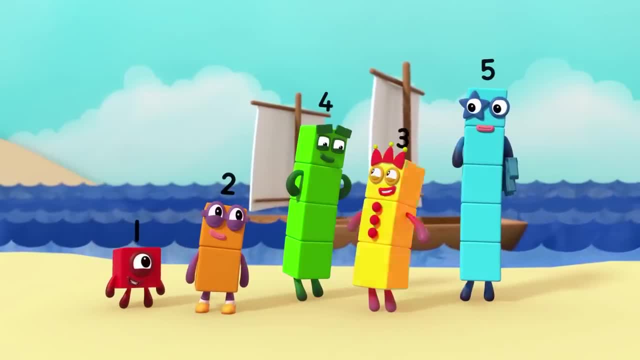 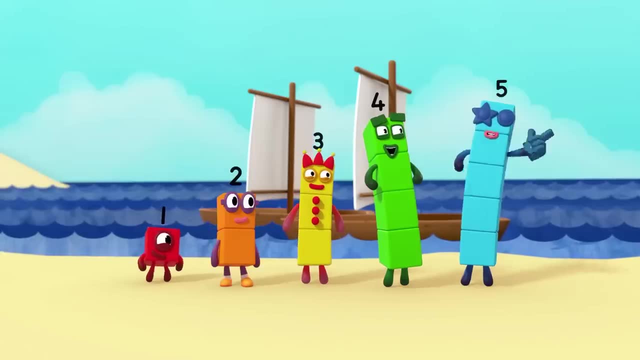 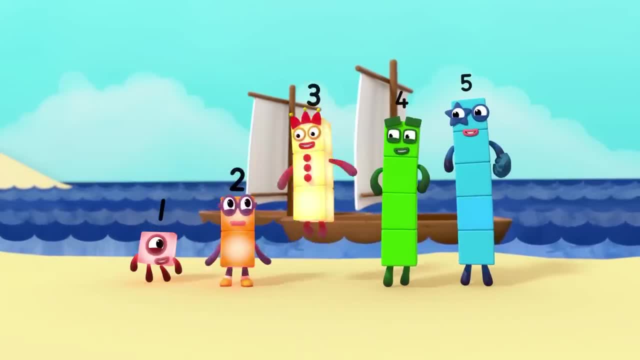 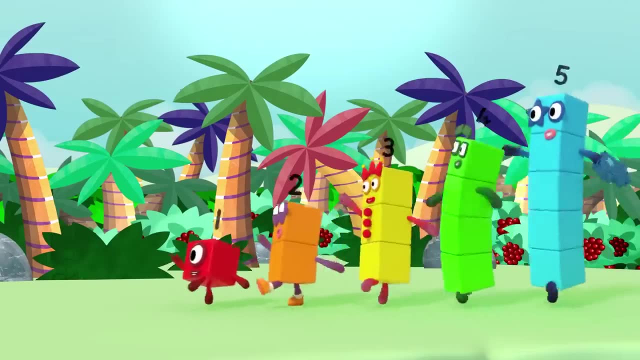 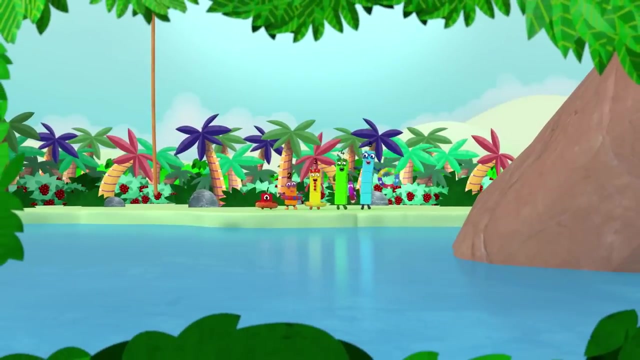 Ready, steady, sing One, two, three, four, five. That sounds right. And off we go again. Off we go On a big adventure. We don't know what the day will bring. Here we are Discovering a new world. 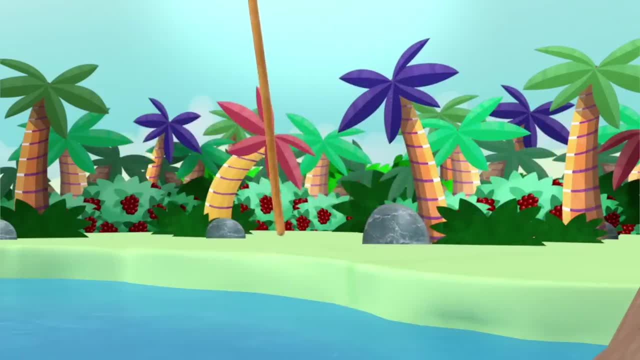 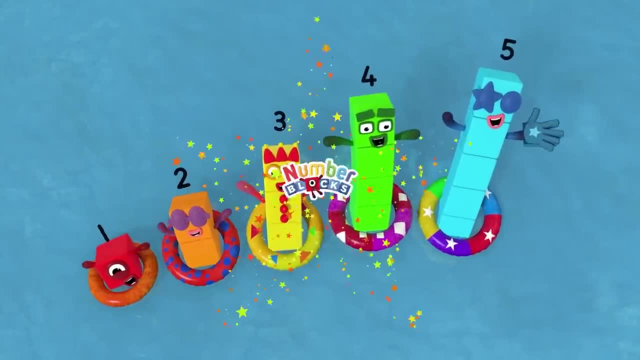 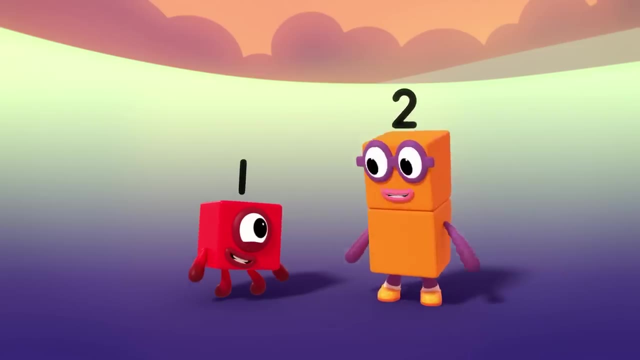 Ready, steady, sing One, two, three, four, five. There we go. One, two, One, two And again One two. Your turn One. I can't do it Right. What was that? 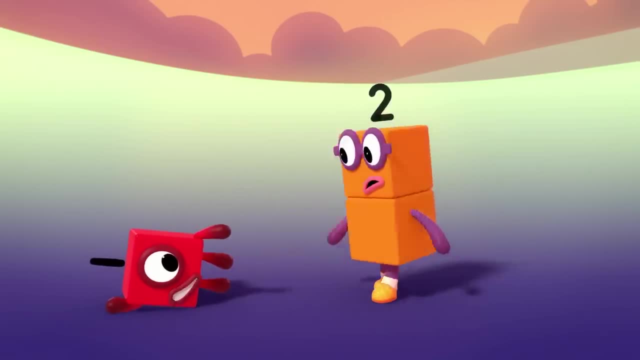 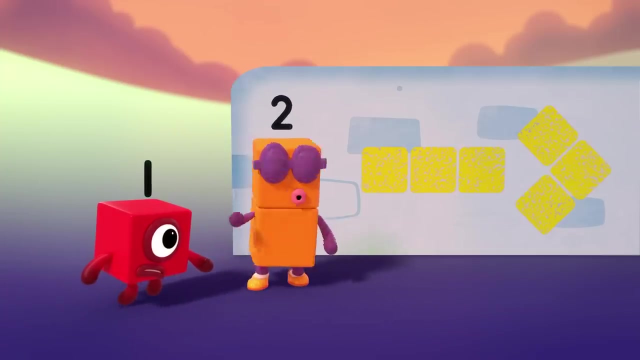 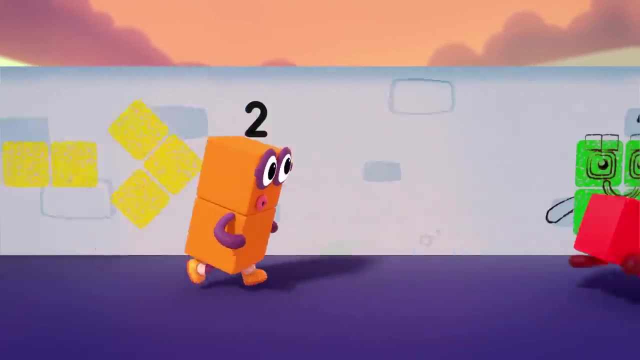 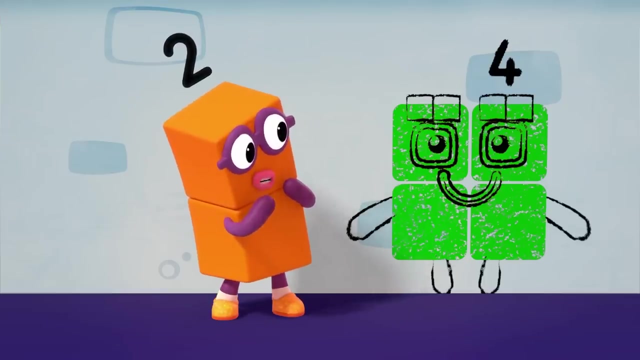 That way. come on, Wait, Looks familiar. Boing, boing, boing, Boing, boing, boing. It's pointing to the sounds. Quick, Hey, It's four, Four, Four. Are we playing musical statues? A painting, A painting of four. 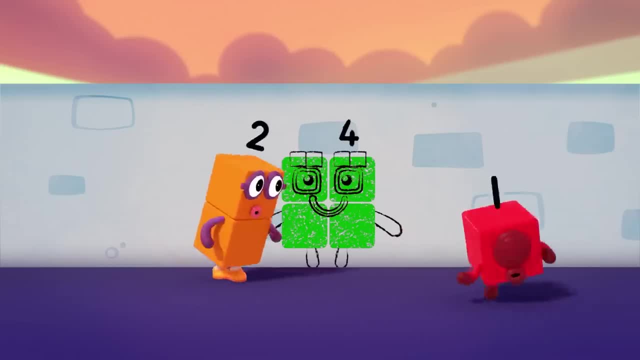 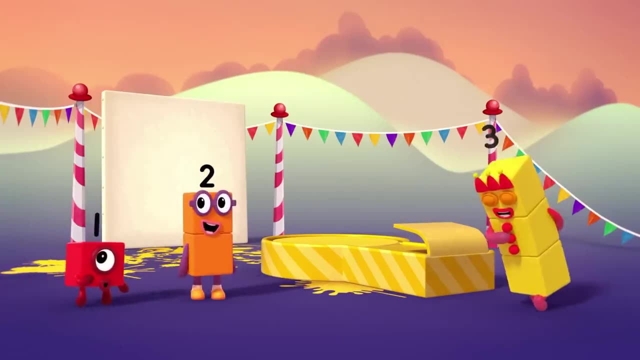 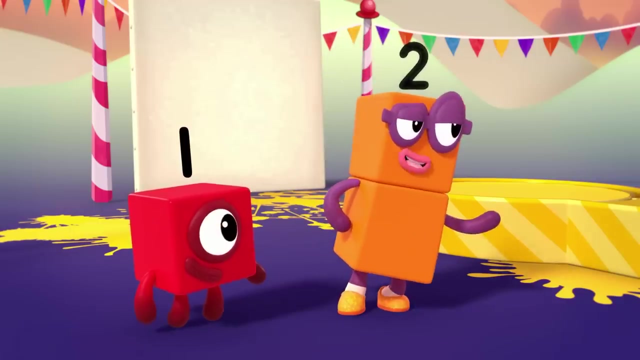 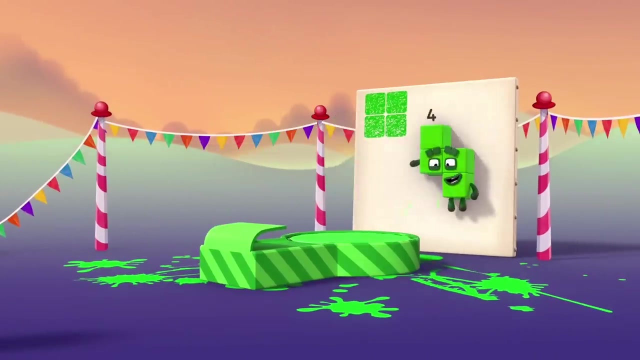 I knew that. But what's that? Welcome, welcome, welcome to my new Stampoline Park. Don't you mean trampoline? No, no, no, Look, Whee, Ooh, that was fun. Four, Is that you? 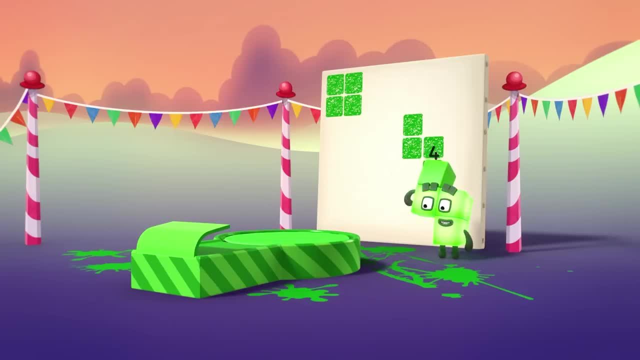 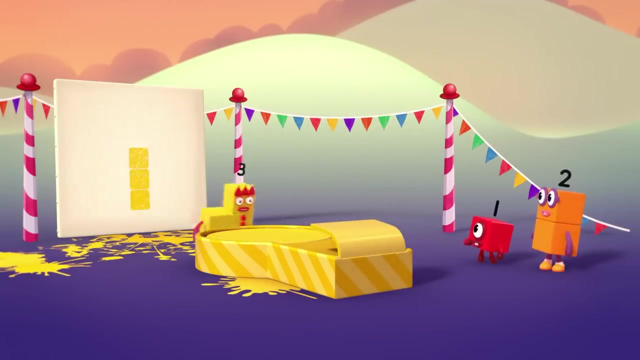 Of course it is One, two, three, four, Four blocks. See Whee. Whatever way round I go, I'm still four Whee. Look at me Whee, I'm still three, Whee, Whee. 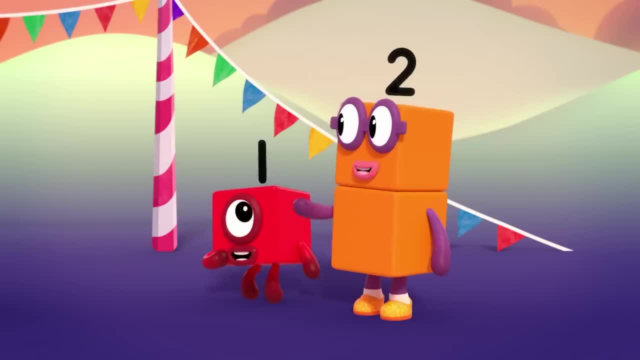 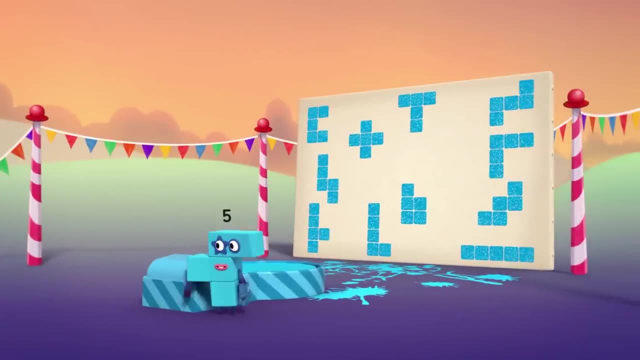 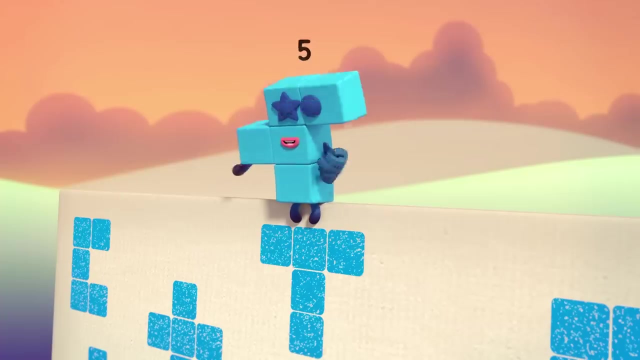 Bum, bum, bum. Ooh, not bad. You think that's amazing? You should see five, Hmm, Five. Did you make all these shapes? I did so. The more blocks you have, the more shapes you can make. 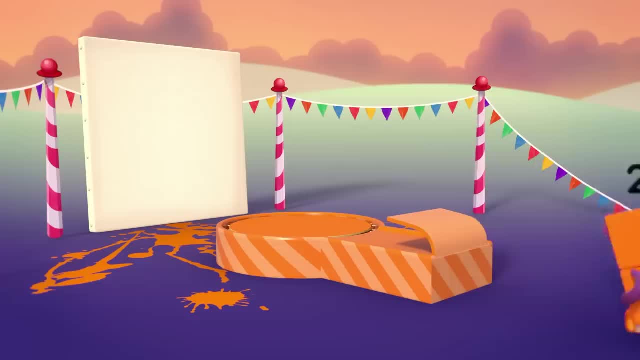 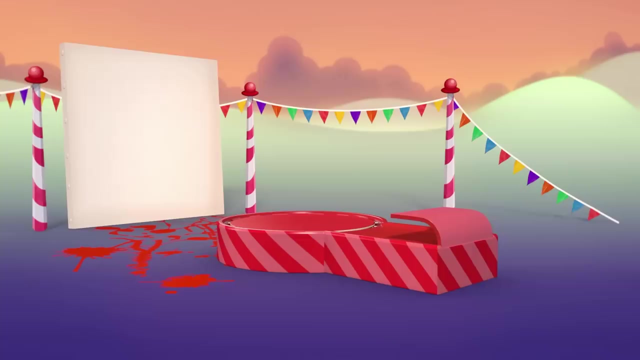 Ha, Oh, My turn, Not bad. two, Of course, they're not really different shapes, are they? It's the same shape. One goes, Oh, it's still better than me. Look, That's all One shape. 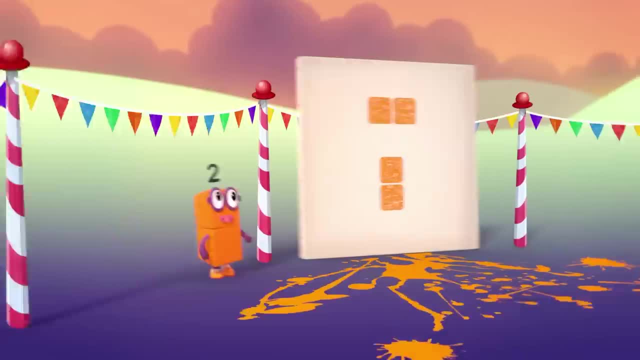 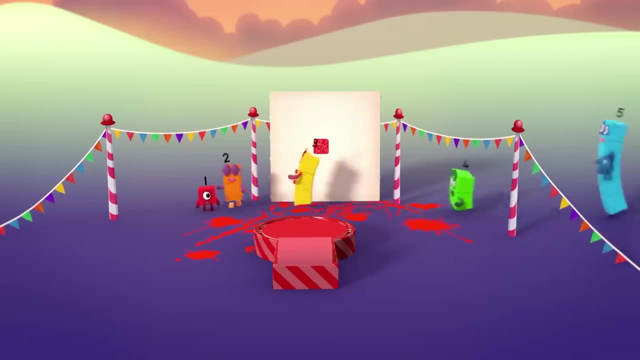 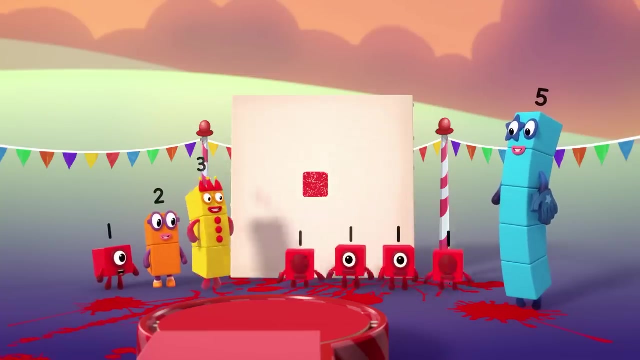 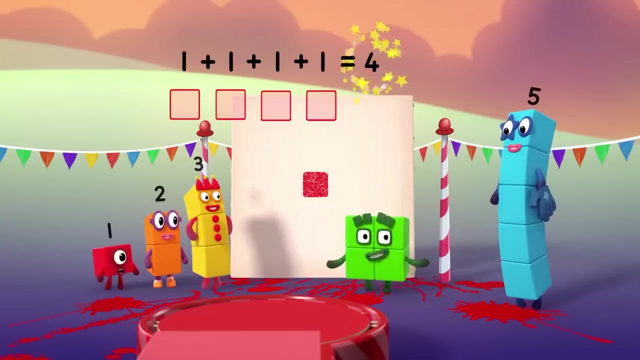 Not very exciting compared to all of you. Now, now, now You're forgetting something. One, two, three, Boo, Hey. One plus one plus one plus one equals four. Every big shape is made up of lots of little ones. 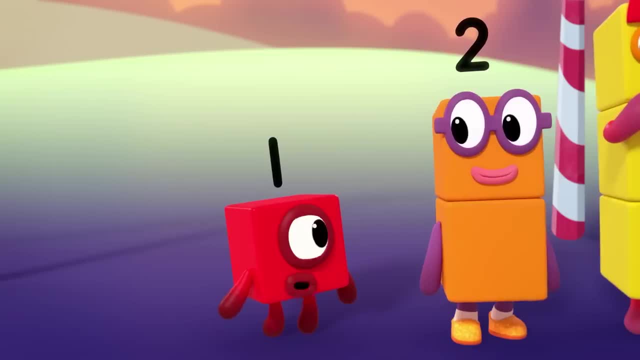 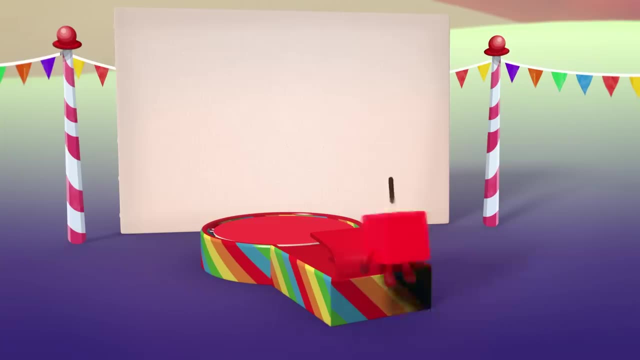 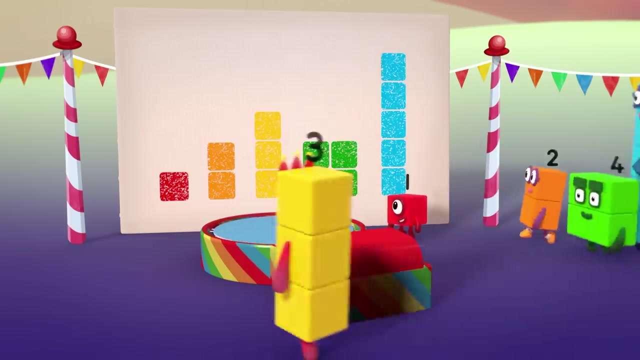 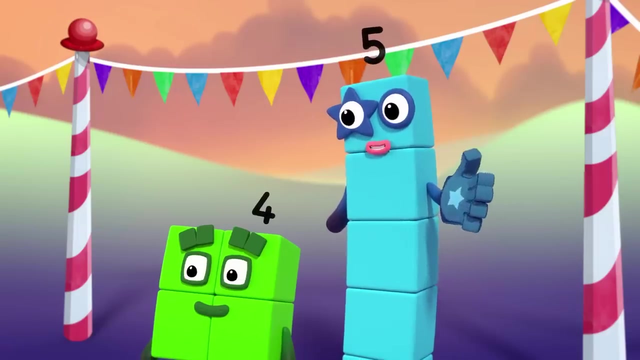 So lots of little ones can make every big shape. Look what I can do. You made all of us Well done, And just in time for the grand finale. What better way to celebrate opening my new park than with fireworks? Ooh. 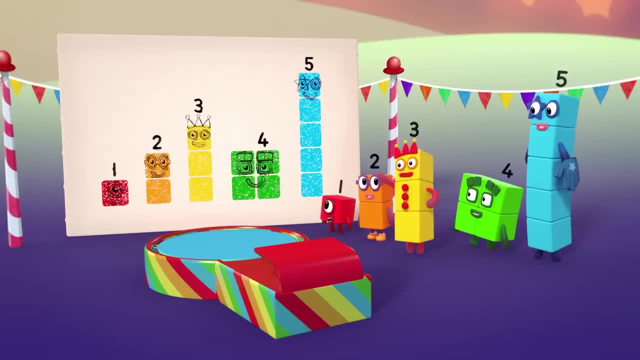 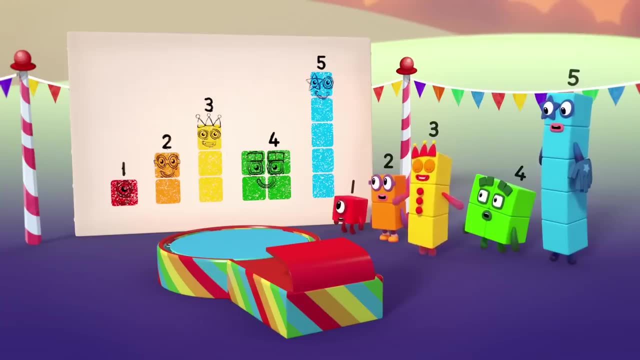 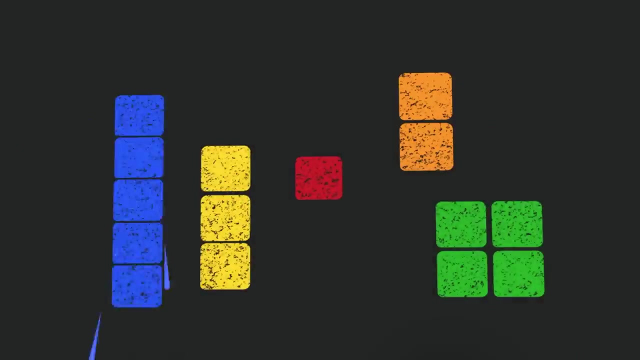 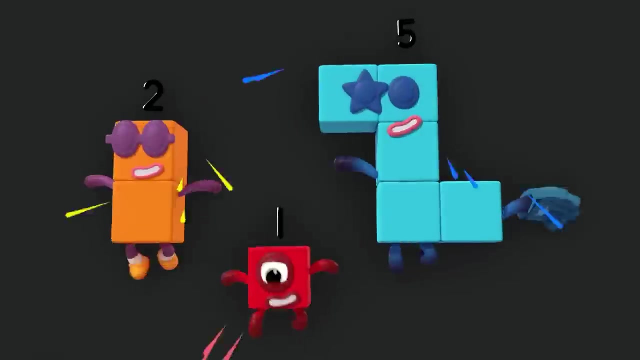 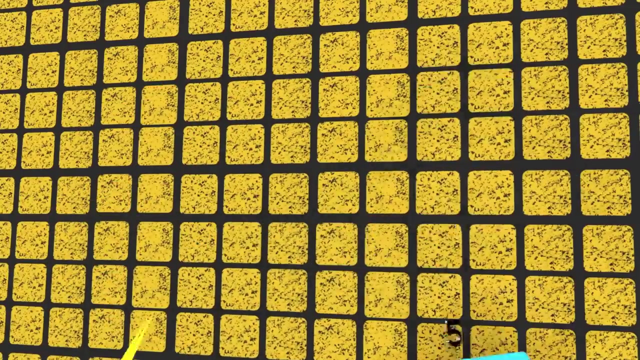 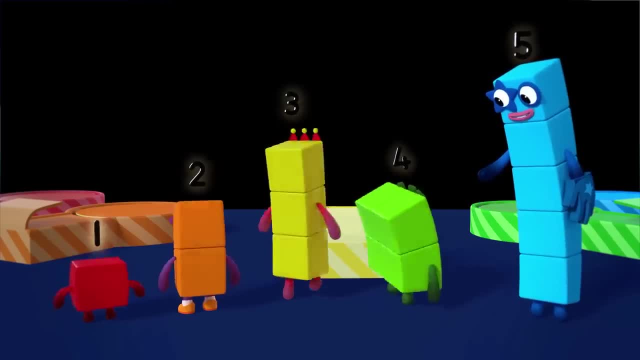 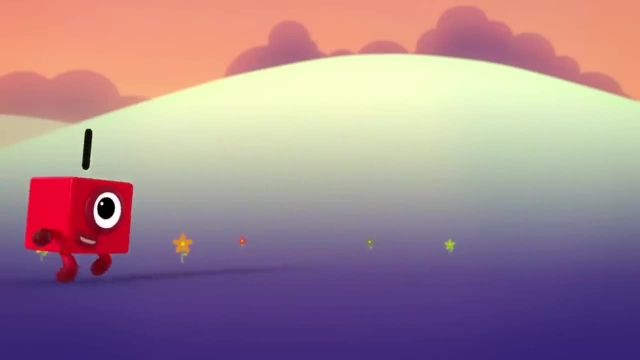 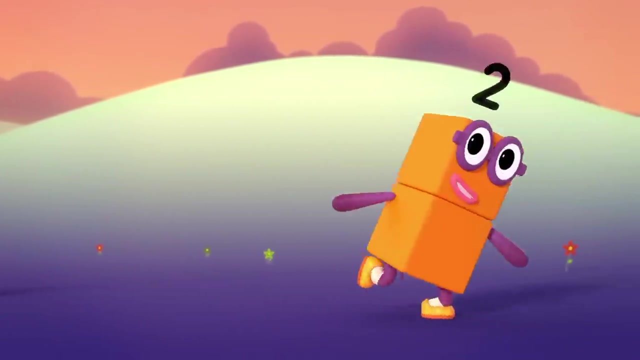 the sky's the limit. They're like stars: One, two, three, Yay, Whoo-hoo, I'm number one And this is fun. I've got one block to play with And the whole of me is one, One, One, two, one, two. 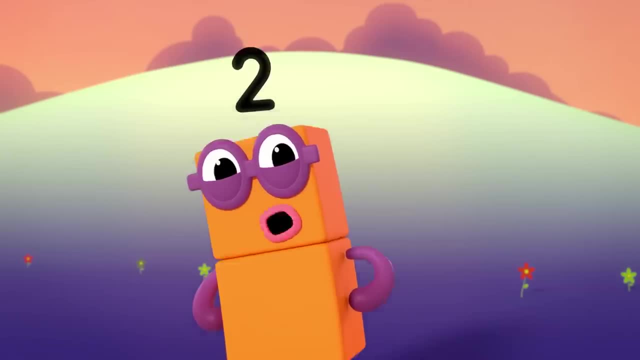 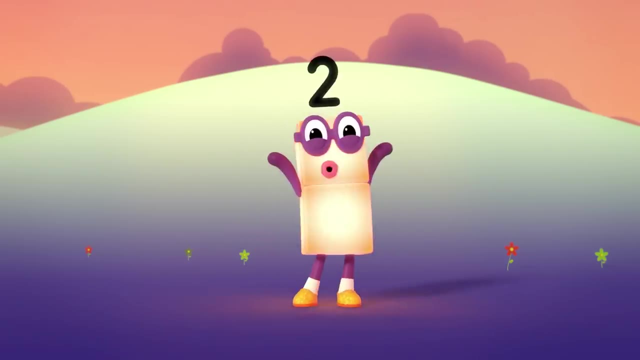 I'm number two. How do you do? I've got two blocks to play with And the whole of me is two. One, two. One is a part of me And one is a part of me, And the whole of me is two. Watch, I'm one. 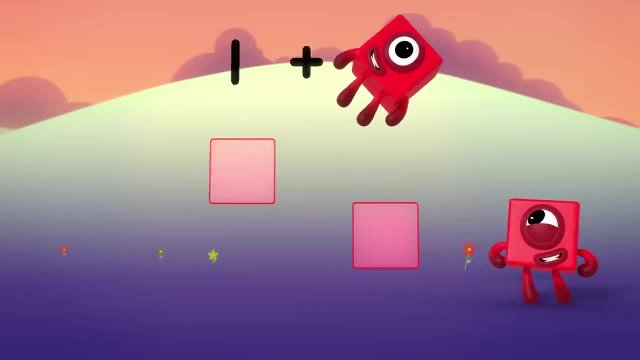 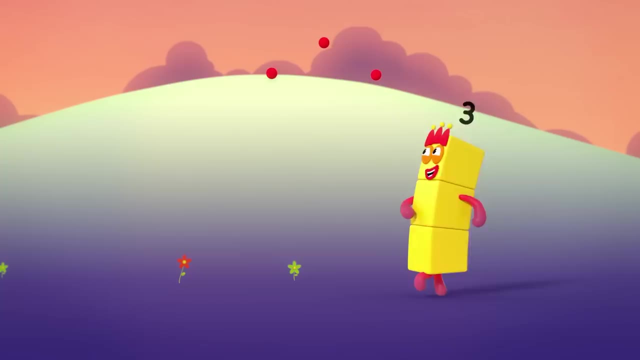 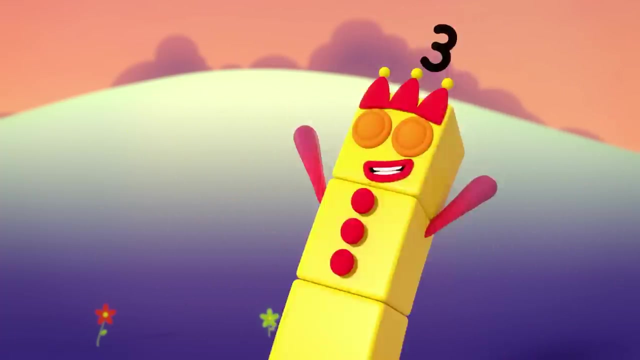 And I'm a part, I'm one And I'm a part, And the whole of me is two, One, two, three, One, two, three, One, two, three. I'm number three. Now look at me. I'm the best of all, the number blocks. 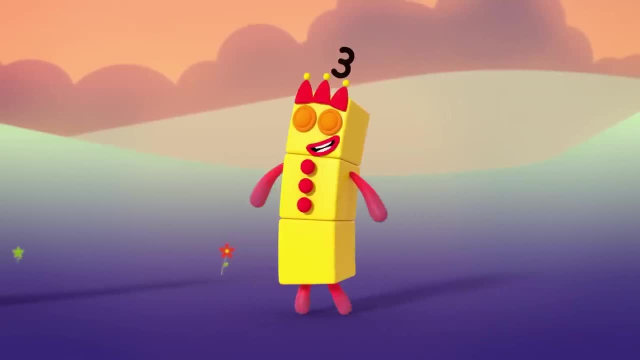 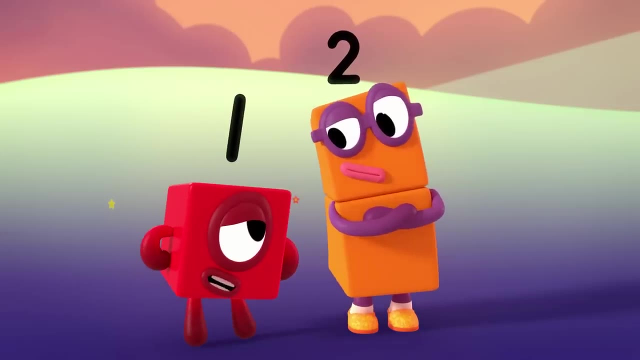 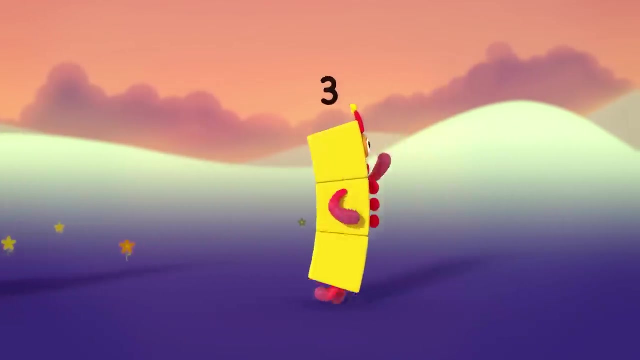 As you can play And finally see The whole of me is amazing. The whole of me is so great. The whole of me is Sorry. Three, Try again. Okay, I'm number three. Yes, look at me, I'm the best of all the number blocks. I'm number three. 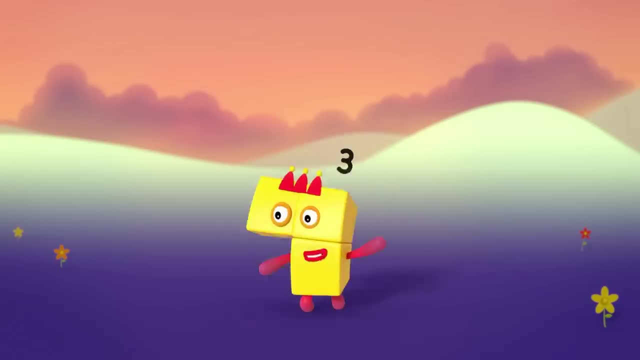 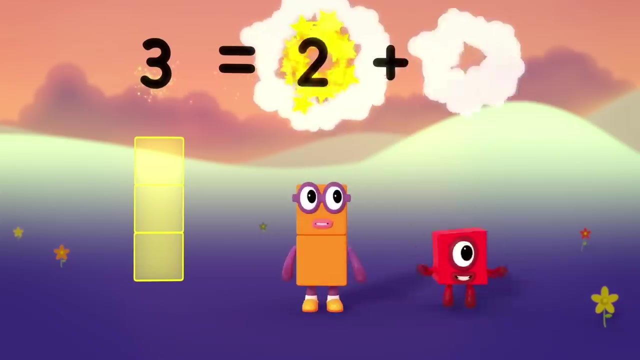 Now look at me. I've got three blocks to play with, And the whole of me is three. One, two, three. One is a part of me And two is a part of me, And the whole of me is three. Watch, I'm two And I'm a part. 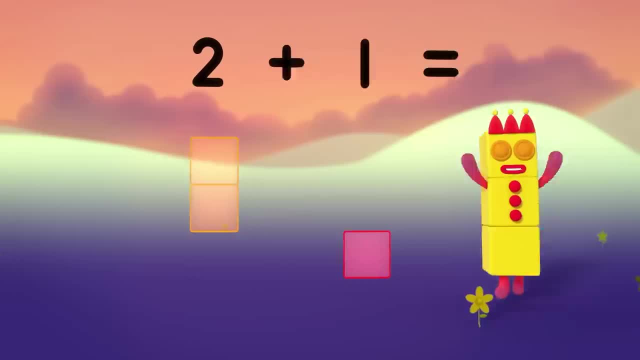 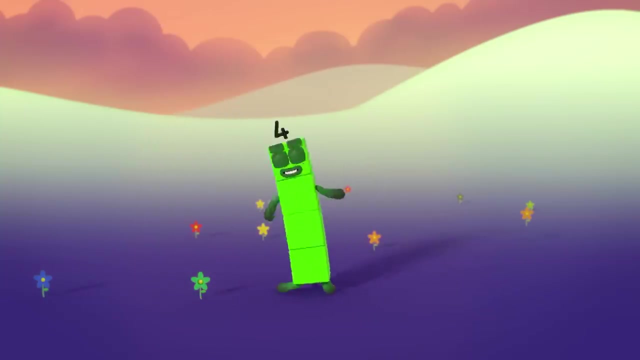 I'm one And I'm a part, And the whole of me is three. One, two, three. I'm number three, I'm number four And I am sure That I've got four blocks to play with, And the whole of me is four. One, two, three, four. 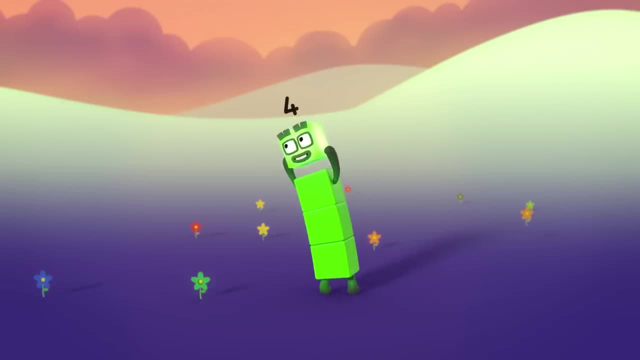 One is a part of me And three is a part of me, And the whole of me is four. Watch, I'm three And I'm a part, I'm one And I'm a part And the whole of me is four. Now, here is my number four. Now, here is something more. 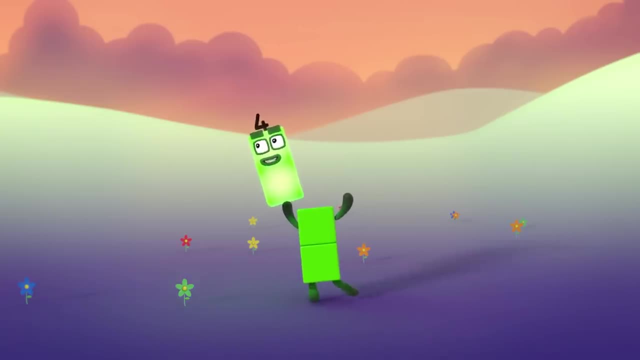 That's different from before. Two is a part of me And two is a part of me, And the whole of me is four. Watch, I'm two And I'm a part. I'm two And I'm a part, And the whole of me is four. I'm a square, look. 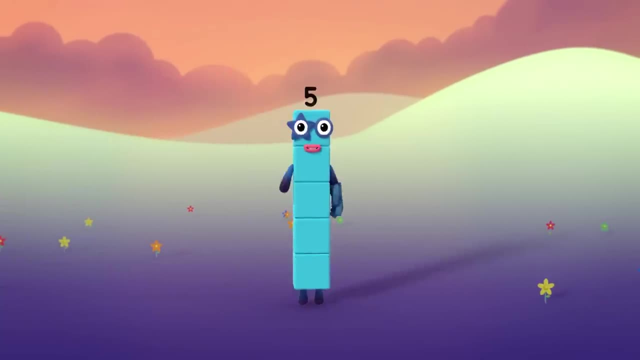 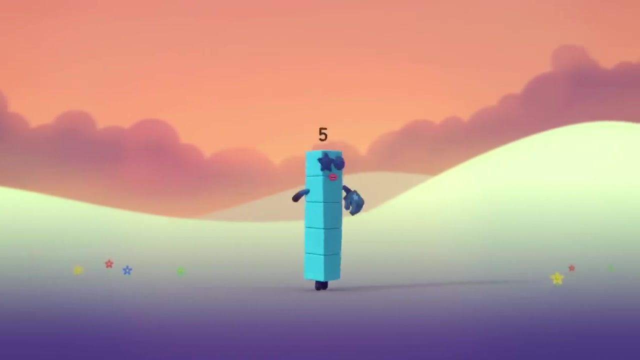 Four sides, four corners. I'm number five, I am alive, I've got five blocks to play with And the whole of me is three. me is five, One, two, three, four, five. One is a part of me and four is a part of me, and 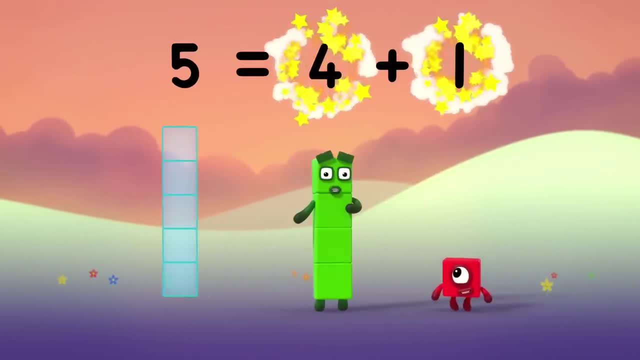 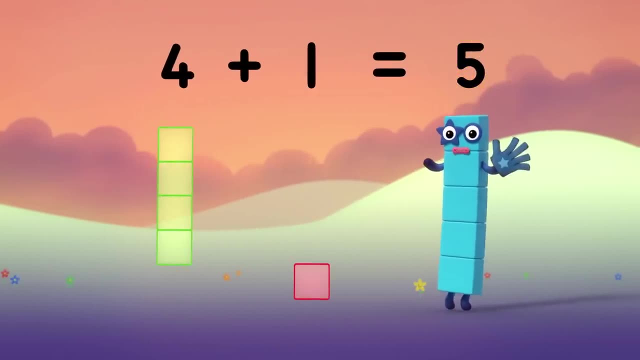 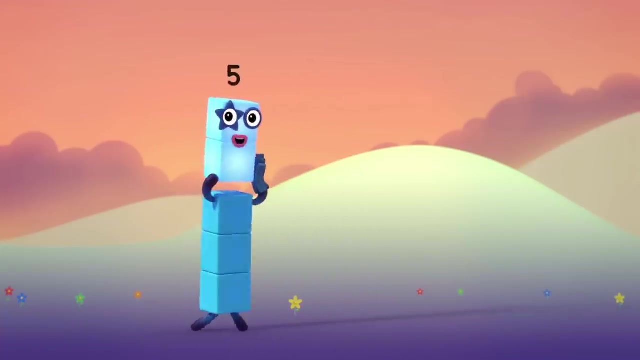 the whole of me is five. Watch, I'm four and I'm a part. I'm one and I'm a part And the whole of me is five. But now I feel alive, going into overdrive. Two is a part of me. 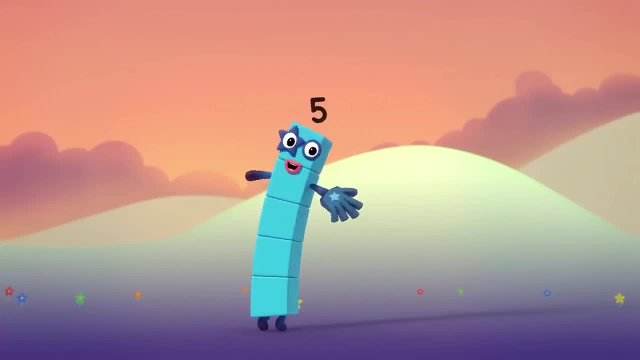 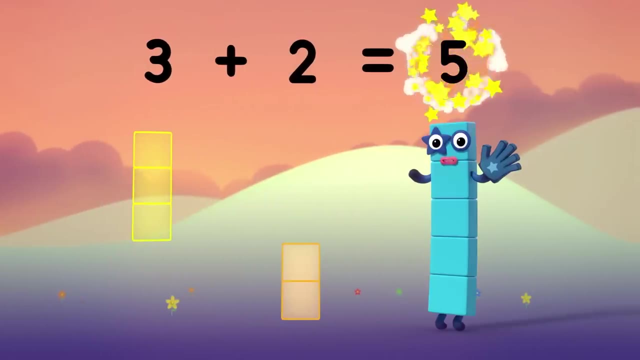 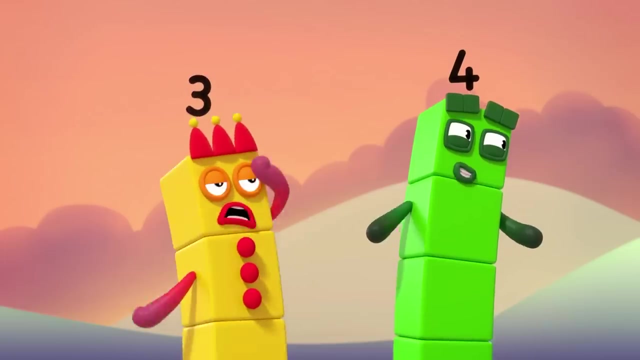 and three is a part of me and the whole of me is five. Watch, I'm three and I'm a part. I'm two and I'm a part And the whole of me is five High five. Making friends is easy when you can come apart. Splitting up is not so hard. it won't break your heart. So when? 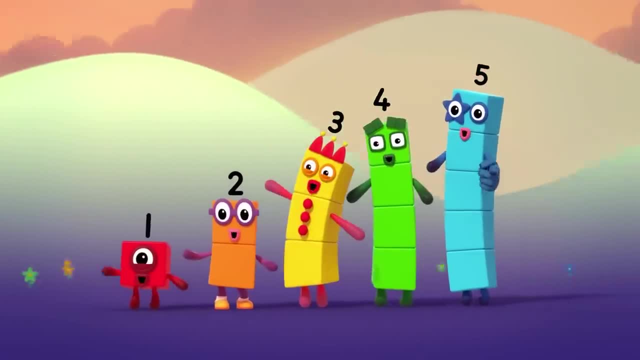 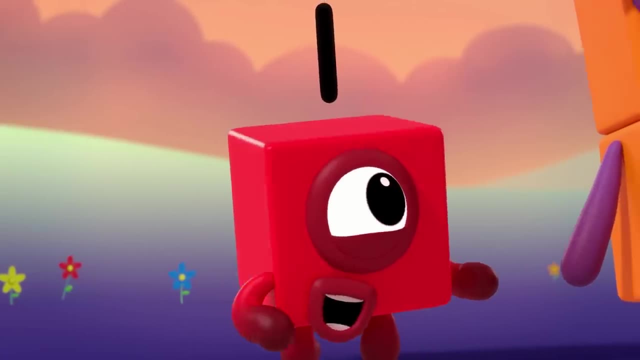 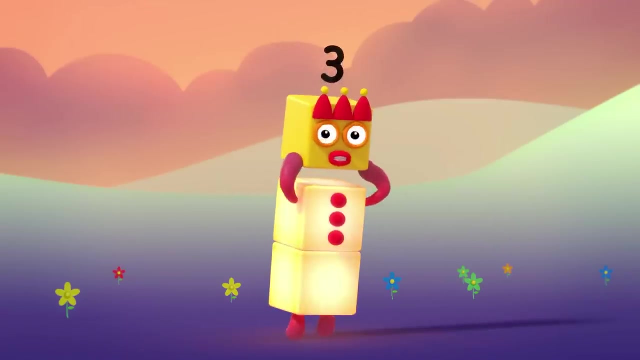 we fall to pieces, we have lost control, A hole is made of all its parts and the parts they make a whole. Just remember that One is a part of me and one is a part of me. One is a part of me and two is a part of me. 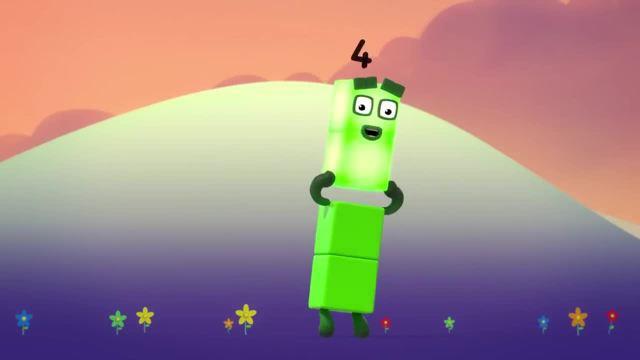 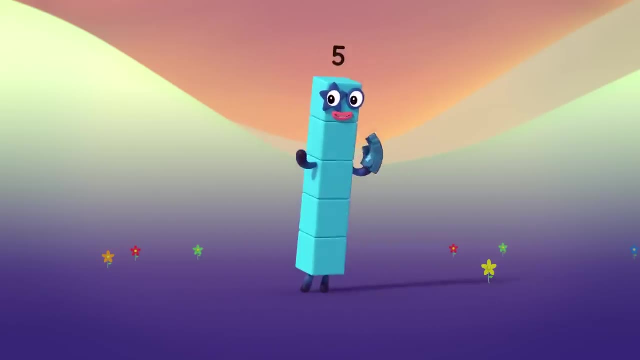 One is a part of me and three is a part of me. Two is a part of me and two is a part of me. One is a part of me and four is a part of me. Two is a part of me and three is a. 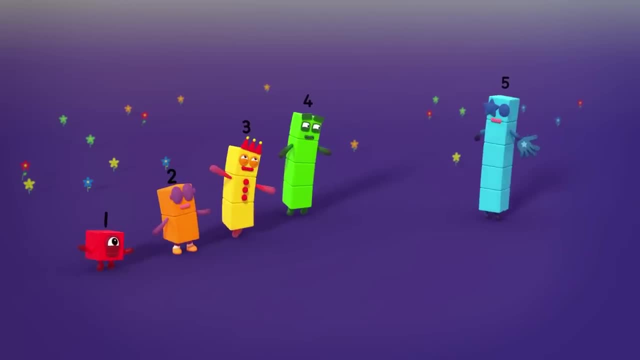 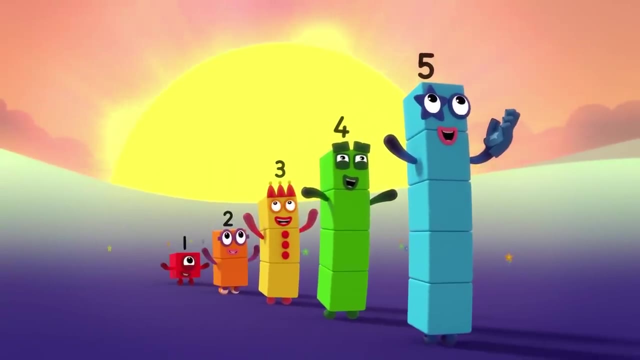 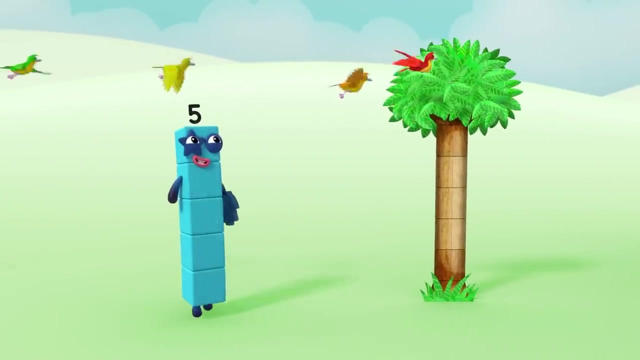 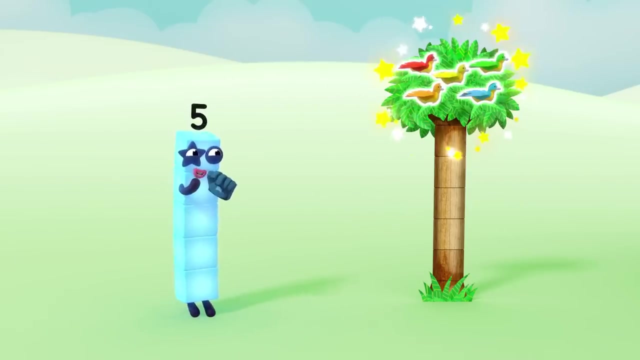 part of me And the whole of me is one, two, three, four, five. One, two, three, four, five. Here I am, and I am five. One, two, three, four, five, Five little birds have just arrived. One, two, three, four. 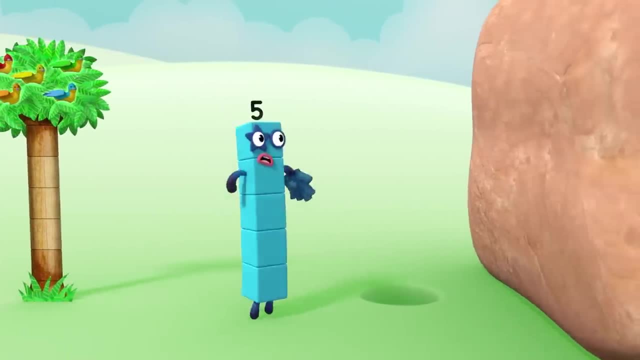 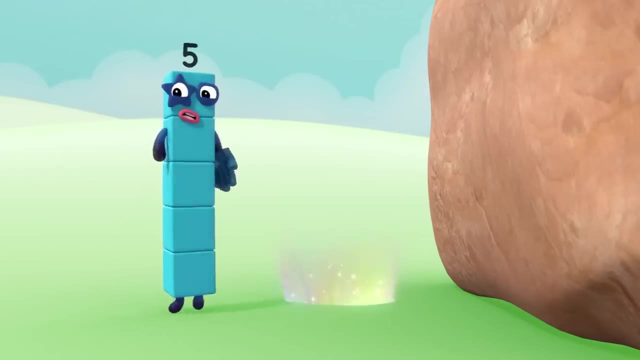 five. What a wonderful day to be alive. A giant rock in front of me. How can I get where I need to be? What is that? What is that? What is that silly sucking sound? Oh, look a hole so big and wide. Why is it there? I? 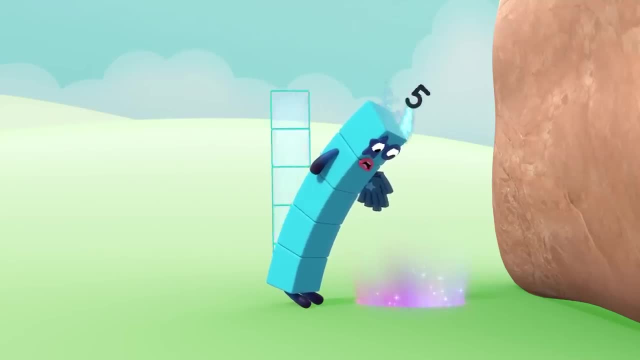 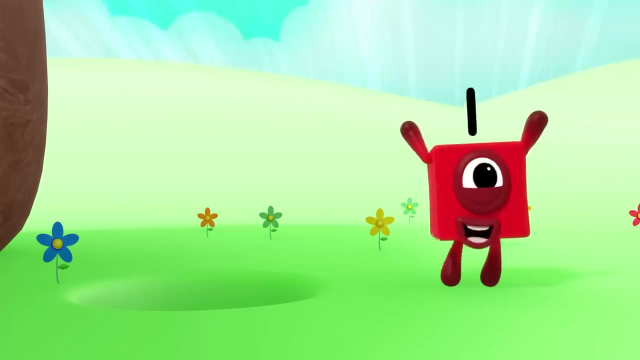 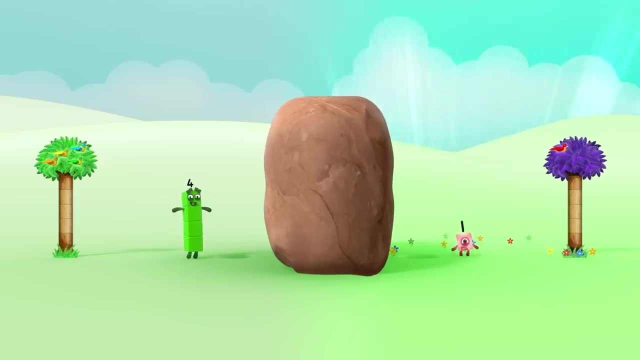 Now, I am four and here I am. I am one, Here I am, The wonderful day to be alive. What a wonderful day to be alive. Where, oh, where, oh, where is five? Where, oh, where, oh, where, oh, where is five? 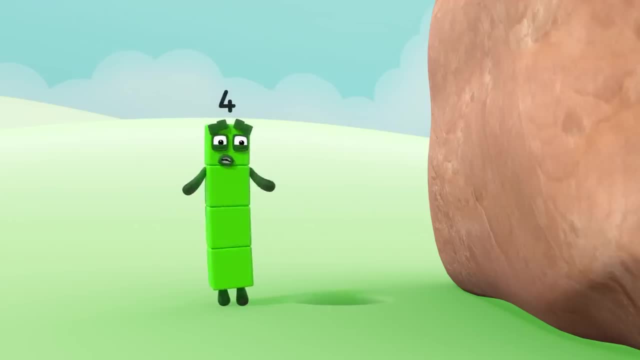 Five is gone. Where did she go? Is she all right? I do not know. Is she here? Is she there? I must keep looking everywhere. What is that silly sucking sound? A giant hole so big and round. Why is it there? I? 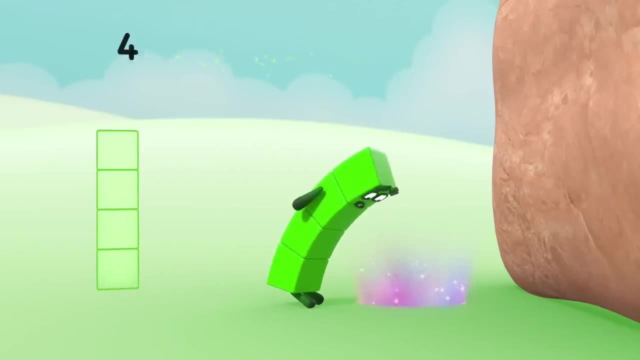 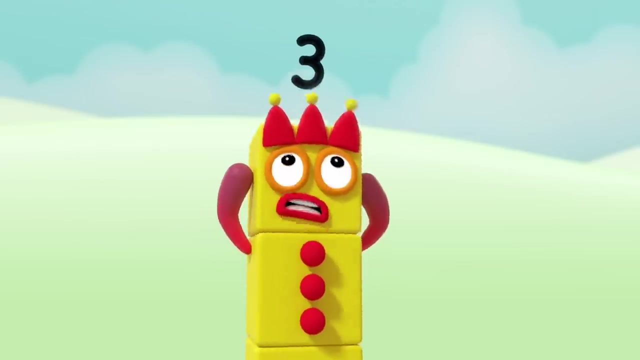 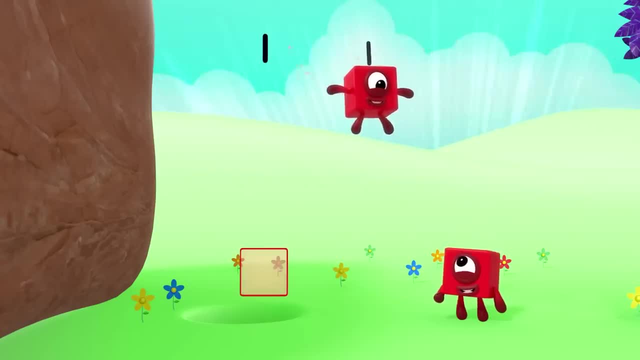 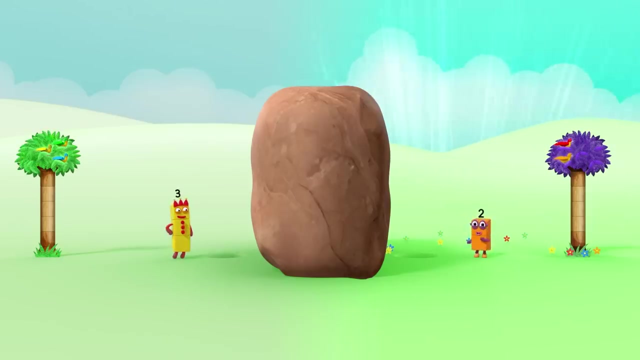 I am one. That was fun. One plus one equals two. What is happening to me? I just got bigger, did you see? Now I am three and here I am. Now I am two and here I am. What a wonderful day to be alive. But where, oh, where, oh, where is five? 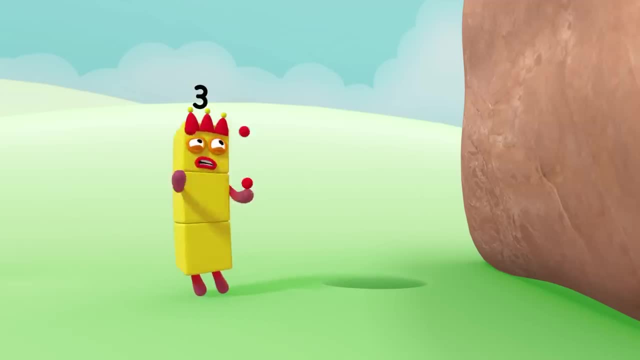 I was five, then four, then three. Someone has played a trick on me. I do not mind at all. you see, Three is who I want to be. What is that silly sucking sound? A giant hole so big and round. 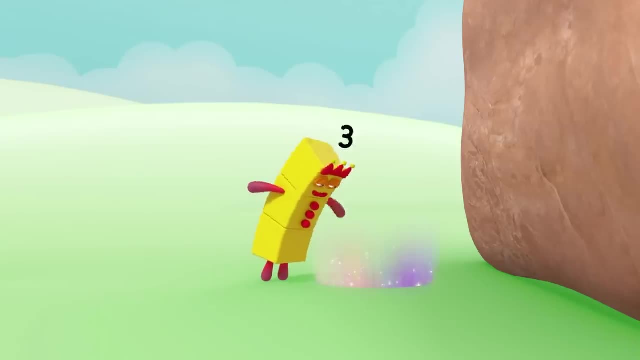 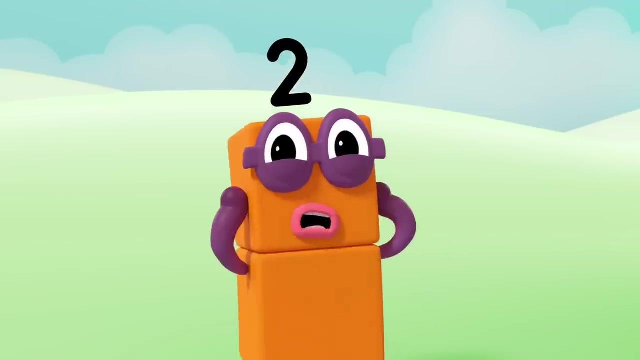 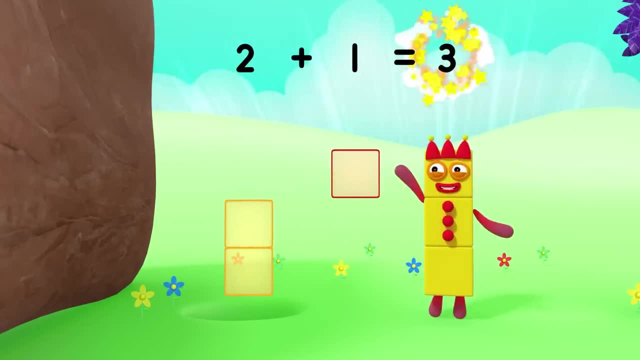 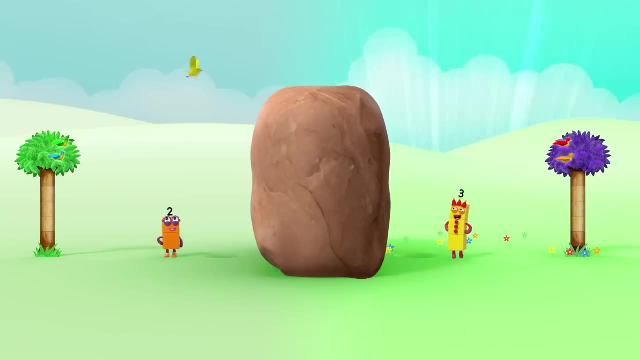 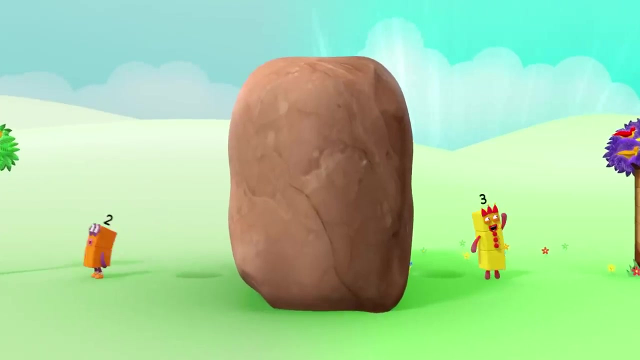 Two plus one equals three. What is happening to me? I just got bigger, did you see? Now I am two and here I am. Now I am three and here I am. What a wonderful day to be alive. But where, oh, where, oh, where is five? 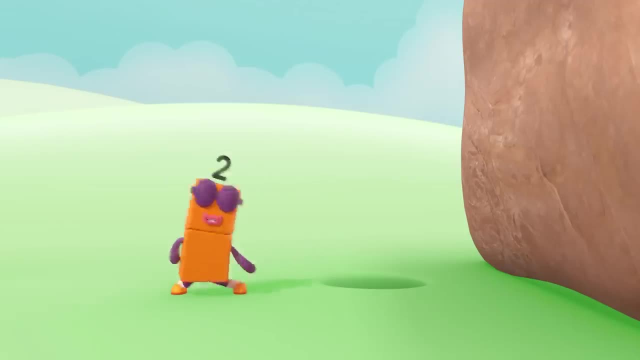 I wonder where the ones will go. I think I've got it now. I know Every time we get one smaller, someone else is getting taller. What is that silly Sucking sound? A giant hole so big and round? Why is it there? I do not know. I wonder what is down below. 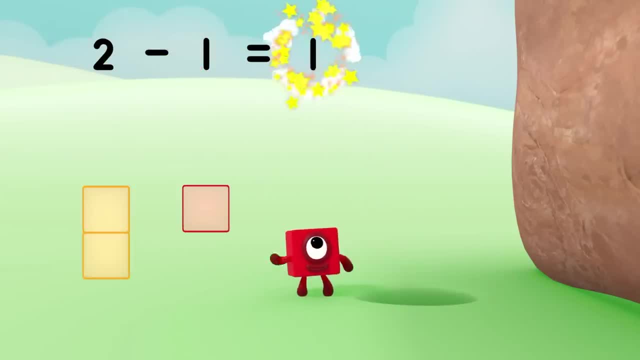 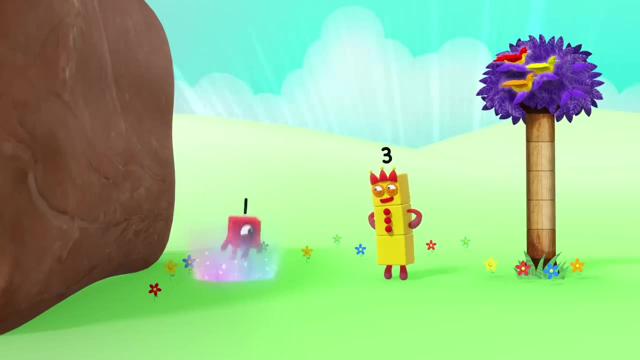 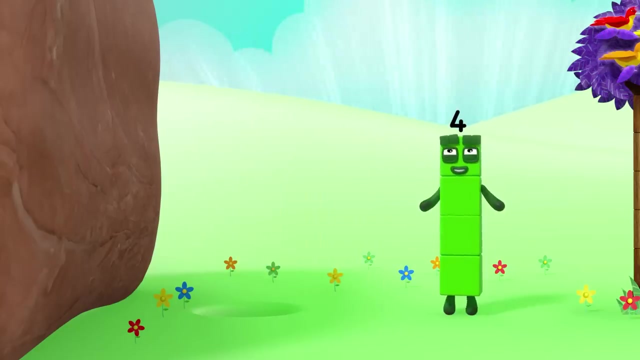 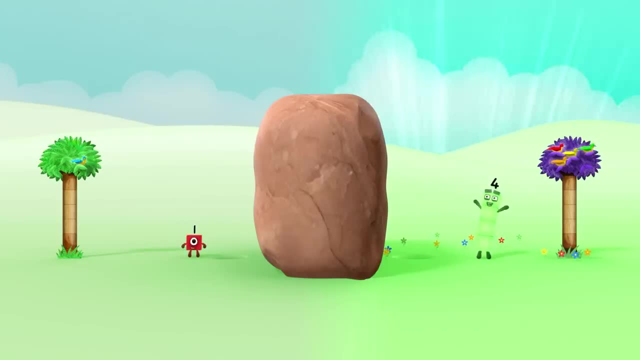 I just got bigger, did you see? I am one, That was fun. Three plus one equals three. What is happening to me? I just got bigger, did you see? I am one? That was fun. Three plus one equals three. 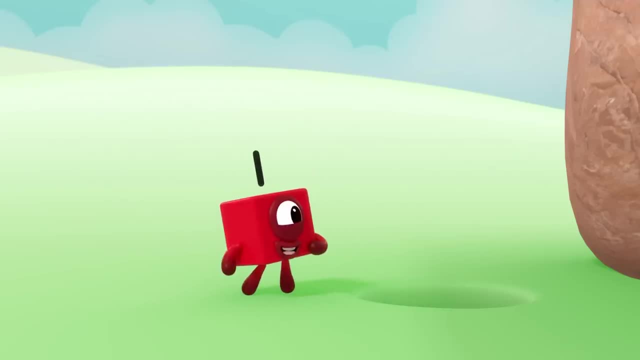 Now I am four and here I am. Now I am four and here I am. What a wonderful day to be alive. But where, oh where, oh, where, is five, Five, four, three, two, one someone's having lots of fun? 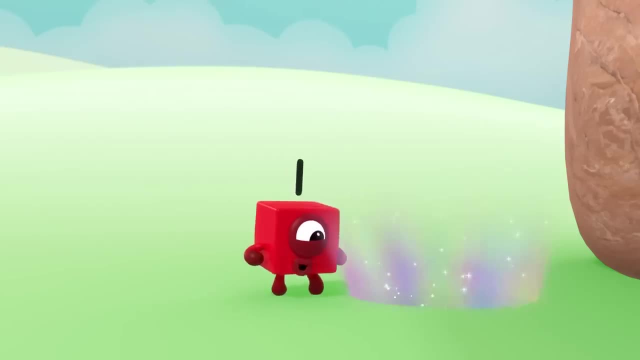 Now I know where five will be. Four is waiting there for me. What is that silly Sucking sound? A giant hole so big and round? Why is it there? I think I know. I think I know what's down below. 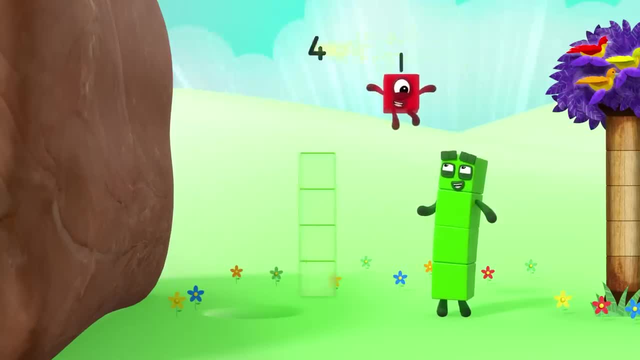 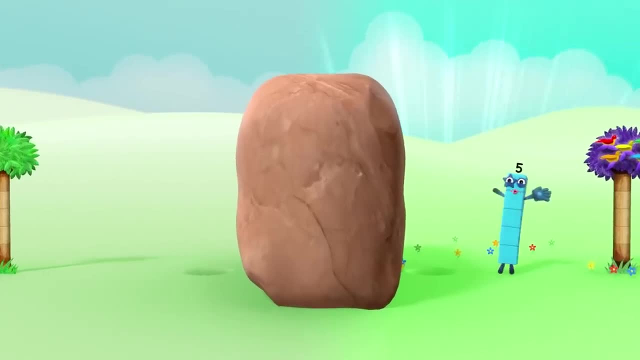 What is happening to me? I just got bigger, did you see? What a wonderful day to be alive, But where, oh, where, oh, where is five? What a wonderful day to be alive, But where, oh, where, oh, where is five? 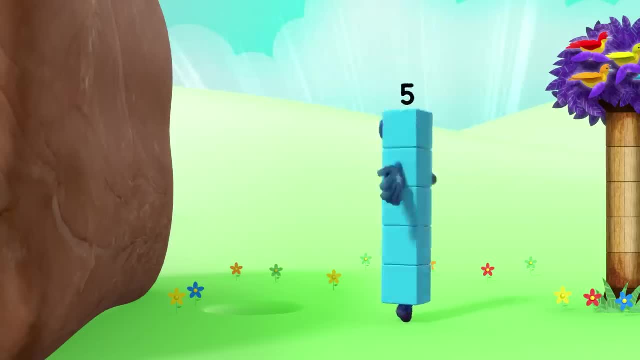 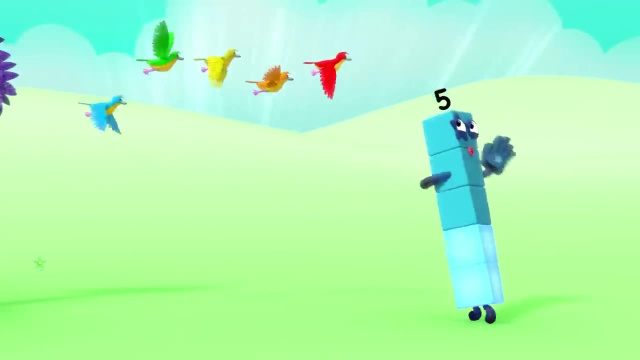 Here I am and I am five. Here I am and I am five. What a wonderful way to arrive. What a wonderful way to arrive: One, two, three, four, five. What a brilliant, amazing, fantastic, terrific and wonderful day to be alive. 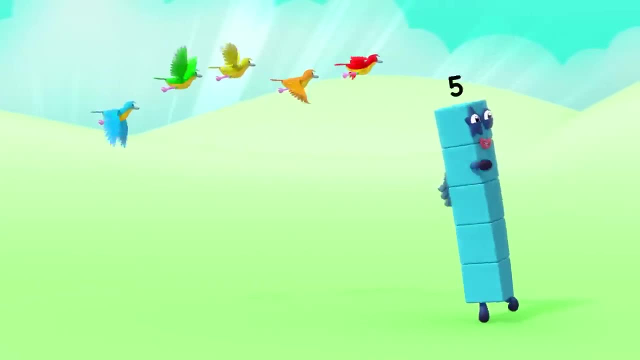 What a brilliant, amazing, fantastic, terrific and wonderful day to be alive. What a brilliant, amazing, fantastic, terrific and wonderful day to be alive. One, two, three, four five. One, two, three, four, five. 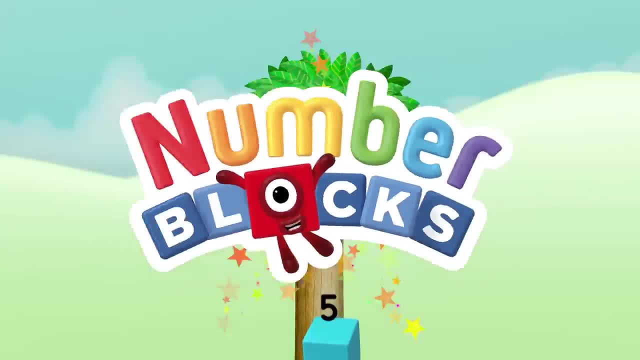 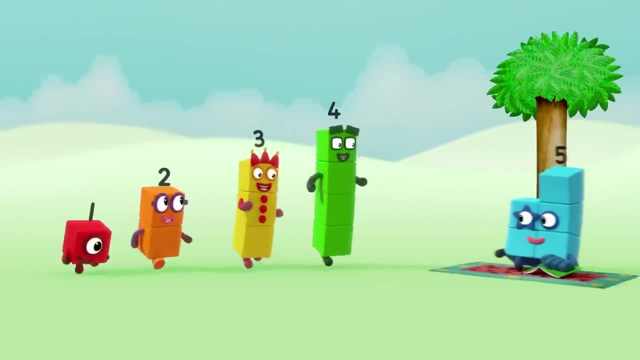 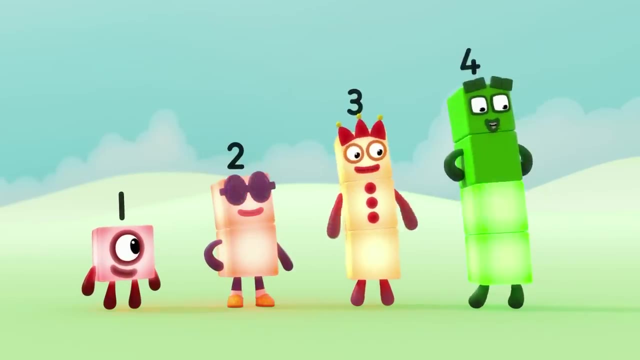 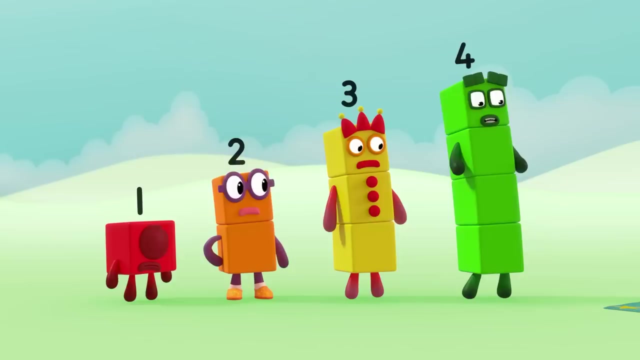 Sh Oi, Oh Yep, Hey, Found you There she is. Hello, We're playing Hide and Seek. Want to join in? I would absolutely love to You hide and I'll seek. Huh, You won't find us sat there. 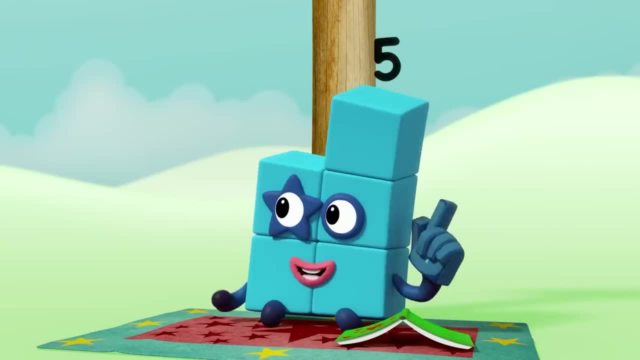 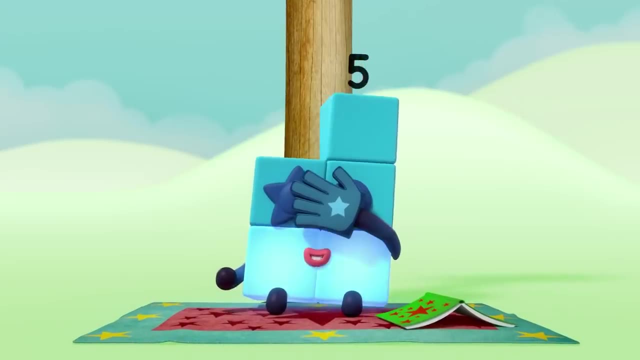 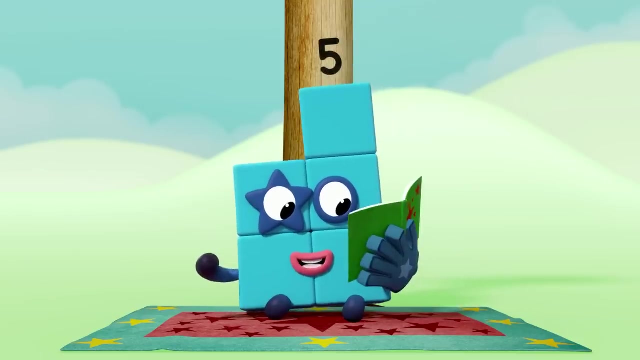 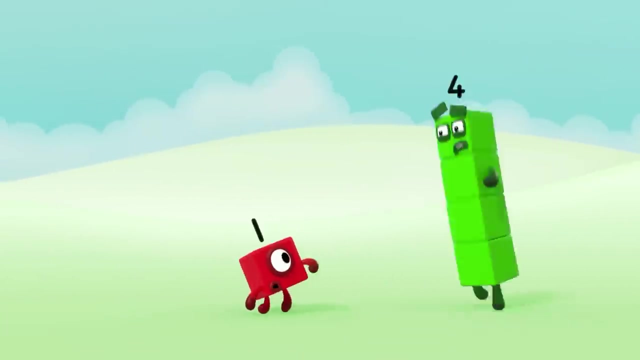 Oh, will I not? now? I'm good at this game. I'll find you and point you out: One, two, three, four, five, Ready or not? here I Get on with my book. Three hide behind me. 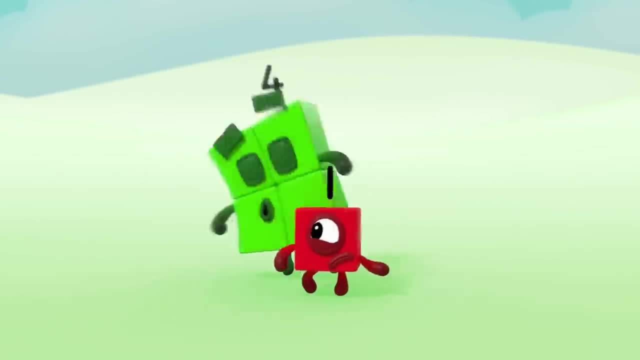 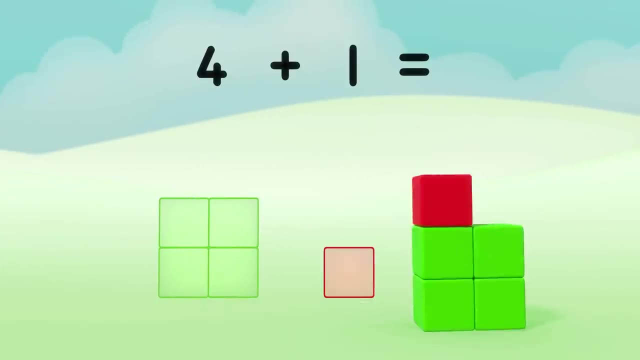 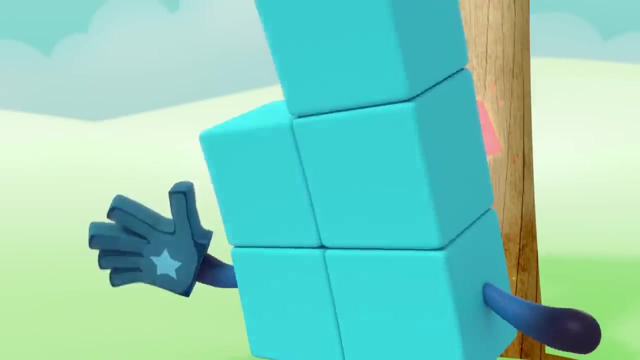 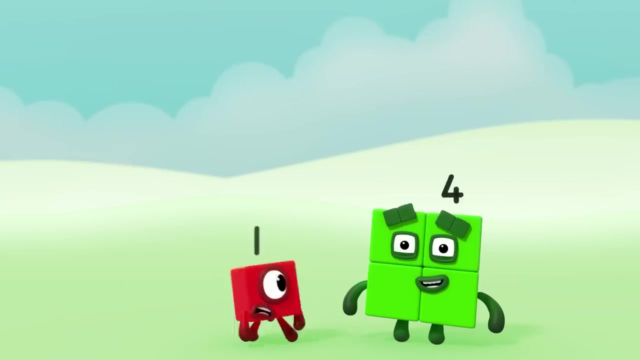 Where can I hide? I know behind you Four. Oops, Four Plus one Equals five. Ready or not, here I come. Find you four, find you one. Five minus one Equals four. Look Five, said she'd point us out. 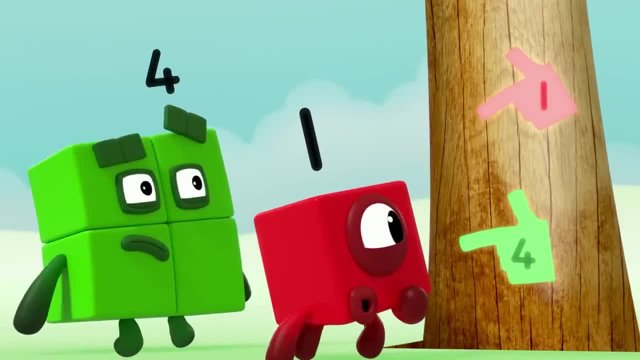 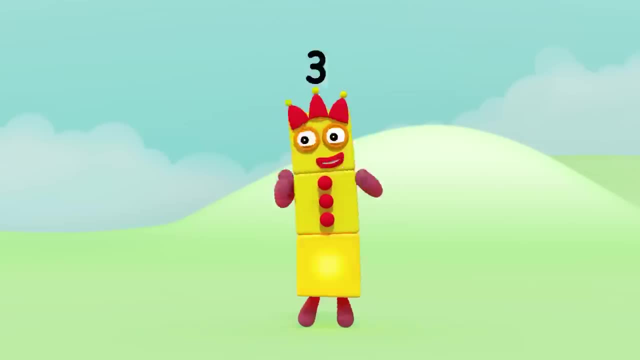 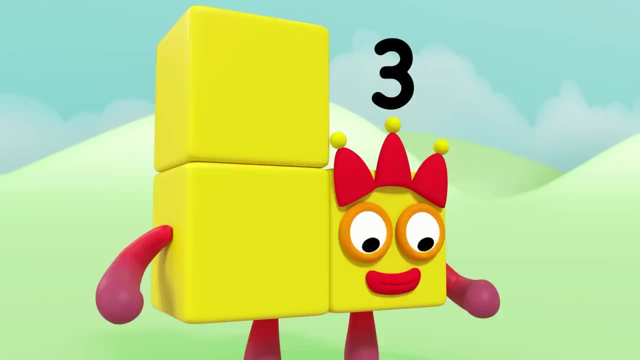 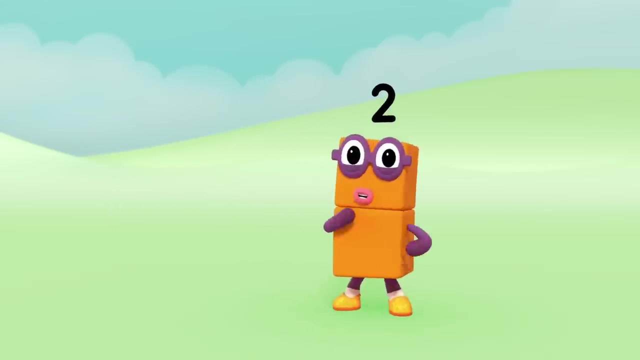 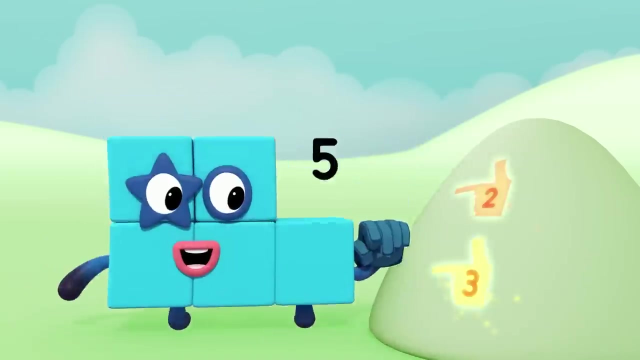 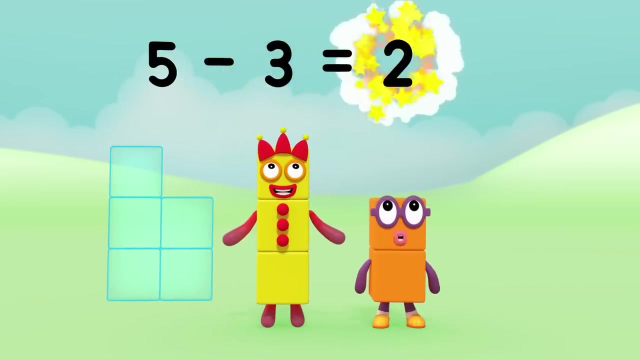 Five was right here. How, Oh, I am three, master of disguise, Shhh, Shhh. Two plus three equals five. Ready or not, here I be. Find you two, find you three. Five minus three equals two. 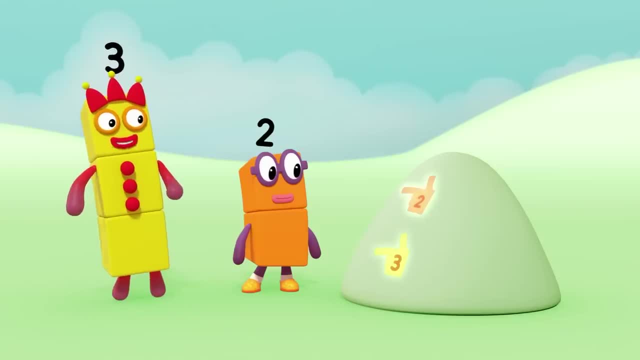 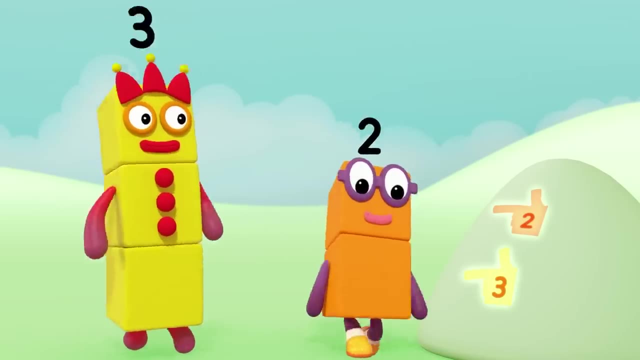 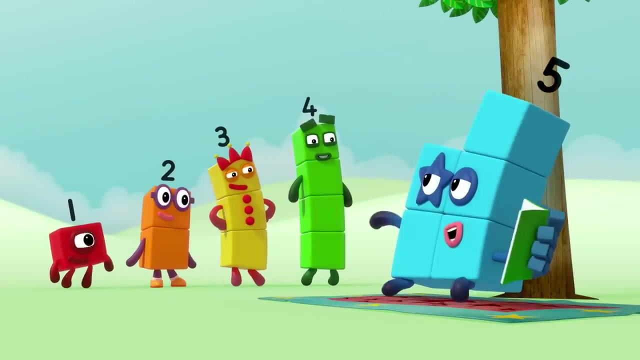 A pair of pointing prints. Five found us, But but how? Five. One, two, three, four, five, Five You're here. How did you Told you I was good? Now my turn to hide. 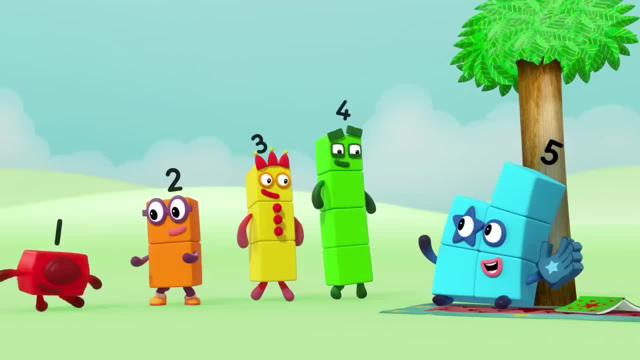 One, two, three, four. Ready or not? five, here we come. Ha ha, ha, Ooh, Aw, you guys. Oh, you're so cute. Ready or not? five, here we come, Ooh. 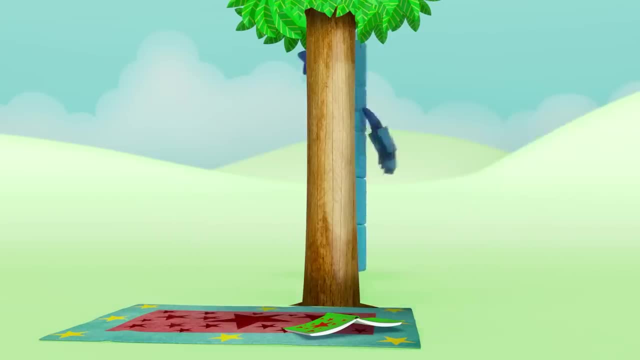 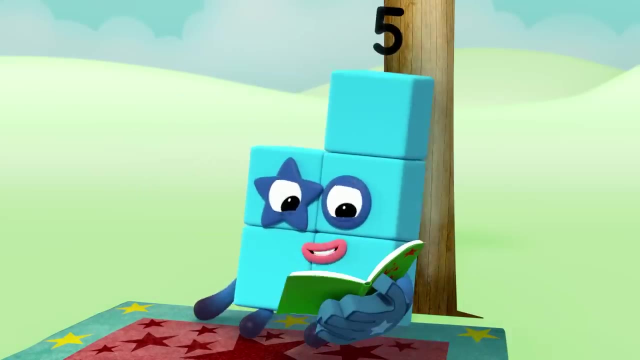 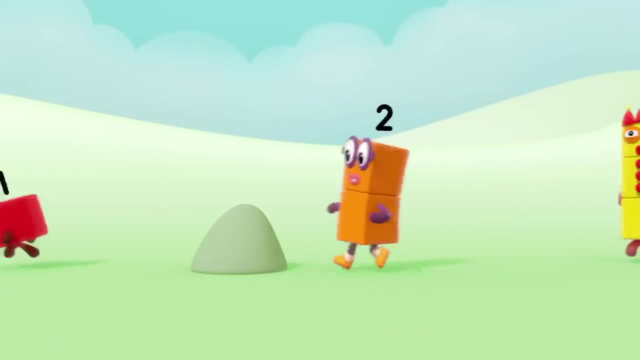 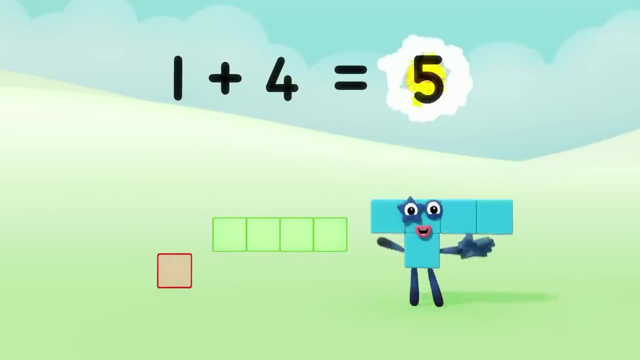 Ooh, Ha, ha ha. Ready or not? five, here we come. Oh, Ready or not five, here we come. Ooh, Hmm, Oh, Oh, Oh, Oh, Oh Rock. One Plus four equals, five. 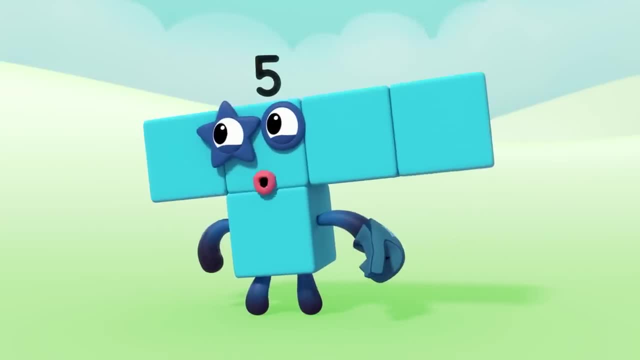 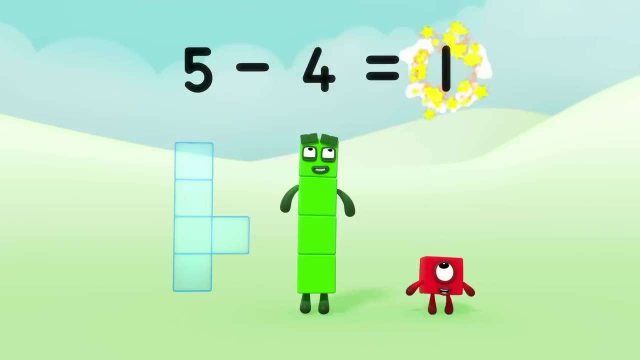 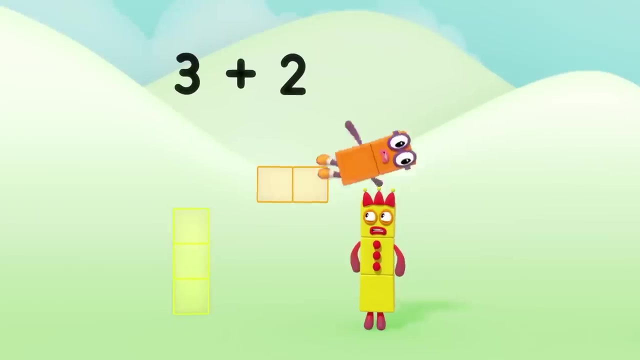 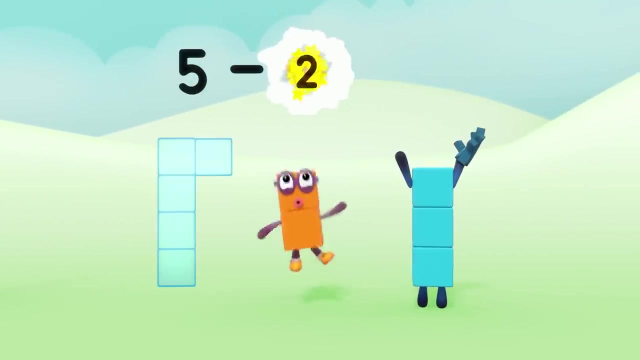 Found you Amazing. Can you find me again? Five Minus four Equals one. Come on, Rock. Three Plus two Equals five. Found you Fantastic. Can you find me again? Five Minus two Equals three. 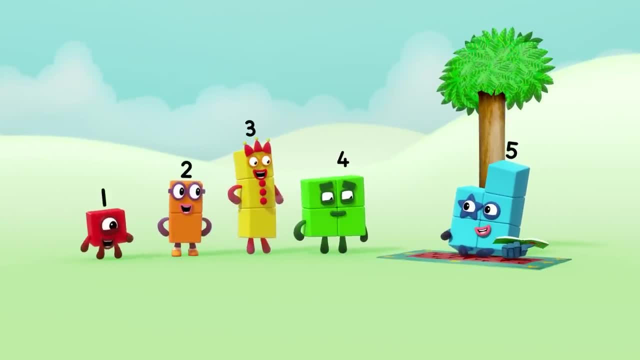 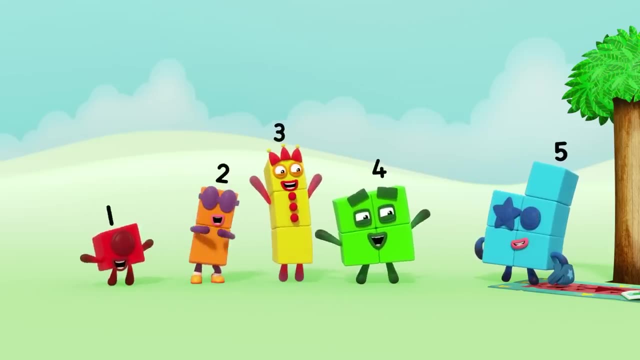 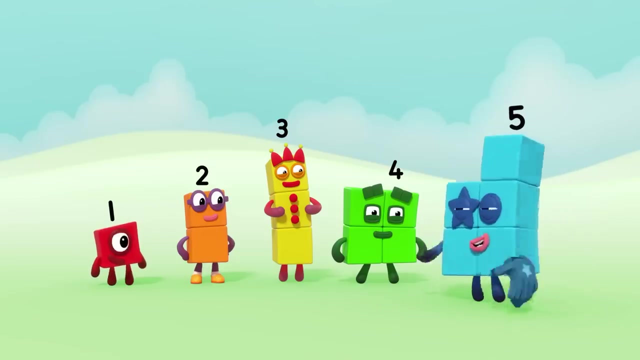 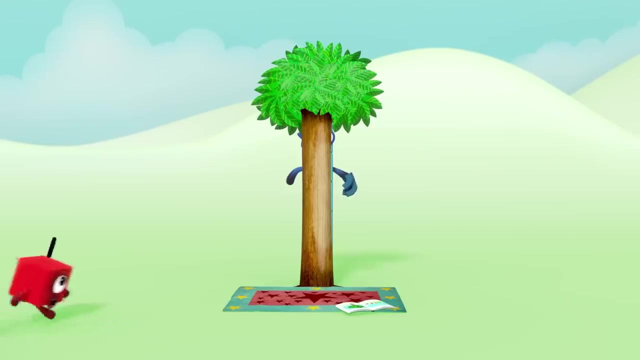 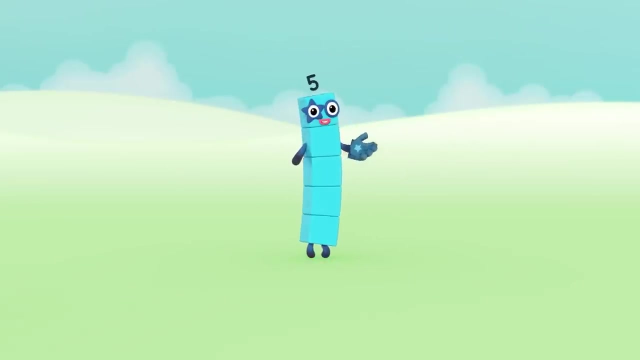 Found you, You stars, You all found me. Can you teach us to be as good at hide-and-seek as you? Sure I can Try this. Ah, Four, Four, Oops. Once upon a time there were three little pigs. 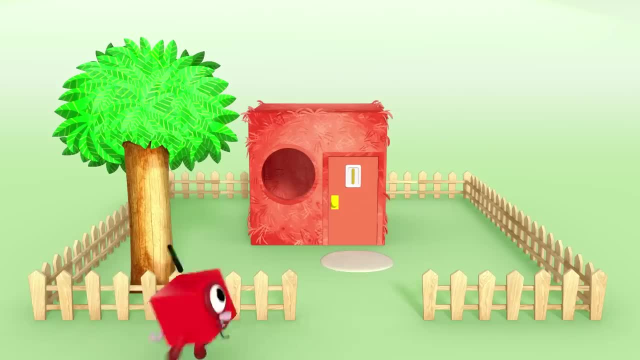 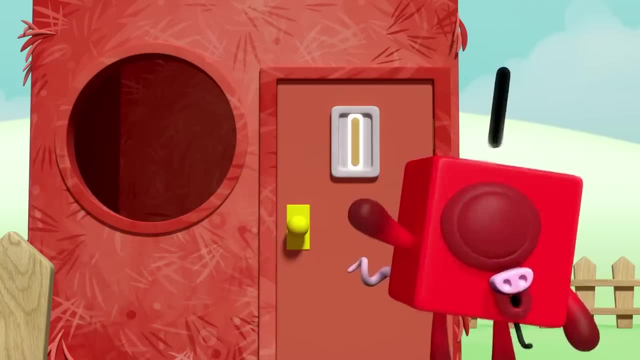 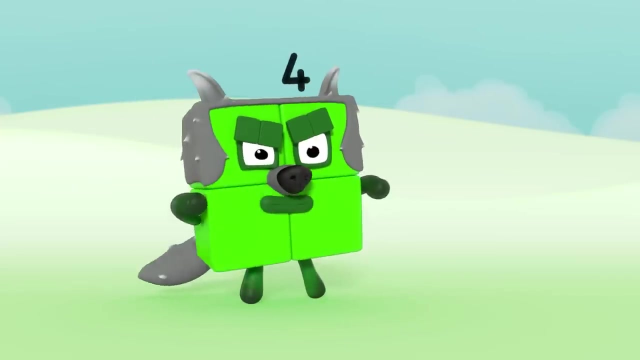 The first little pig had a house with one room. Look, It has one one window and one one tree in the garden And there's a number one on the door. But then came Ha-ha, The big barred square. 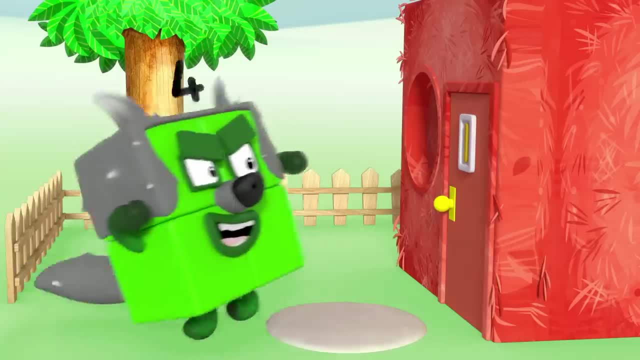 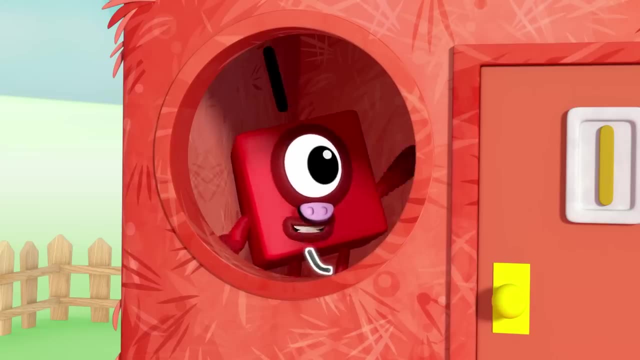 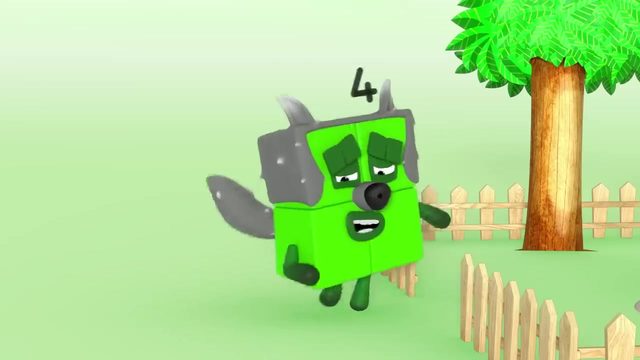 Roar, Little pig, Little pig, Let me in. Let me in, Not by the hair on my chin, Then I'll hoof and I'll poof and I'll blow your house in Shame. That's so square. 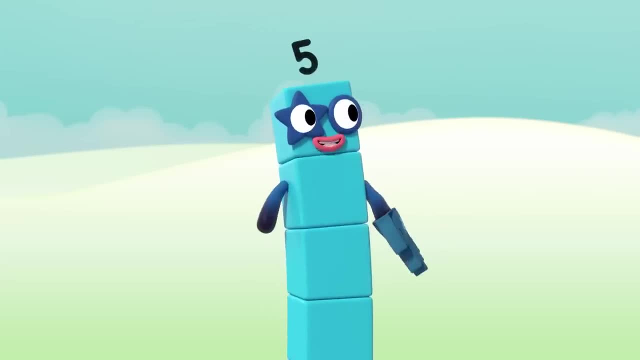 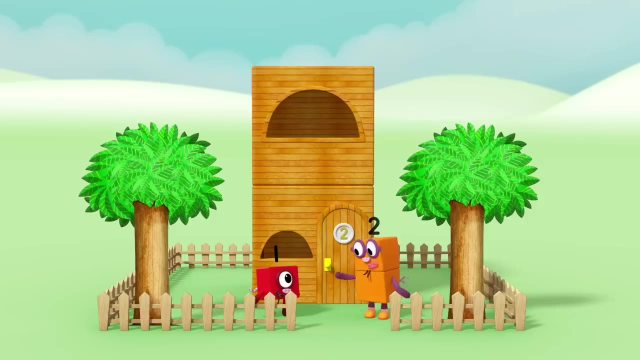 Luckily, the second little pig had a house with two rooms: Room for two, me and you. It has one two, two windows and one two two trees in the garden, And there's a number two on the door. 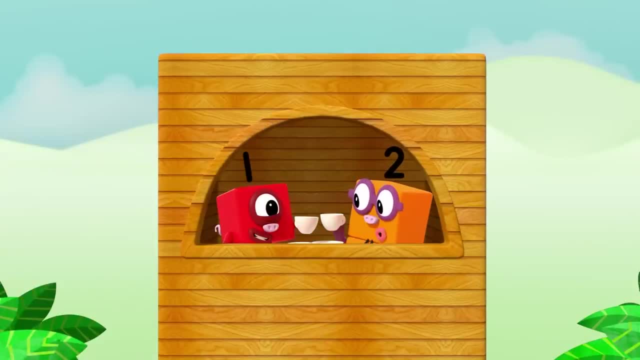 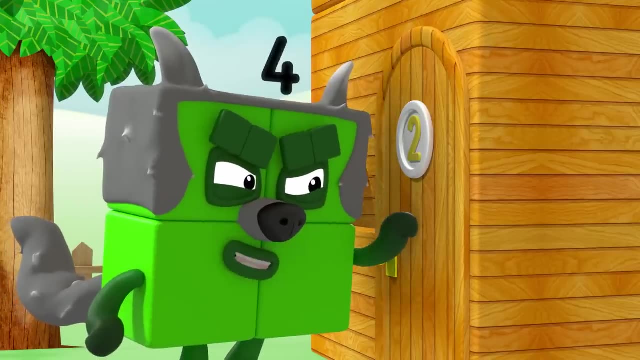 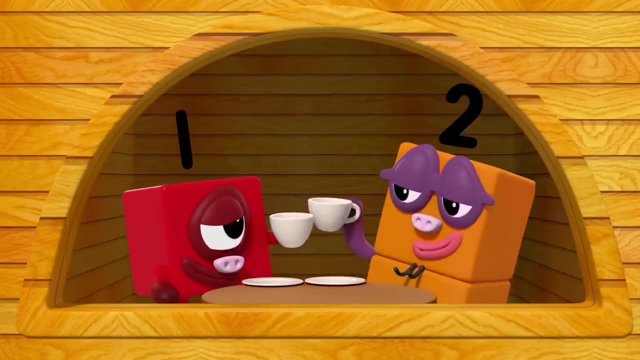 Tea for two and two for tea, Little pig. What are you doing here, little pig, Little pig, Little pig, Let me in. Let me in, Not by the two hairs on my chinny-chin, Then I'll hoof and I'll poof and I'll blow your house in. 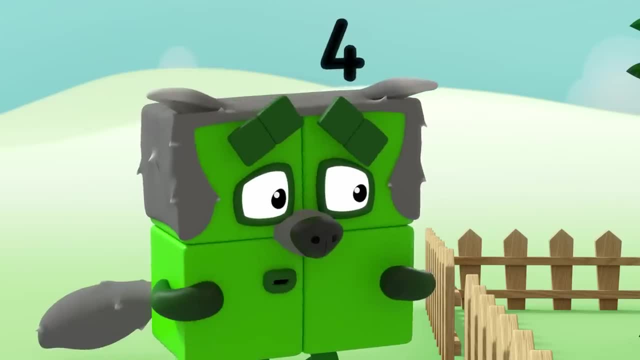 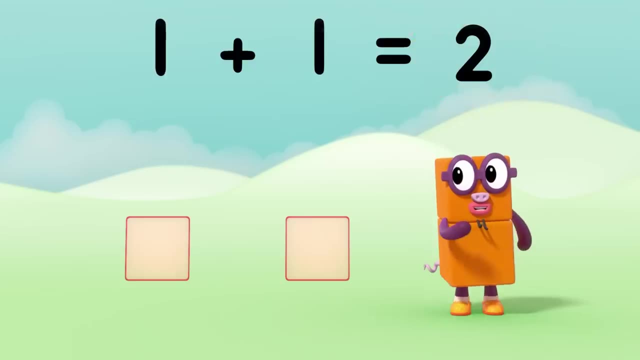 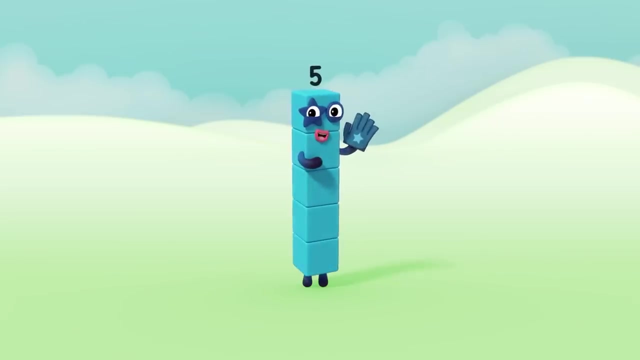 No, Oops, Sorry, two. One plus one equals Two. No worries, It's only pretend, But where will we live now? Luckily, the third little pig- Oh, that's me Busy, busy, busy- had a house with three rooms. 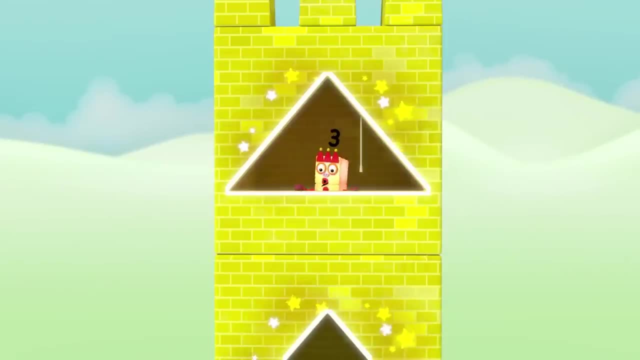 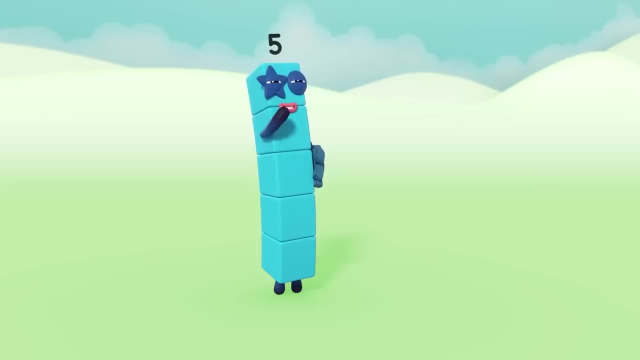 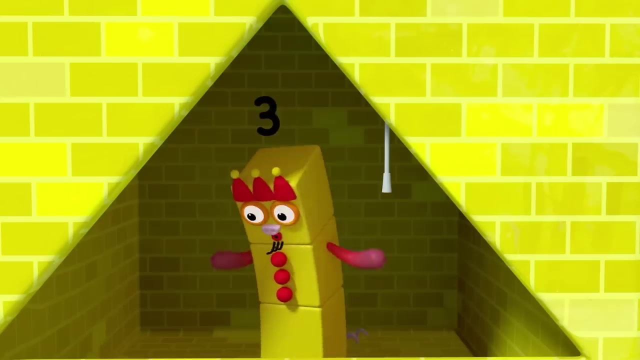 and one, two, three, three windows, and one, two, three, three turrets and one, two, three, three flags. and yes, yes, thank you, three. Room for a couple more Sure, Two's company and three's a party. 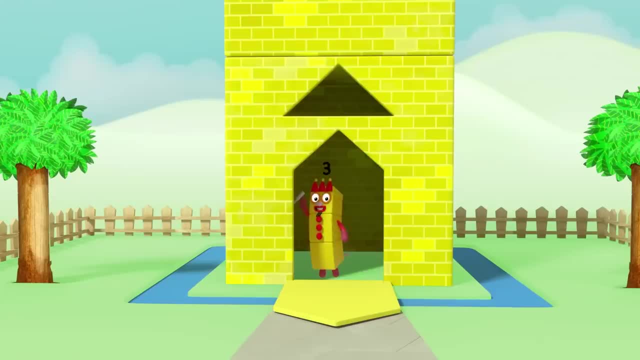 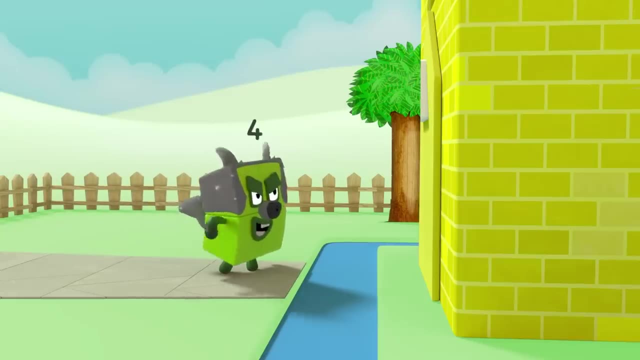 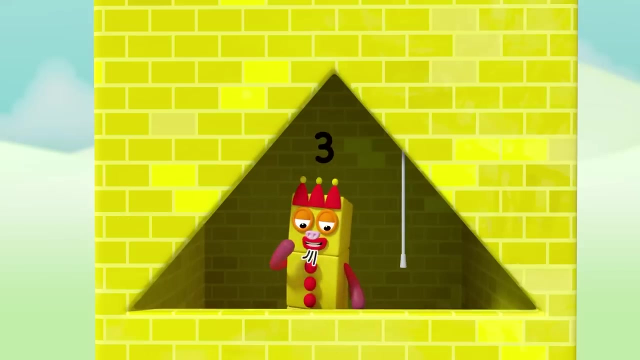 Keeping that big bad square out is as easy as one, two, three Little pig, little pig, let me in. Let me in, Not by the three hairs on my chinny-chin-chin, Then I'll hoof and I'll poof and I'll blow your house in. 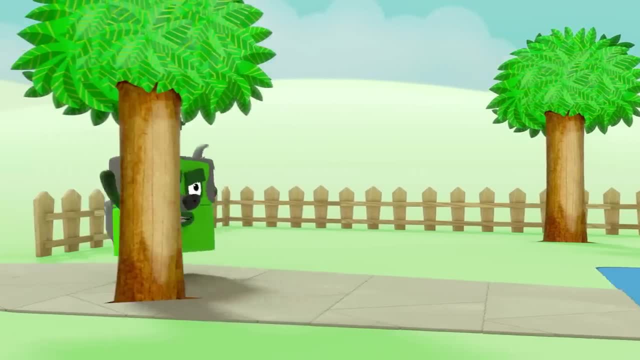 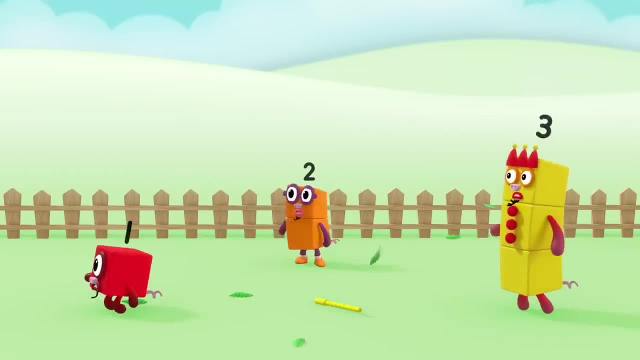 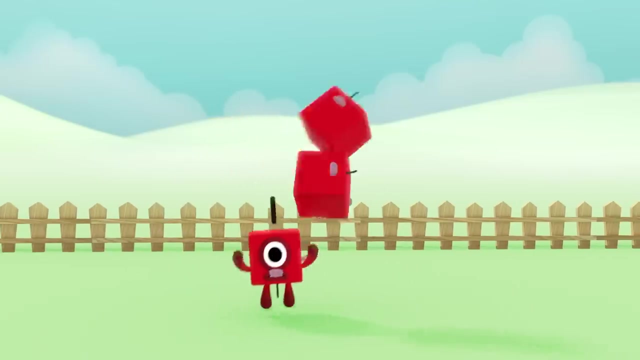 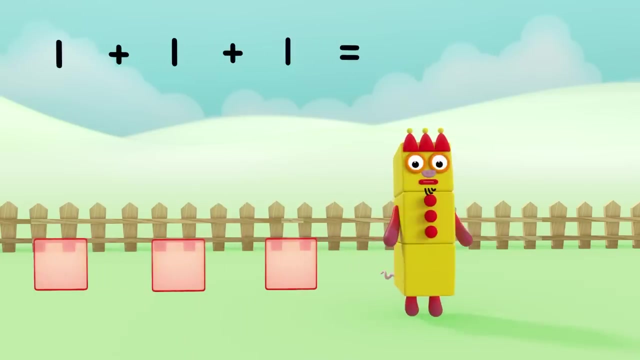 Then I'll hoof and I'll poof and I'll blow your house in What? But how? Just a little hoof, Hey, One plus one plus one equals three. See how you like it. See how you like it. 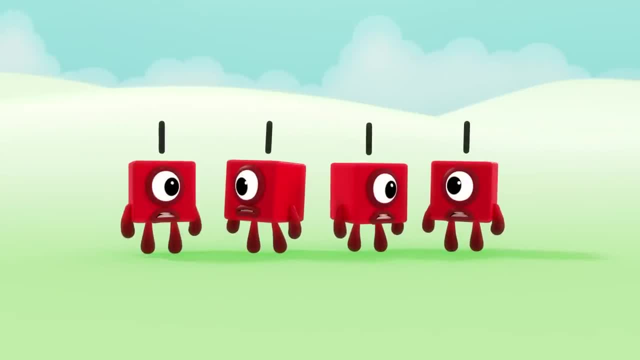 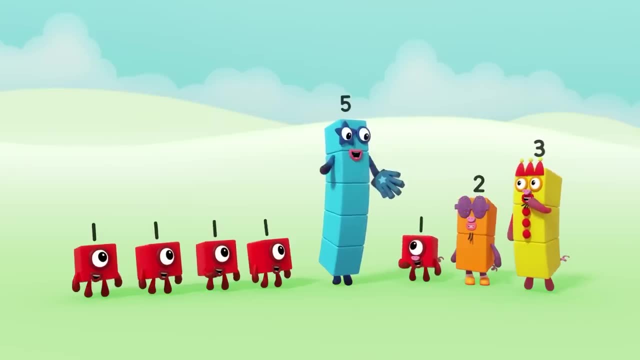 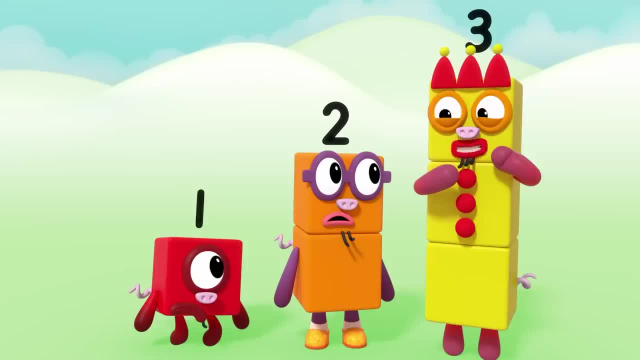 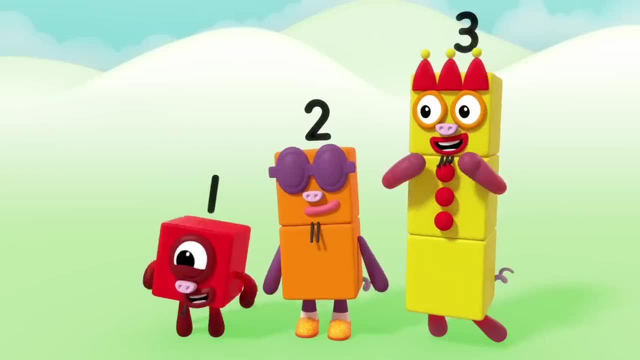 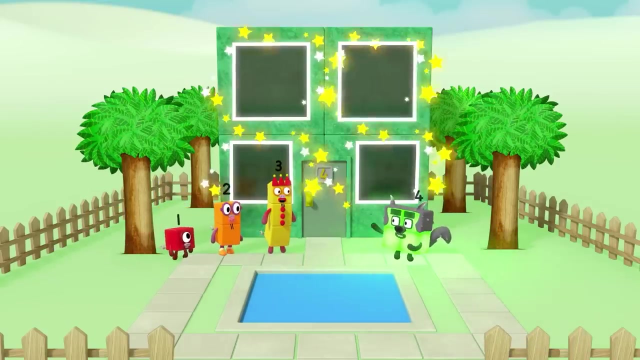 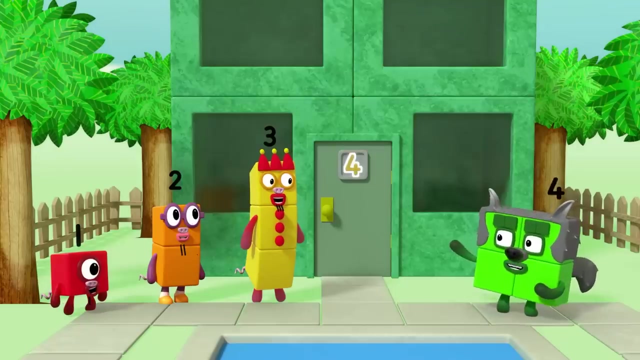 Four. Where will the three little pigs live? now? There's always my house. Oh, It's got four rooms with one, two, three, four, Four windows, and one, two, three, four, Four, threes and a number four on the door. 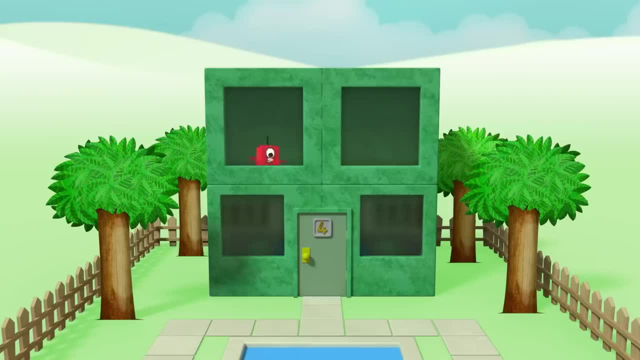 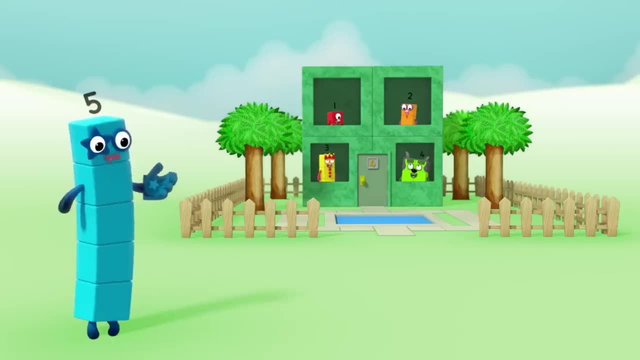 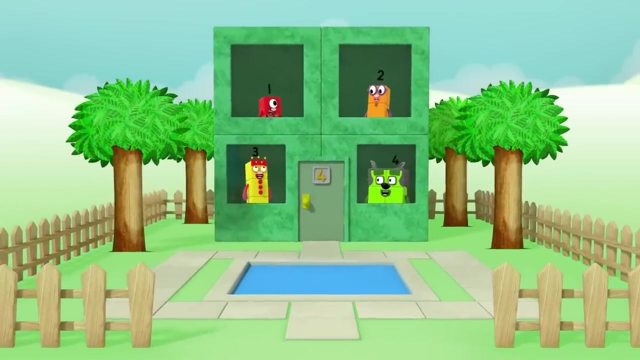 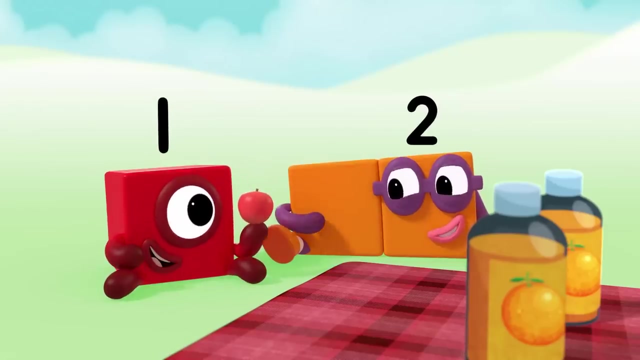 Woo-hoo- One, two, three, four. That deserves a big hand. Once upon a time there were three little pigs and a big bad square, and they all lived happily ever after The end. Yay, Mm. 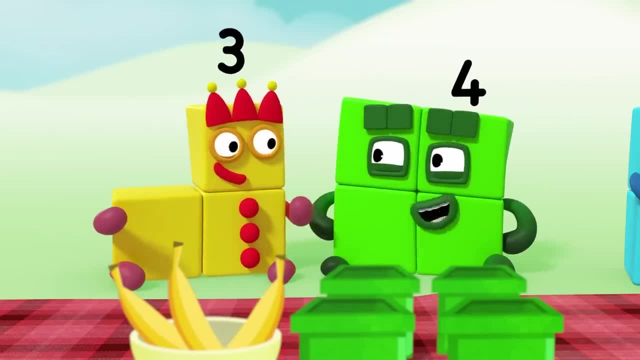 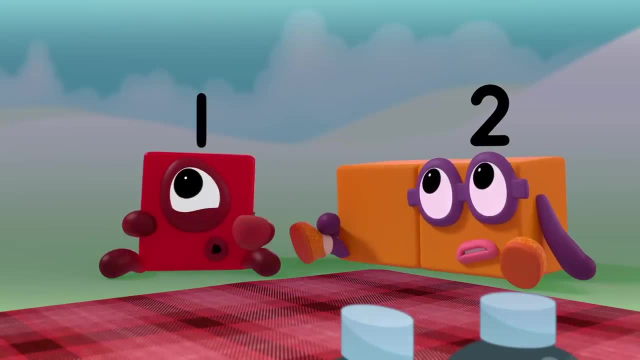 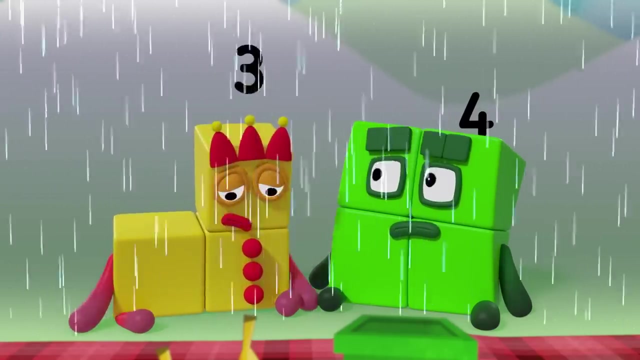 Nice picnic. I can't wait. It looks so yummy. That's a five-star picnic. Let's get stuck in, shall we? Oh, the sun's gone in. That's unlucky. Starting to rain? That's unlucky. That's raining a lot now. 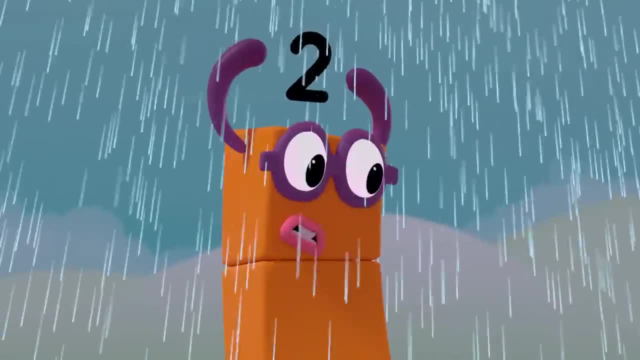 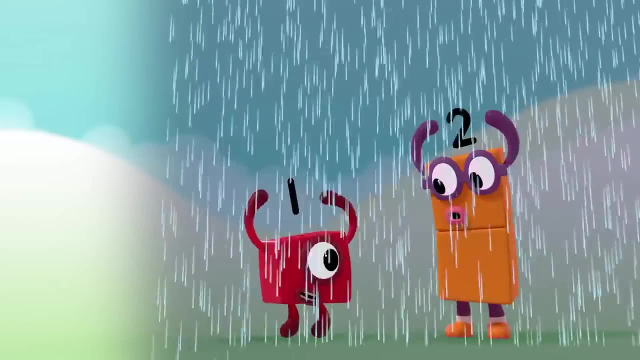 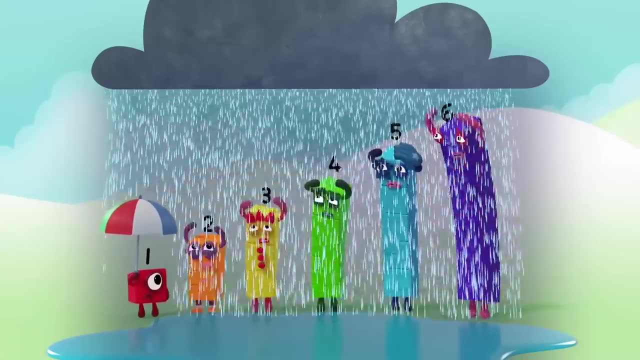 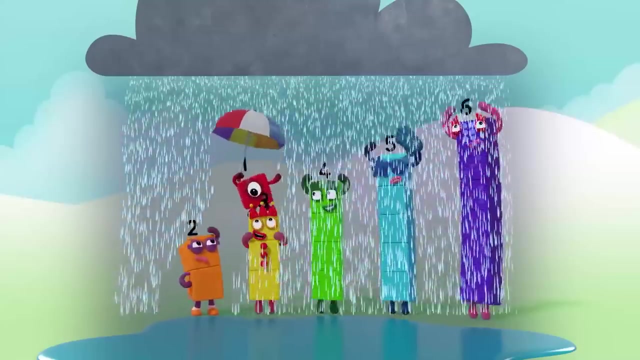 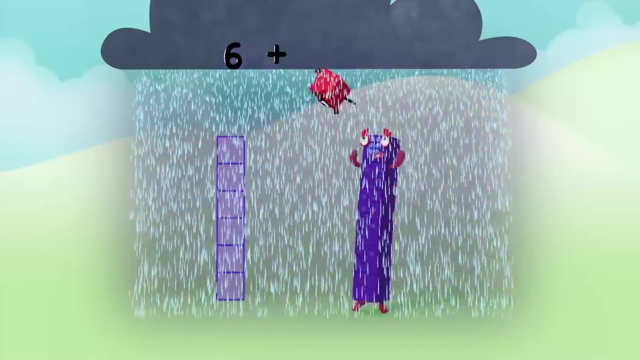 That's unlucky, That's all. Anyone got an umbrella? I ain't got one, Only one. That's unlucky. Hmm, I can share it. Huh, Ah, Huh, Oh, Oh Oh. Six plus one equals seven. 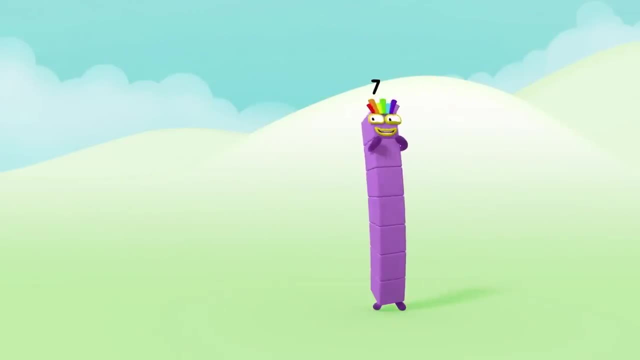 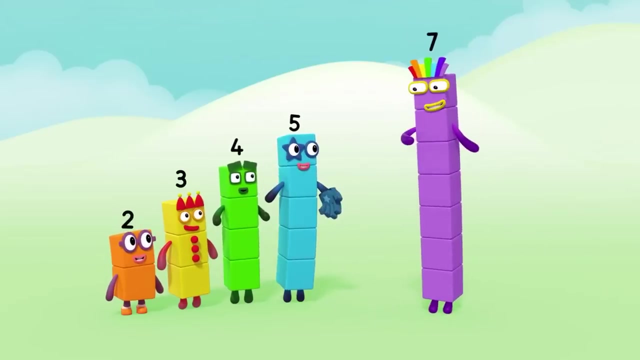 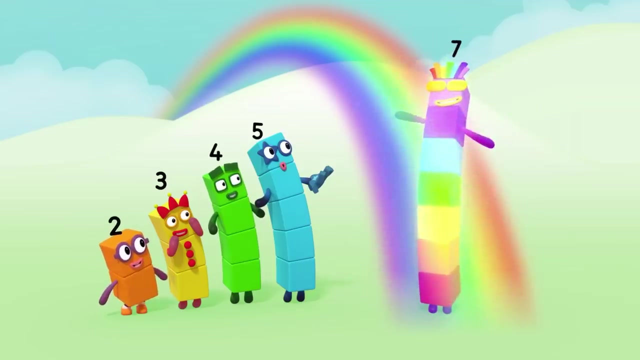 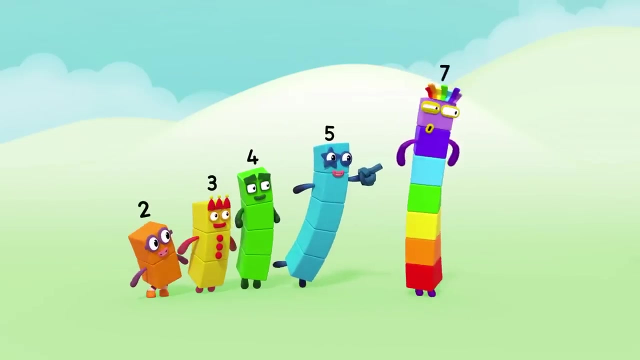 I am seven. Am I in heaven? You're in Numberland. Oh, lucky me. Ooh, A rainbow, Woo-hoo-hoo, Ooh, Wow, What, What happened? Look, Oh, A mirror, That's lucky. 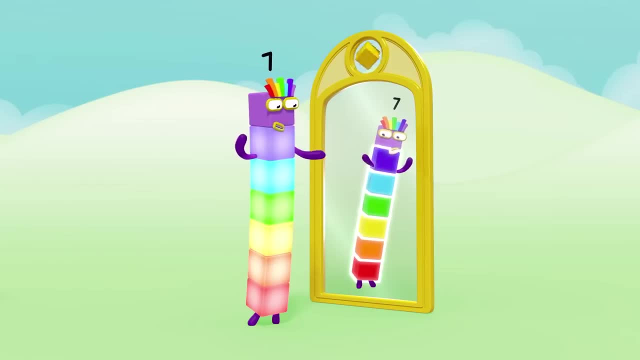 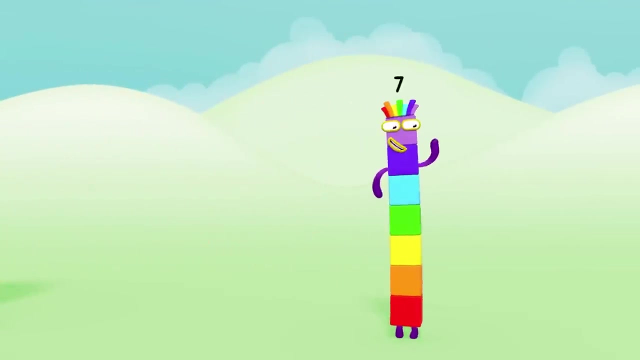 One, two, three, four, five, six, seven, Seven colours- I'm all the colours of the rainbow. Now, isn't that a stroke of luck? Luckily, I know just what to do now. Seven minus one equals six. 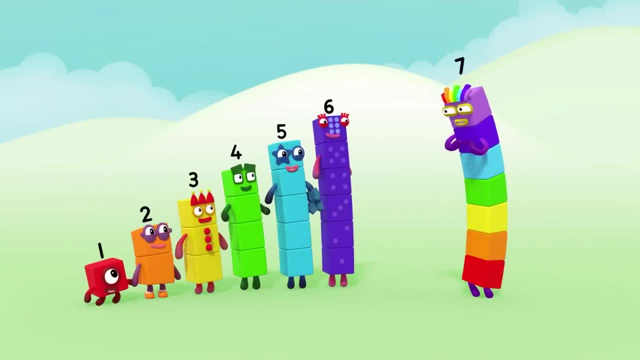 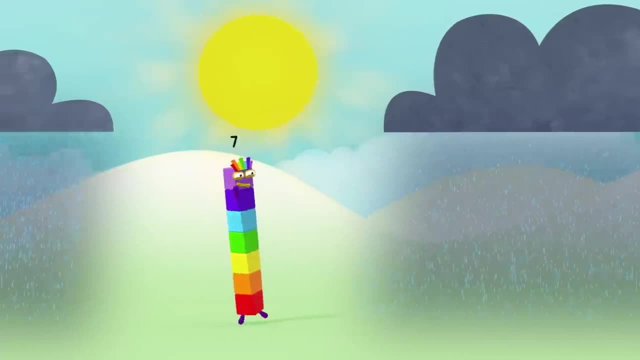 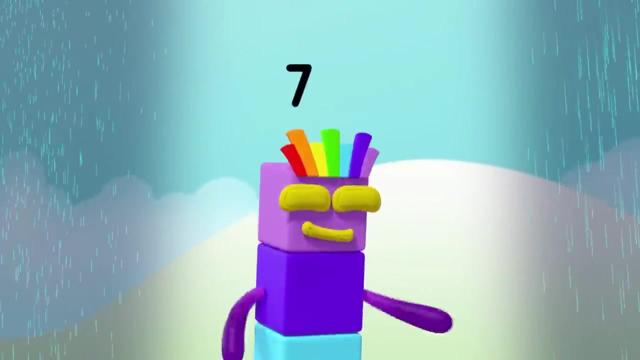 All you lovely blocks are my friends. Mm-hm, I'm the luckiest number block in the world. I'm lucky number seven, I'm in a happy place, The sun is always shining And there's always a smile upon my face. 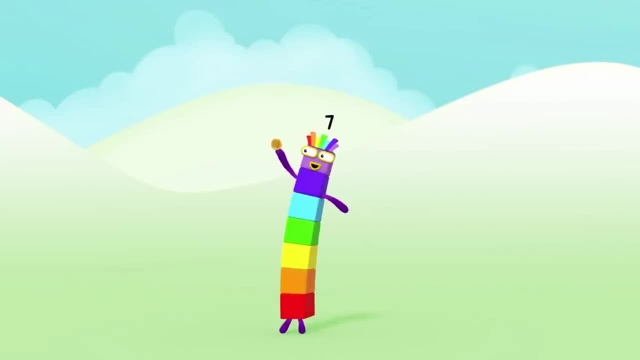 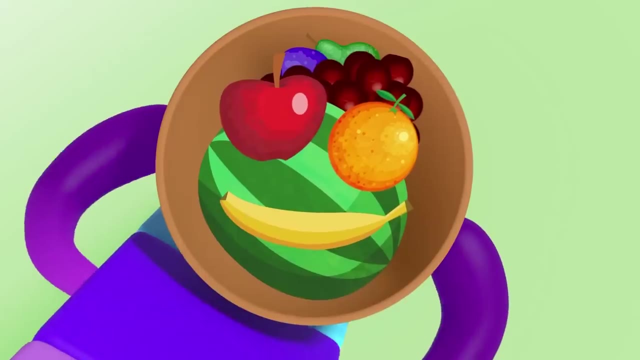 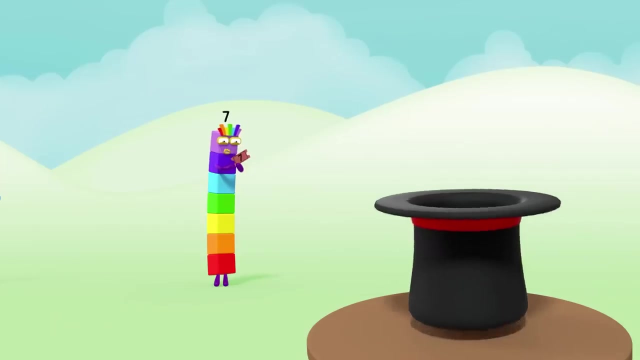 I see a penny in a picket up And all day long I have good luck. I'm lucky number seven And everything is falling into place. I'm lucky number seven And, as you might have guessed, I always win the raffle. 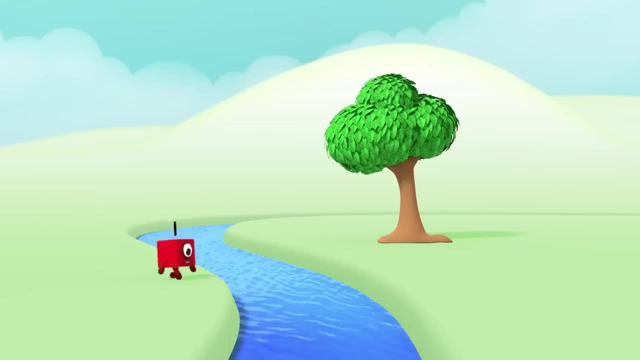 With seven on your side. you're seven blessed In a pickle. you're in luck. I'll help you out when you get stuck And if you stick with seven, everything will work out for the best. Yay, Rainbow time. 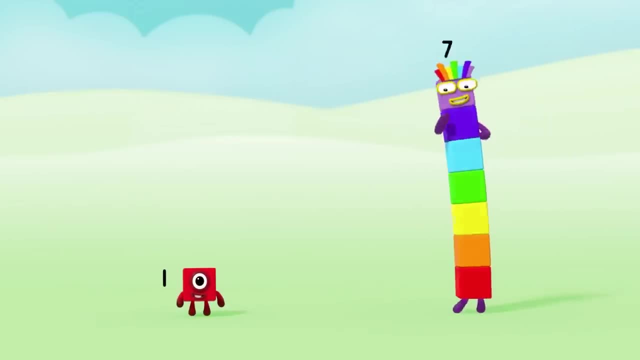 Red: My first block is the same as you. Orange, My second block is the same as two. Yellow, My third block is just like number three. Green: My fourth is green, as you can see. Blue for five, Indigo for six. 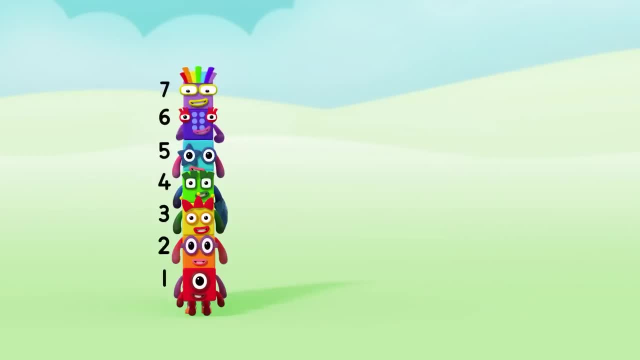 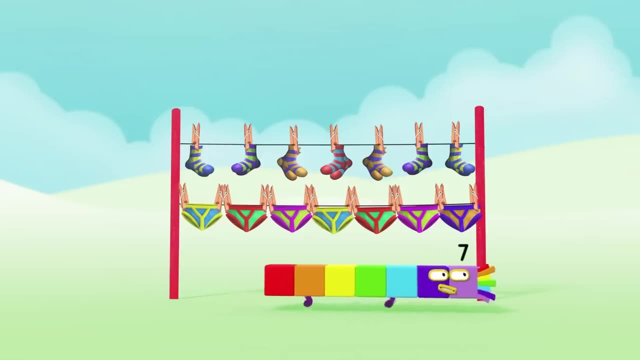 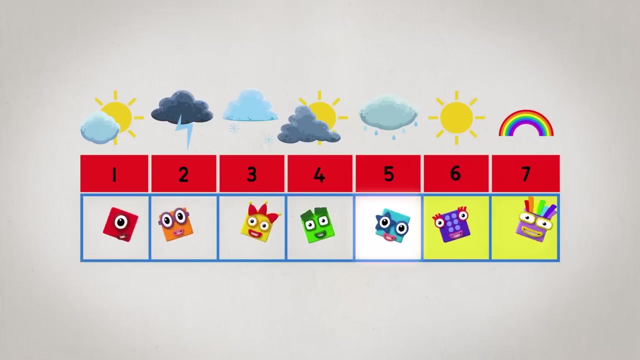 Violet is for seven. Oh, that's me. I've got seven rainbow-coloured blocks. that makes me unique. I've got seven pairs of pants and socks, one for each day of the week: Monday, Tuesday, Wednesday, Thursday, Friday, Saturday, Sunday. 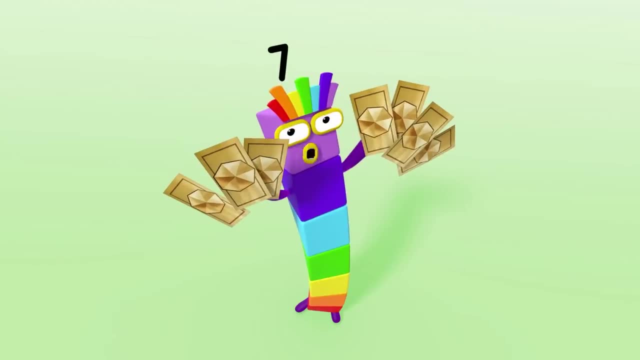 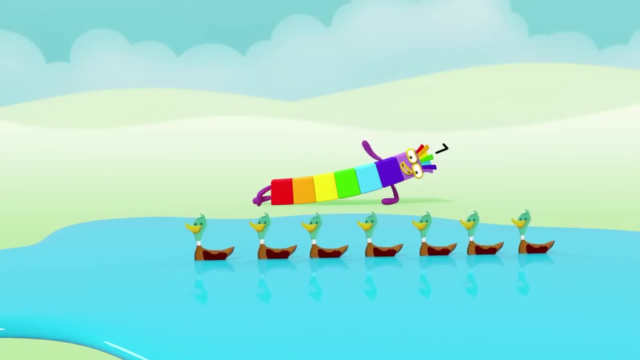 One, two, three, four, five, six, seven. I've got seven golden tickets: One, two, three, four, five, six, seven. All my ducks are in a row: One, two, three, four, five, six, seven. 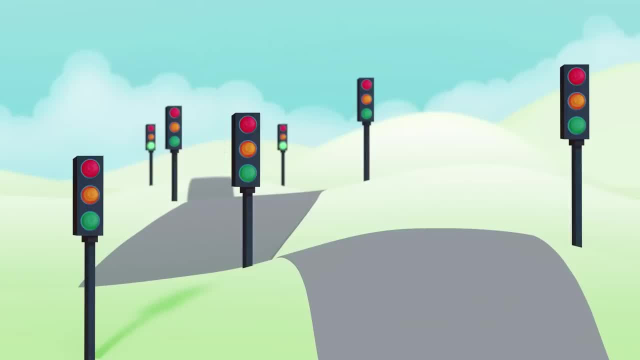 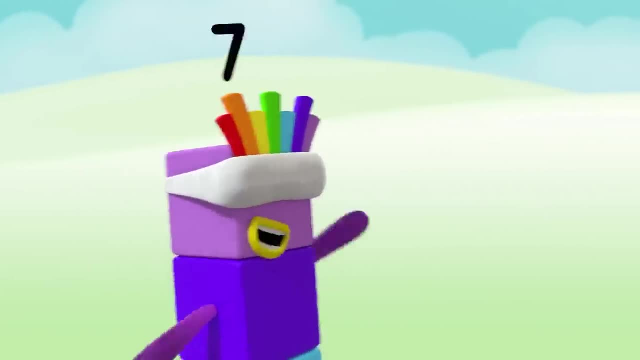 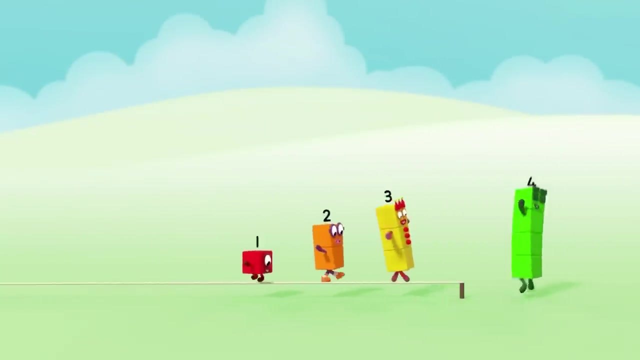 Nothing's going to stop me or my traffic lights, Orange go. I'm lucky number seven. I'd like to chance my arm In tricky situations. there's really no reason for alarm. I take problems in my strike. I've got fortune on my side. 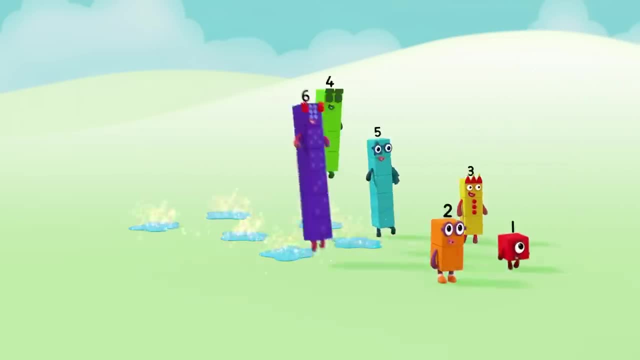 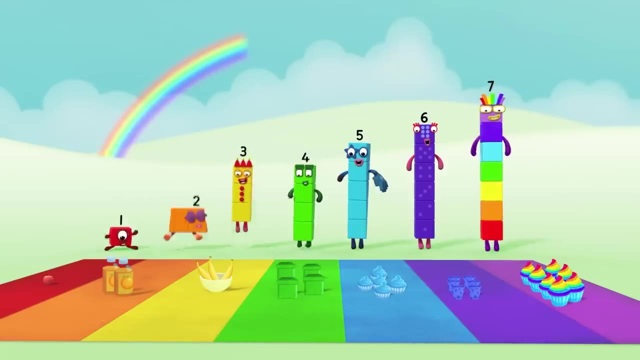 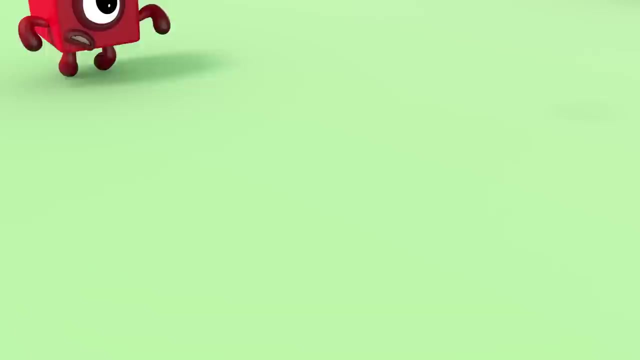 I'm lucky number seven. When you're with me I'll be your lucky charm. One, two, three, four, five, six, seven. So lucky number seven. I've got seven tickets: One, two, three, four, five, six, seven. 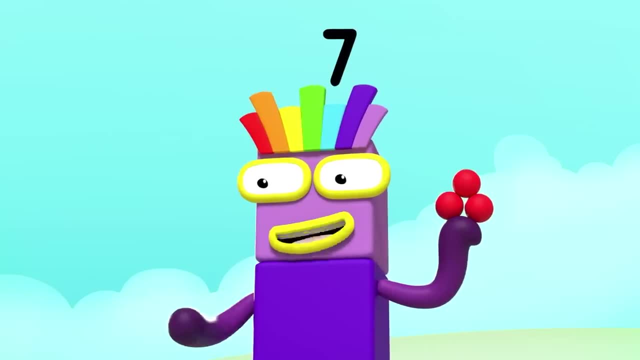 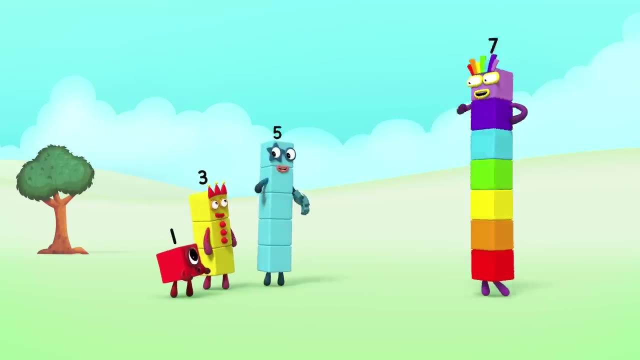 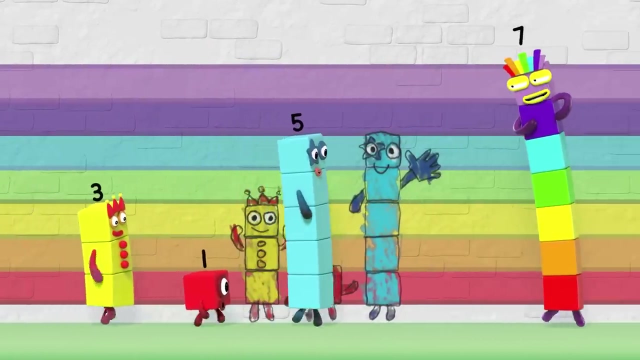 I got bombed. I've got happiness. I'm lucky number seven. One, two, three, four, five, six, seven. I've got fortune number seven. We all have our place, but we're different. That's very easy to see. 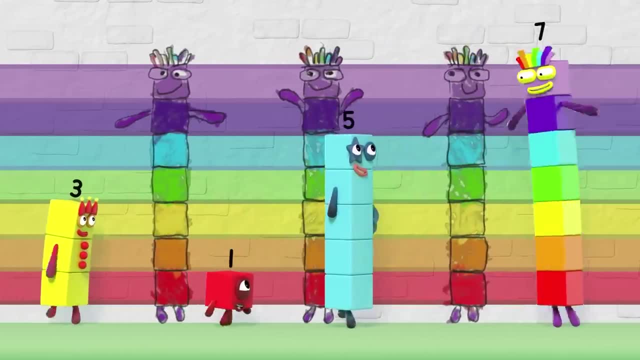 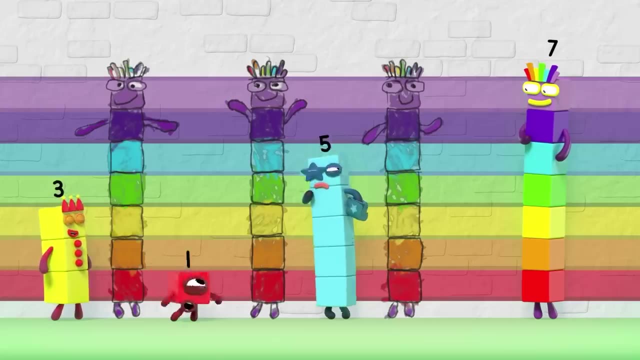 We're all friends here, but we're different. But what makes you you and not me? I'd love to be you, but I come up short. I need to add something. but what? I'd love to be lucky like Seven. 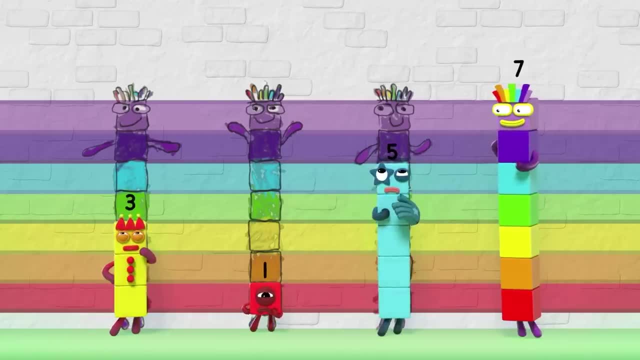 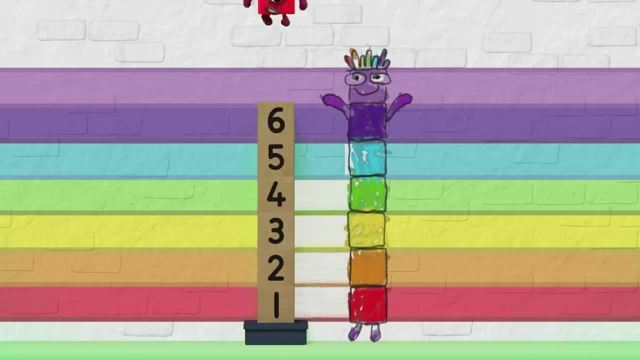 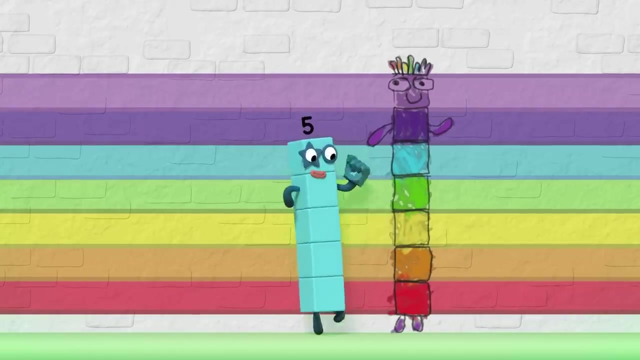 What have you got that we haven't got? I could try on a hat, That's the difference. Or I could stand on a box, That's the difference. And if the difference won't pop into your head, you can count the missing blocks. 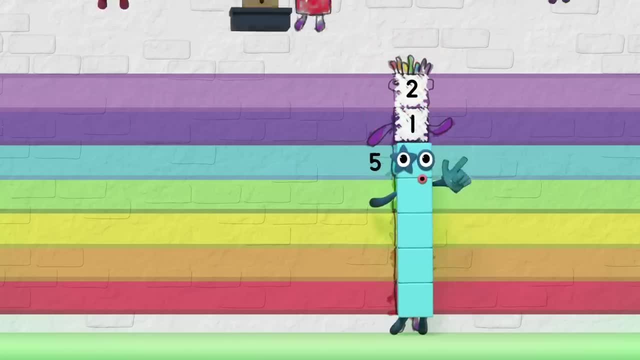 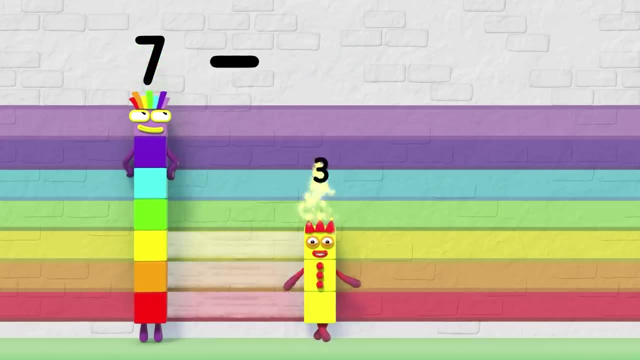 One, two, two. The difference is two. So what's the difference? Seven minus three equals four. That's the difference. Four, Seven minus me equals six. That's the difference. Six Seven minus five equals two. That's the difference. 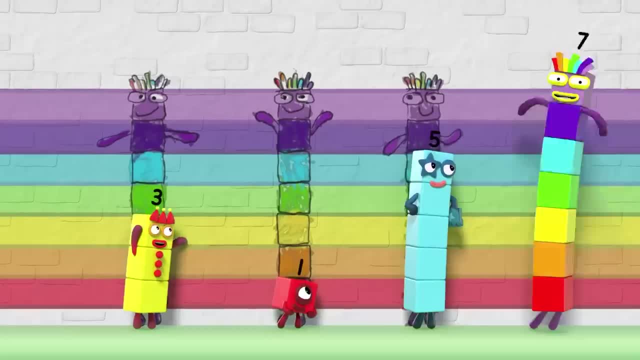 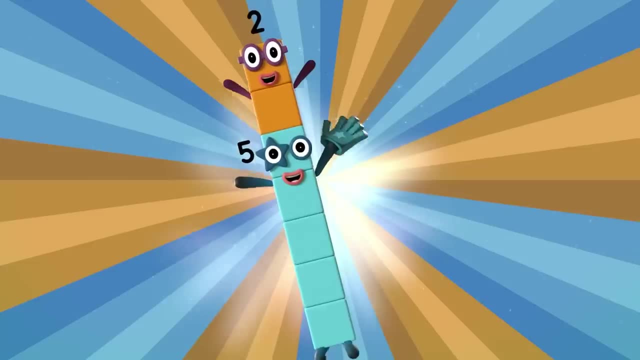 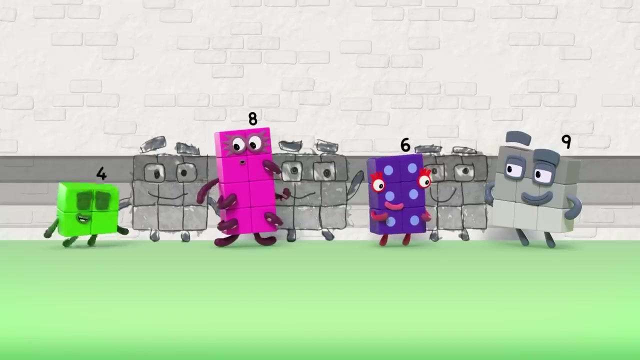 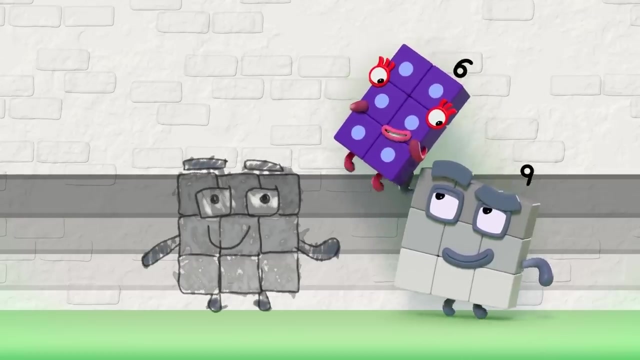 Six. So make up the difference and everyone will see what the difference is between you and me. I'd love to be you, but I come up short. I need to add something, but what I'd love- to be stronger like mine- is. 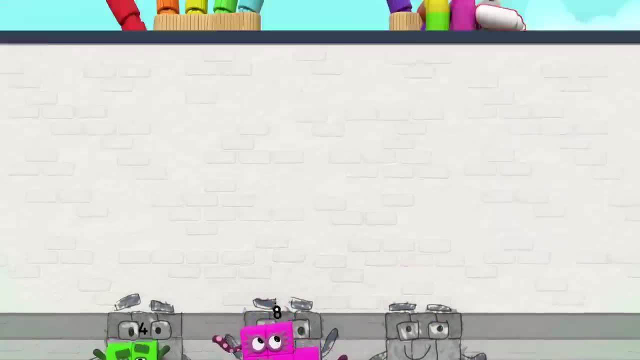 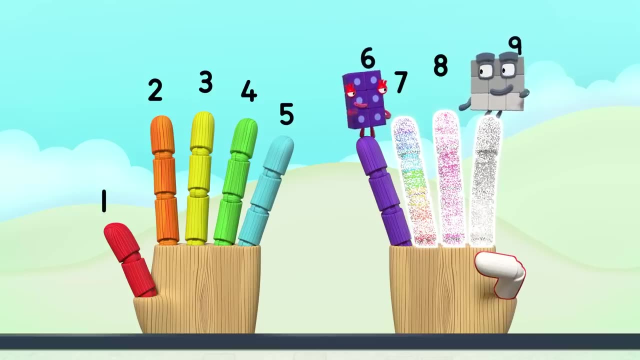 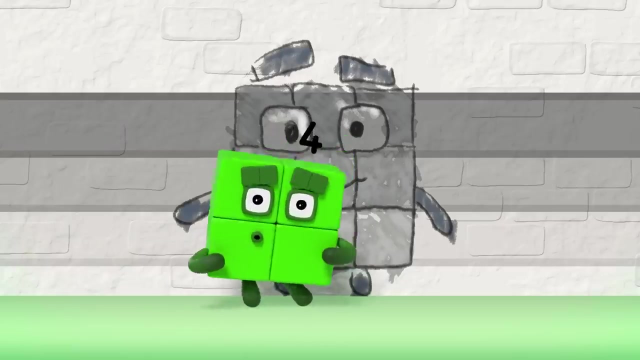 What have you got that we haven't got? You can count on your hands. Seven, eight, nine, That's the difference. Three. One, two, three. You can fill in the space. That's the difference One. And if the difference won't pop into your head, 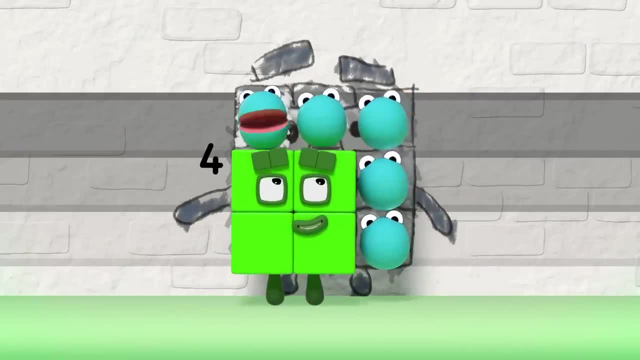 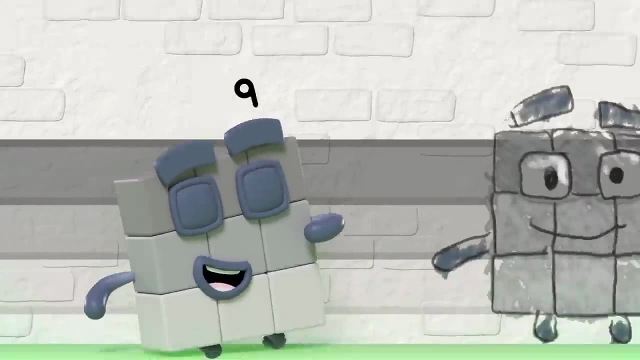 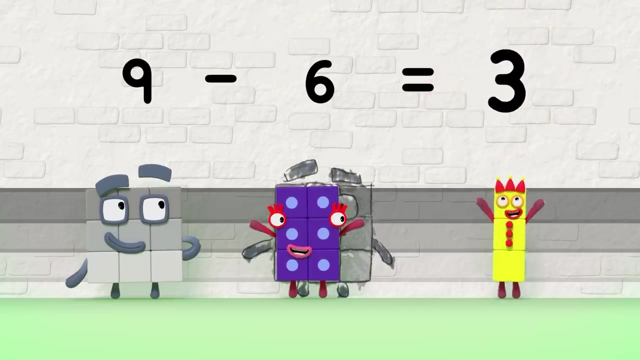 you can count number blocks in place: One, two, three, four, five, Five. The difference is five, Five, Five. So what's the difference? Nine minus six equals three. That's the difference. Three Nine minus me equals one. 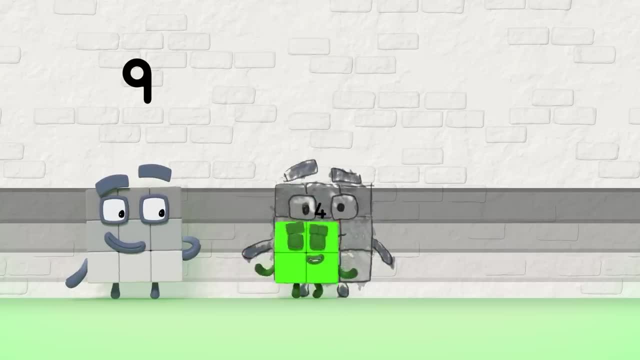 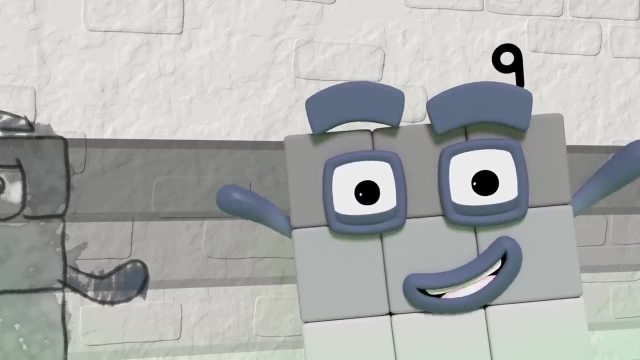 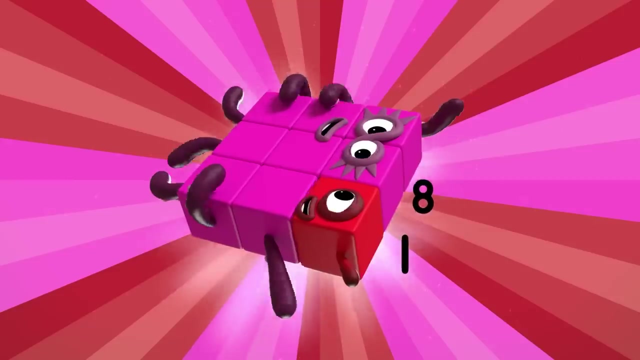 That's the difference One. Nine minus four equals five. That's the difference Five. So make up the difference and everyone will see what the difference is between you and me. Every time you are wrong, you getWithout einzigoooooo. 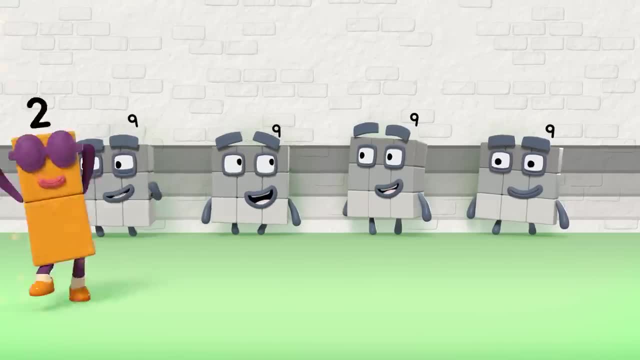 Every time you are rightinapproper And it's not fairthat you don't get zoomed in on fun 0. I see, But if you get buzzedealthdiggghzzz, you get buzzedealed. 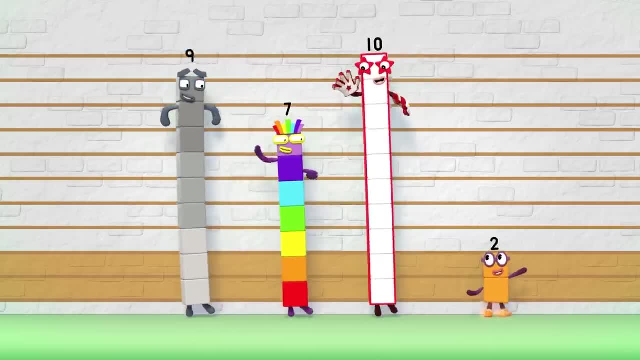 Remember, you are impossible. Actually three, You don't get buzzed. I like that. It's a whole purchase, So we're going to evaluate it to me And if you think I'm still doing what I do, it's too cheesey and farce.